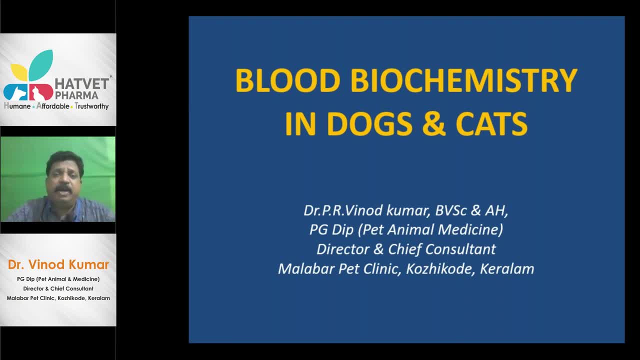 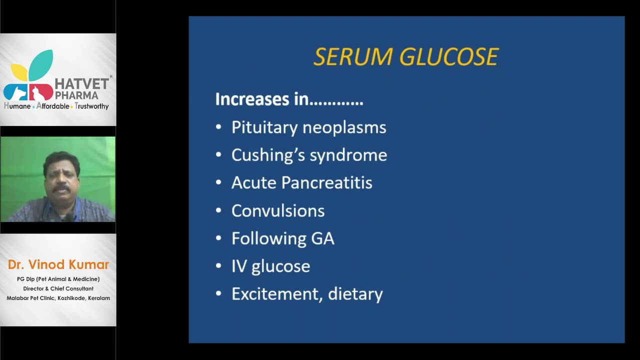 Detailed studies, And blood biochemistry deals with the solids in the plasma. So first of all we are going to deal with how or what is the plasma and what the serum is. Plasma we all know, because in the fluid therapy class itself, 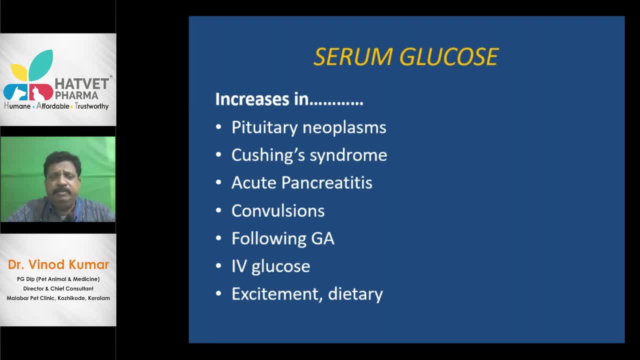 we have discussed regarding plasma. It is nothing but the fluid portion of the blood which contains all the elements of the fluid, including the blood cells. Some are seen as visible elements in the blood, For example the blood cells. Some are seen as invisible elements in the plasma. 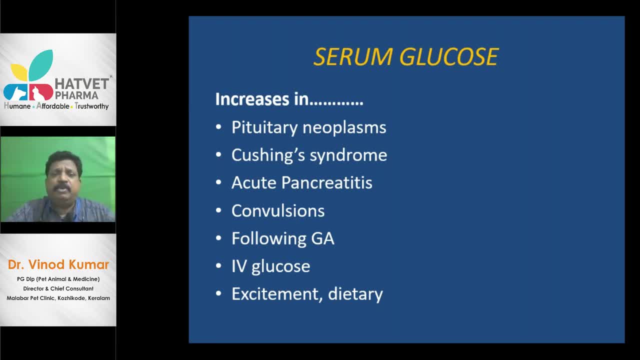 Those are the electrolytes and other dissolved substances. All these are chemical substances. So, whereas in the other part, the blood cells, it was not a chemical subject, It was only a biological part of the blood. And now today, we are going to deal with the dissolved chemicals of the blood. 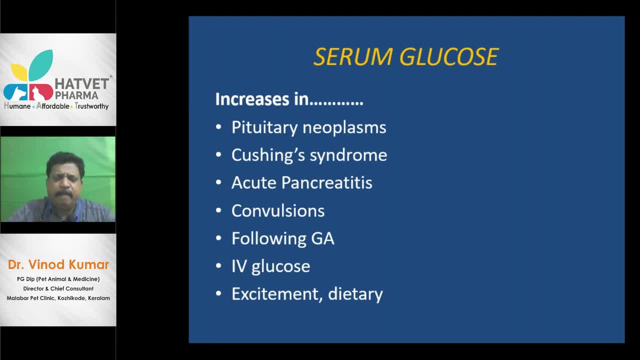 Let us deal with not all, Because if we are going to deal with all the chemicals, it will be very difficult. Of course, it takes a day together, So we are going to. So we are going to discuss the most commonly analyzed plasma elements. 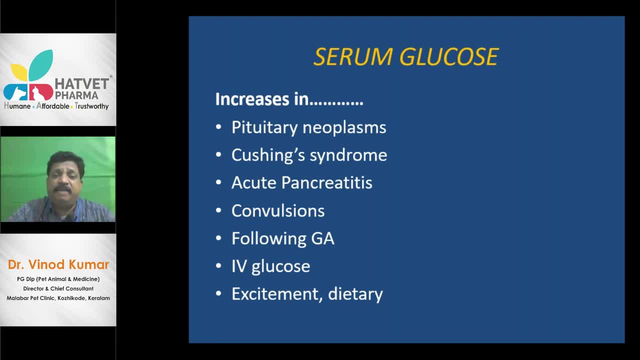 So when the blood is taken- yesterday we studied about how the blood is taken and how the blood is allowed to clot, or how the blood is not allowed to clot. See, the blood can be kept aside for it to be allowed to clot. 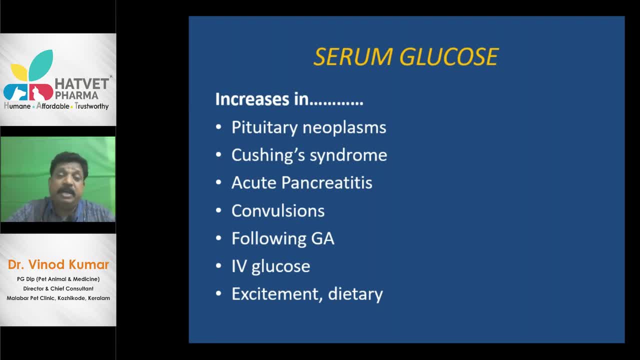 Good, Thereby we are going to collect the serum. Sometimes, even with an anticoagulant, the blood will not clot. See, if it is with an anticoagulant, it will not clot. Sometimes, if there is no anticoagulant, also, it will not clot. 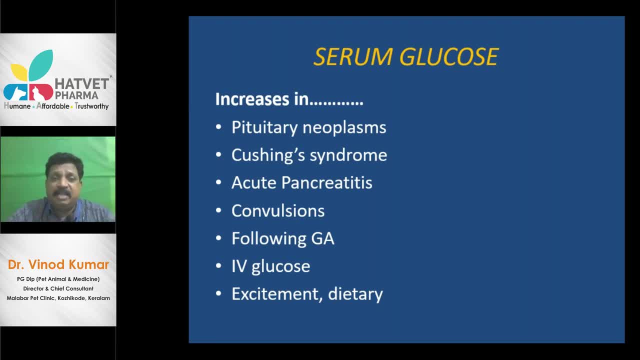 We know certain conditions, and the most important such condition is a snake bite. We know the protocol of a snake bite. In a snake bite suspected case, the first thing that we, the veterinarian, can do is so simple: Take some blood, Keep it aside for 20 minutes in a simple vial which doesn't contain any anticoagulant. 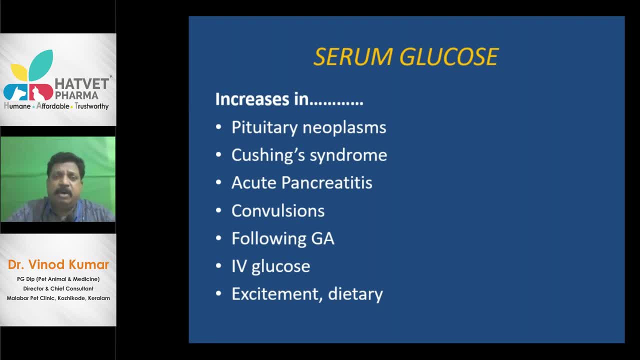 Yesterday we studied about the Heller and Paltz double oxalate anticoagulant, the heparin, the sodium citrate, the EDTA. So all these things anticoagulants we studied And we found that the commonest used is EDTA. 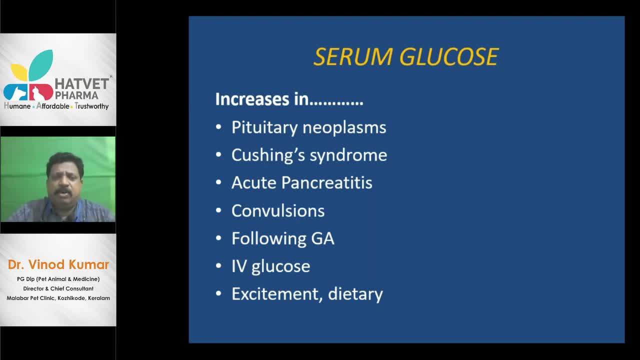 Suppose you are presented with the case of a labrador which is suspected to be bitten by a snake. Let it be a hemotoxic snake or a neurotoxic snake, It has been bitten. What will be the first test you are doing? 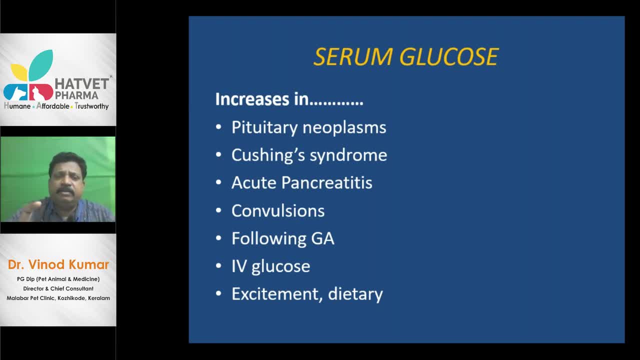 So simple. You take a blood collection vial which is not anticoagulated- Nothing is added to it- Take the blood in it, Keep it aside for 20 minutes And if it is clotting, it means that it is not a snake bite. 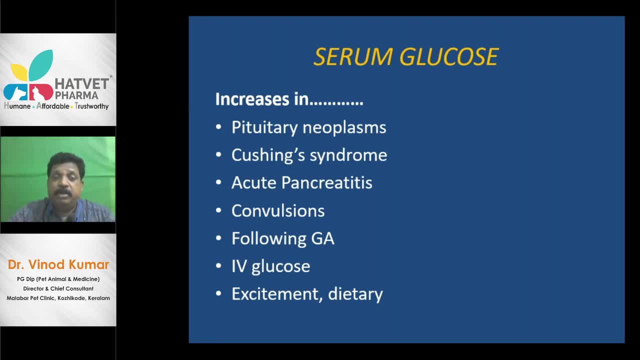 If it is not clotting during these 20 minutes. it has no tendency to clot. After that. make it upright, twist it so that it has not clotted means it could be a snake bite. At the same time, it is showing all the signs of a snake bite. 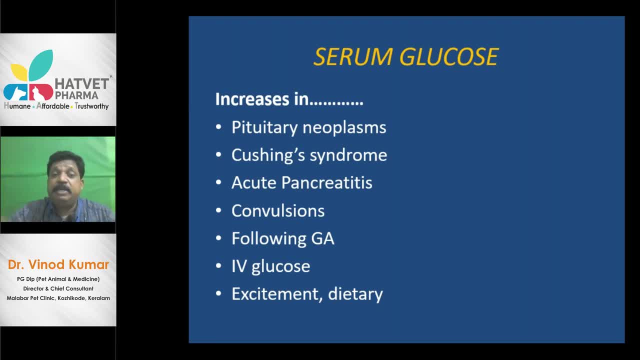 But at the same time, on this 20 minutes clotting test, it is positive. So that is the blood clotting And at the same time, after clotting of blood, we can see that all the cells will be clumping together or agglutinating to form a clot. 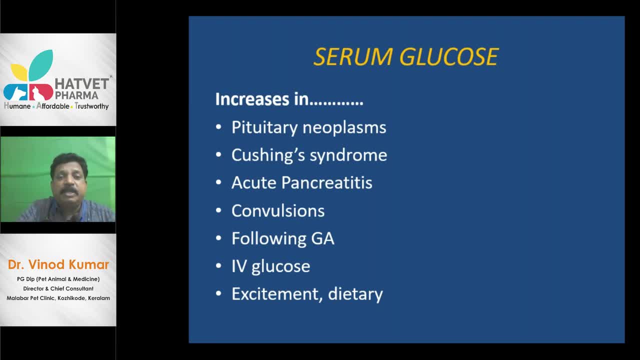 So the blood clot will be formed, It will be separated And the remaining portion you can see as a clear, light yellow fluid And this we call as a serum. That is how the serum is separated And the serum can be slowly poured off into another vial. 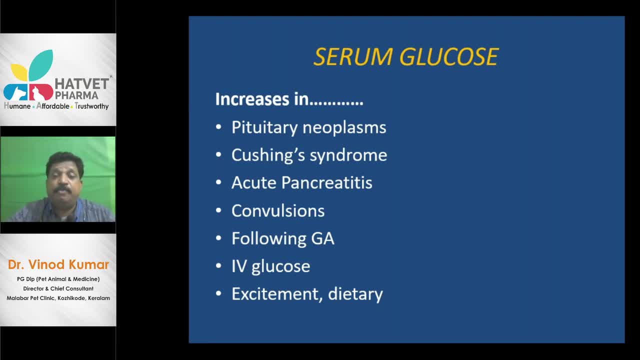 And this serum is mainly used for our estimation of almost all the elements of blood- chemical elements. This serum is used When you are giving the blood to an outside laboratory. either you can give the clotted blood as such Or, if you are equipped enough or you have enough time, to separate the serum and the clot. 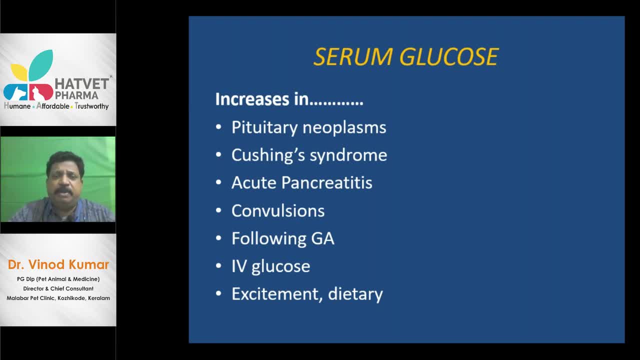 so that it can be centrifuged at 5000 rpm for 3 to 5 minutes. Then you can take it out. You see that the decanted clot and the supernatant will be the serum, So that the serum can be separated or it can be aspirated. 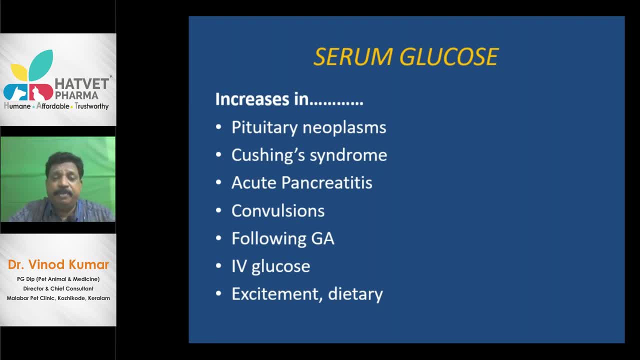 And then it can be given for analysis Or, as what I am doing, give the blood directly to the laboratory. They will collect the serum and do the test. So many things are there to be tested in the blood. Those are the salts in blood or the chemicals in the blood. 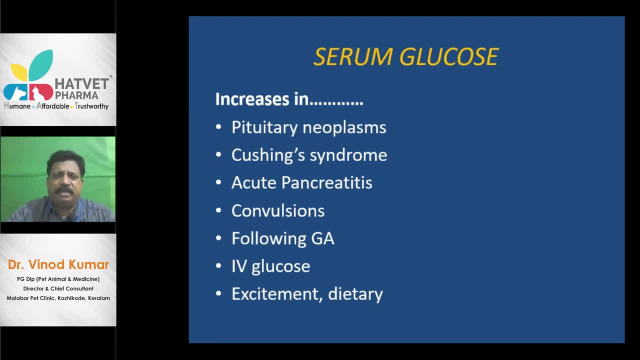 It each has its own significance, For example, the glucose in the blood. Of course, we all know that there is glucose in the blood of every individual, Whether it is a mammal or a reptile or an avian, whatever it be. 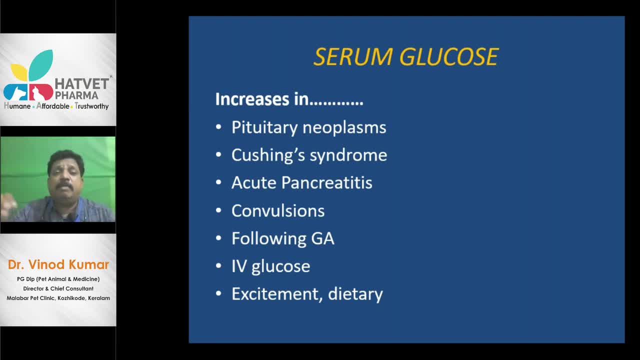 In avians we all know the BGL normal blood glucose level is typically high Because they are intended to fly, So it has high glucose normally. And within the mammals we can see the ruminants Our cow got normally they have a blood glucose of approximately 50 mg per deciliter. 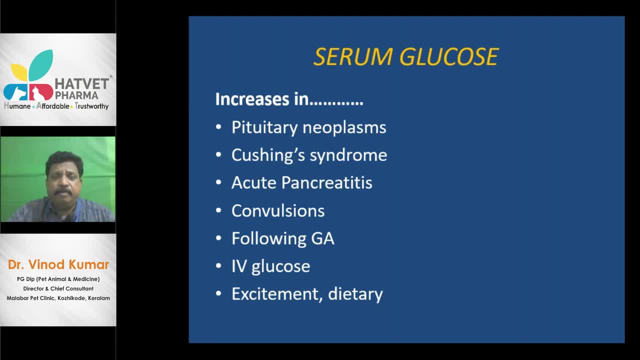 Normally it will be like that, But in the human beings- the dogs, the cats, etc. They have almost the same blood glucose level, That is, 80 to 120 mg per deciliter. Sometimes, in certain conditions, the blood glucose level increases. 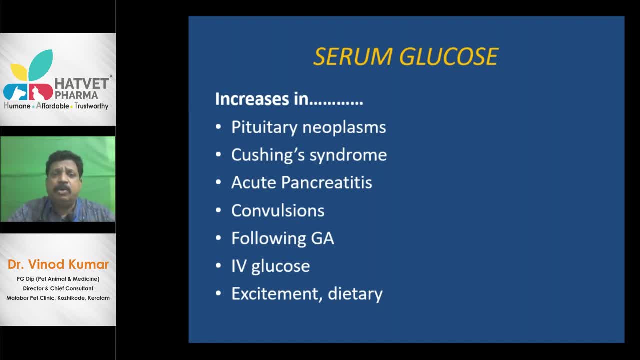 Sometimes, in certain conditions, the blood glucose level increases. Sometimes, in certain conditions, the blood glucose level increases. So we have to quantitatively analyze how much the blood glucose is. With that we can determine what the condition of the diseased animal is. 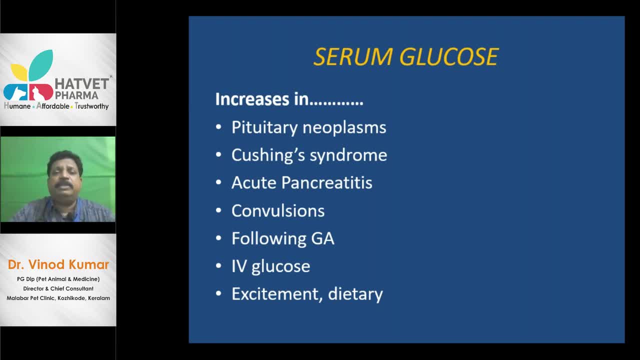 So the blood glucose can increase or decrease. Increase in blood glucose is known as The blood glucose is known as hyperglycemia, And decrease in blood is known as hypoglycemia. If it is normal glucose, it is euglycemic animal. 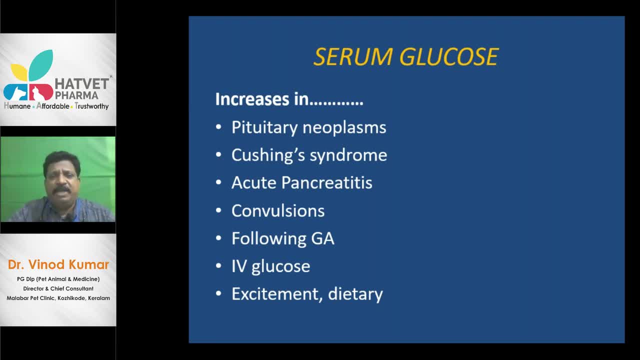 So let us see which are the conditions where the blood glucose increases, That is, Hyperglycemia occurs. So here let us see Hyperglycemia occurs Number one, In pituitary neoplasms. Why there is hyperglycemia in pituitary neoplasms? 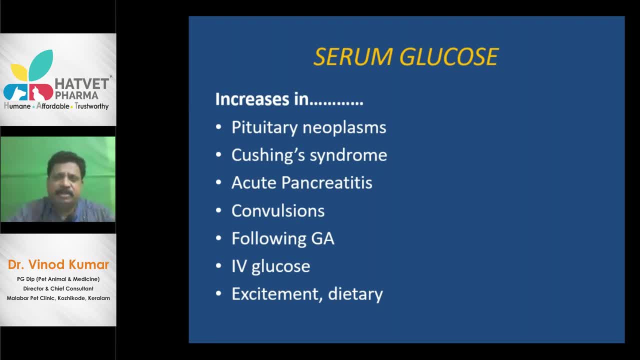 In pituitary neoplasms. We all know ACTH, ACTH- adenocorticotropic hormone. It is being released from the anterior pituitary And when there is a neoplastic pituitary, It is not common in animals or humans. 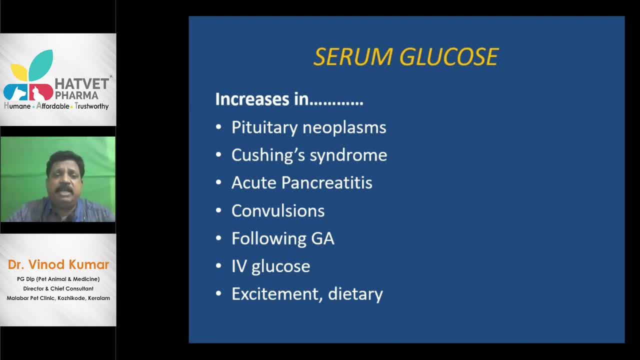 And it is not so easy to diagnose. also, We can simply study And we can simply suspect. if there is a sustained hyperglycemia in an animal, You rule out all other causes And for the last, as a last resort, you can suspect. 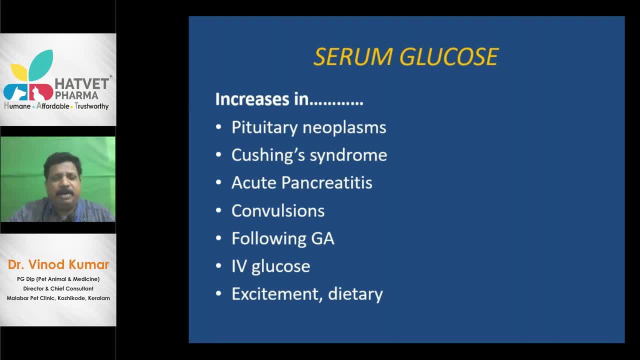 It could be a pituitary neoplasm. But unfortunately, if you find a pituitary neoplasm, What we can do Can we do a pituitary adenectomy. We cannot do anything. We can just go through the theoretical part. 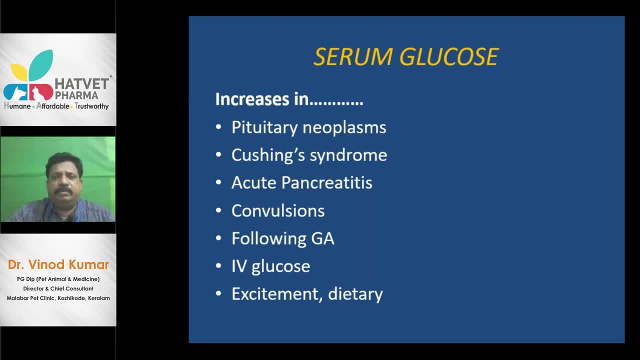 That is all. So. in pituitary neoplasms, As I said, There will be increased release of adenocorticotropic hormones. Some time earlier, We studied about Cushing syndrome In dermatology class. Most of you were there in the dermatology class. 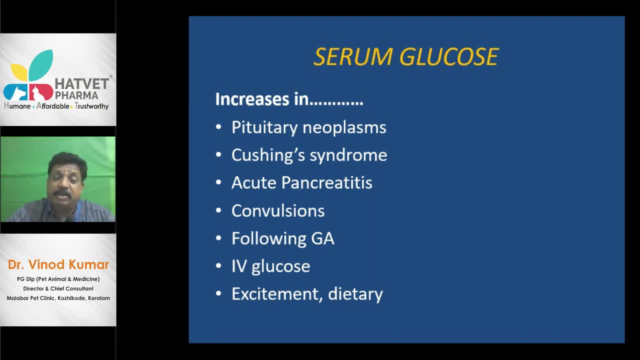 And there we studied or there we discussed How there is hyperglycemia in Cushing syndrome. And in that class I told Cushing syndrome are of two types: PDH and ADH. PDH means Pituitary dependent hyperadenocorticism. 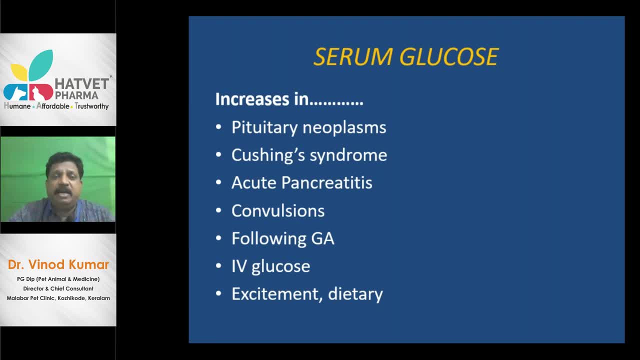 PDH means Adrenal dependent hyperadenocorticism, And I told that Pituitary dependent hyperadenocorticism Is seen in 85% of the cases of Cushing syndrome. So So In If it is pituitary dependent hyperadenocorticism. 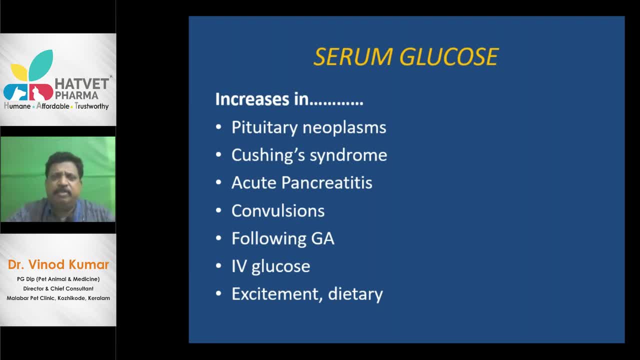 The ACTH. The high levels of ACTH Will stimulate The adrenal cortex. The adrenal has a cortex and a medulla. Adrenal cortex itself has A zone Of cells Which has a layer known as The zone of vasiculator. 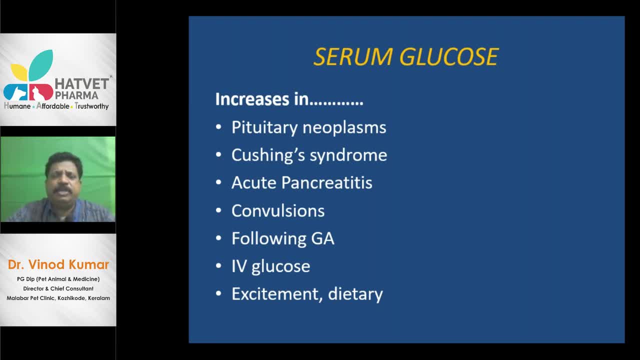 It has Typical Cortisol producing cells. Those cells will be stimulated. That means the adrenal cortex Is an adrenocorticotropic hormone. It will stimulate the adrenal cortex To release the Corticosteroids, Glucocorticoids. 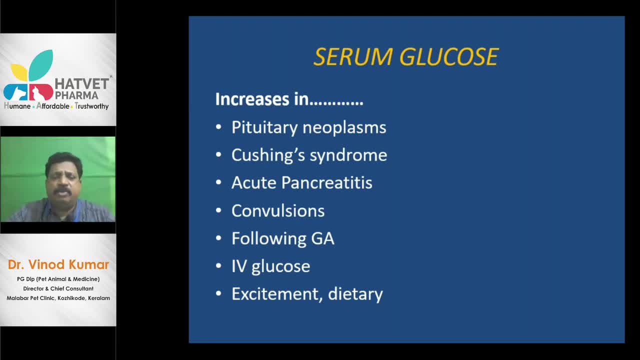 So that Glucocorticoids in large quantities will be released And These glucocorticoids Will convert Other nutrients To glucose. It is known as Gluconeogenesis. So when there is a gluconeogenesis, 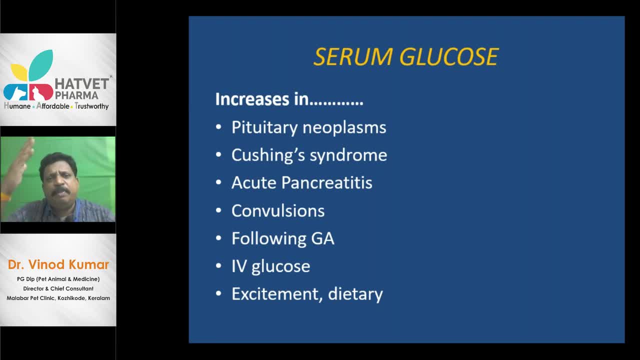 Quite natural, Blood glucose level will shoot up. Hyperglycemia occurs. The same thing happens in Pituitary neoplasm. There will be tremendous release of ACTH Ultimately, Which ends in hyperglycemia. So that is one reason. 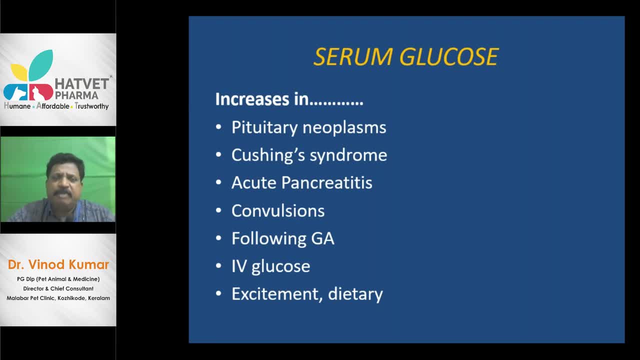 Number two is Cushing syndrome. Yes, We have discussed Cushing syndrome, How it occurs, Whether it is Pituitary dependent Or Adrenal dependent. See If there is a, If there is a primary tumor. 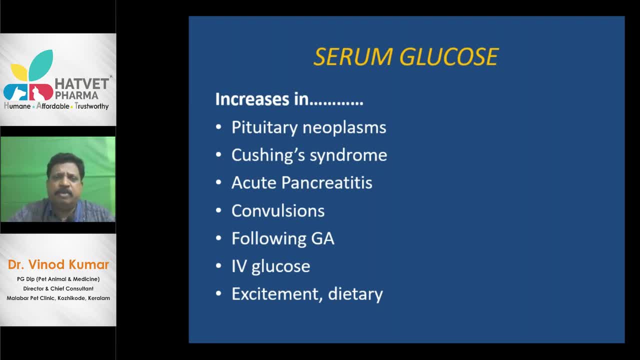 Of the adrenal cortex, For example In pheochromocytoma It is a primary Neoplastic condition Of the Adrenaline See. This generally happens When, When, When, When, When, When. 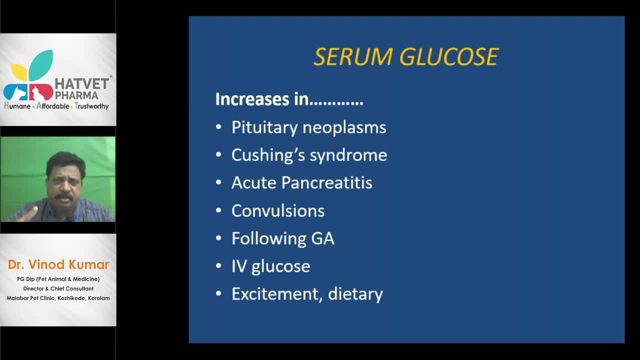 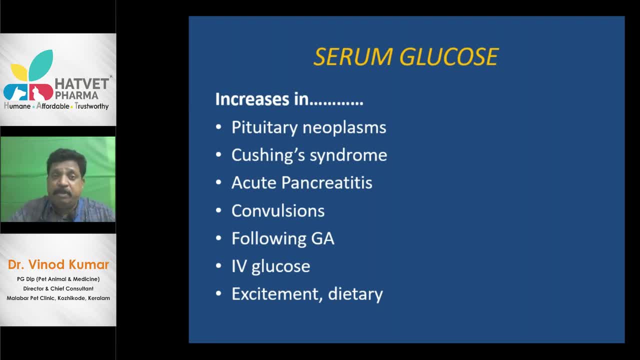 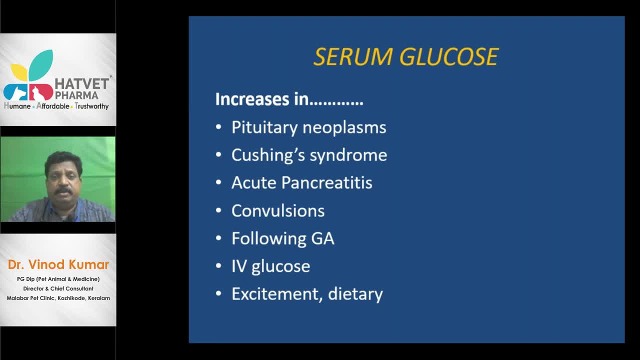 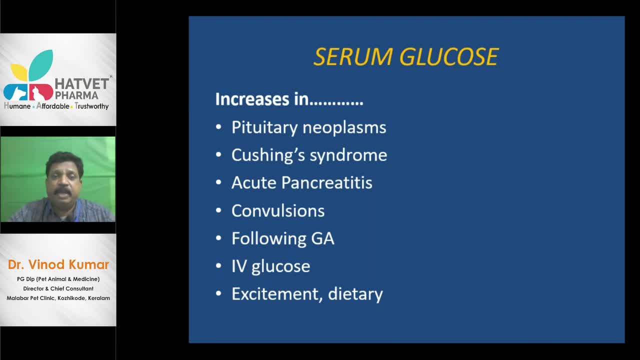 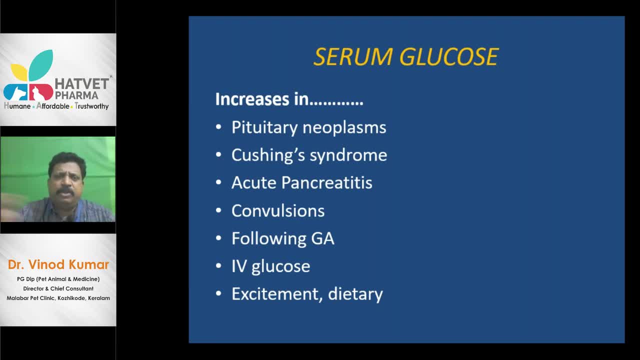 which is situated in between the folds of the descending and the ascending duodenum, And the pancreas, has an exocrine part and an endocrine part. We all know that the exocrine part releases digestive proteins, their enzymes, And the endocrine part releases the endocrine 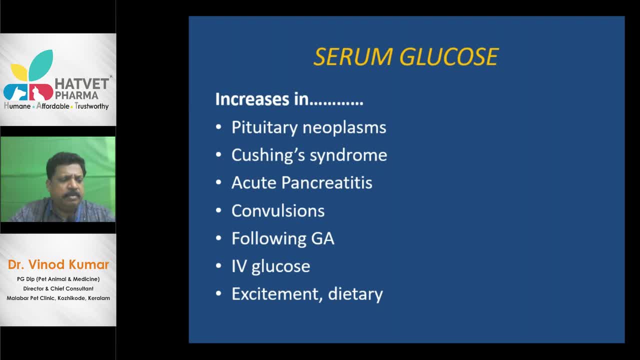 cells and the beta cells, And the endocrine part has the alpha cells and the beta cells. Of course, the endocrine part has the alpha cells, which produces glucagon, which increases the BGL, increases BGL and increases the beta cells. And the beta cells are alsootymic. 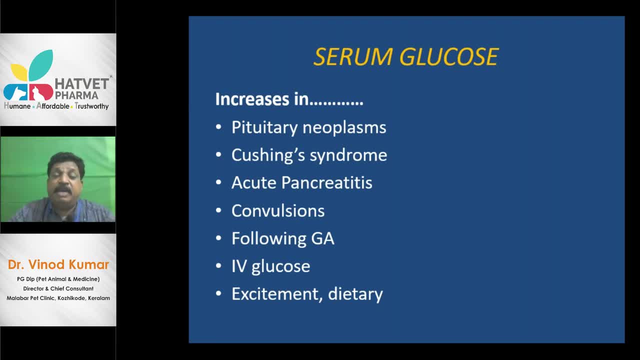 So the endocrine part releases glycogenesis, increases the beta cells and will produce increases the blood sugar content and we have the beta cells. They are found histologically as islands, We say the islands of Langerhans. It releases our very important hormone, insulin. 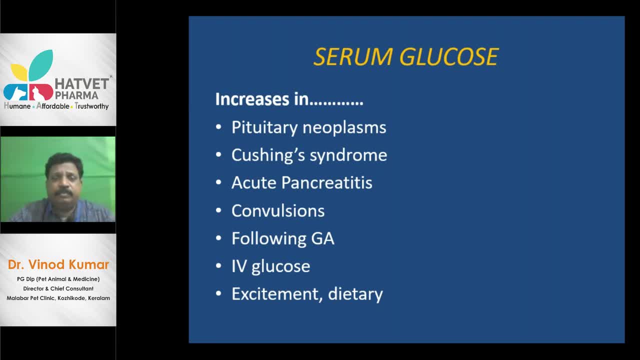 It is a double-chain molecule. We all know about insulin And this insulin is necessary for the intracellular metabolism of sugar. Of course, we all know this. In an acute pancreatitis, in an acute necrotizing pancreatitis, what will happen? 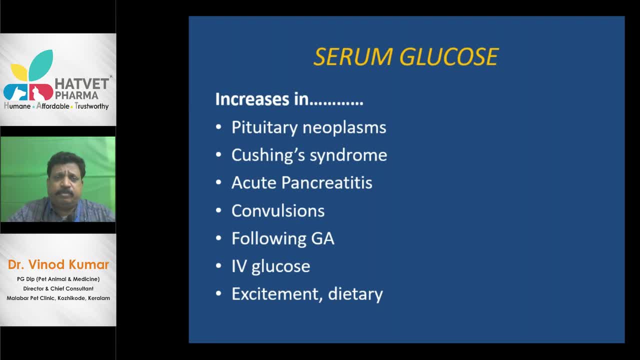 The secretory cells of both the endocrine and exocrine portion will be destroyed And very only a feeble quantity of insulin will be secreted. So what will happen? The ultimate effect is hyperglycemia. So that is in acute necrotizing type of pancreatitis, And it is 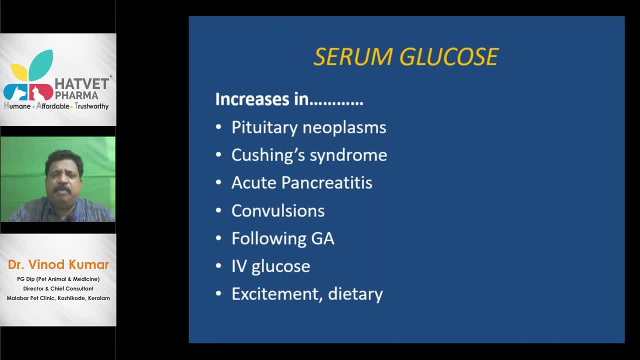 very easy to determine, because the dog will be having severe vomiting, acute abdominal pain, diarrhea, high rise in temperature, fever, etc. Then in convulsions blood glucose will increase Highly substantial Because in a Glucose is stored in the liver and the skeletal muscles as glycogen. In convulsions there is more demand of energy for the convulsions and contractions and so tremendous quantity of glycogen will be immediately metabolized to form glucose. 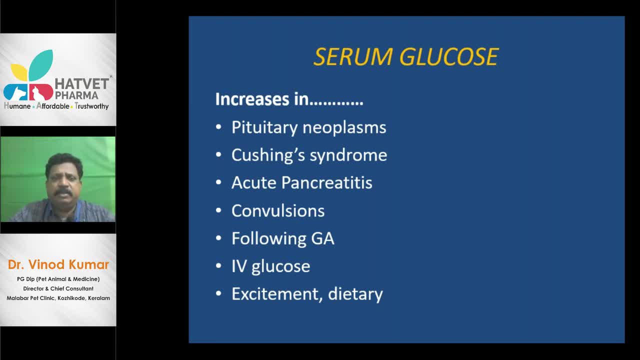 And this glucose is being metabolized for need of ATP. So convulsions produces hyperglycemia. Then following general anesthesia, Why during general anesthesia there is a transient hyperglycemia. That is why it is said during a deep general anesthesia. 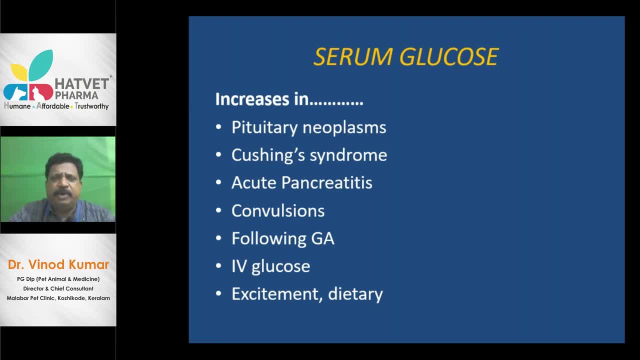 Don't put any glucose containing fluid as IV fluid. Why? Because during general anesthesia, hyperglycemia occurs. Why? Because glucose in the blood will be immediately metabolized. Okay, that is great. Because it should not be. It should be sustained in the system. 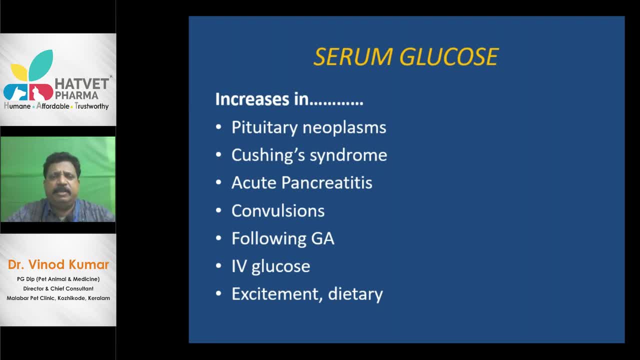 It should be immediately metabolized, And so the glucose is being metabolized in the body by three methods: Number one, the glycolytic pathway, Number two, the Krebs cycle, And number three, the pendo's phosphate pathway. Pendo's phosphate pathway. 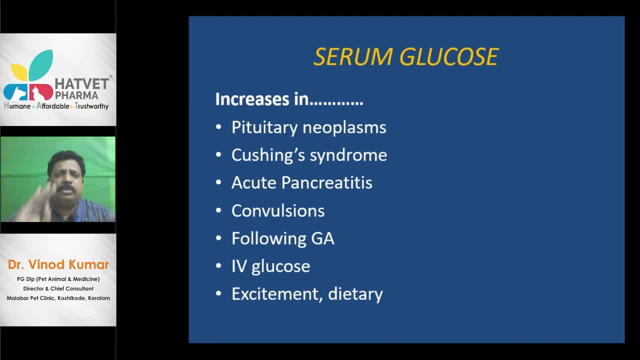 So the glycolytic cycle, the Krebs cycle and the pendo's phosphate pathway. So in all the somatic cells in the body except the brain, glucose is being metabolized through glycogen, Glycolytic pathway and the Krebs cycle. 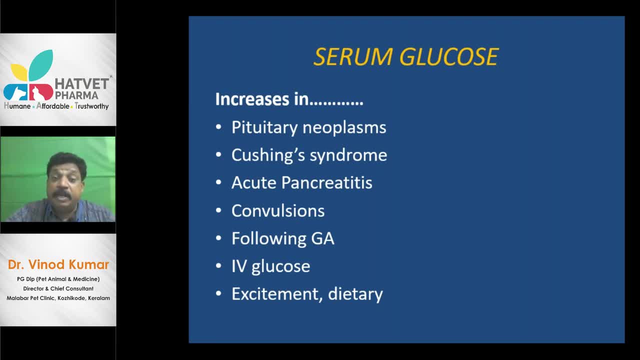 But in the nervous system, in the neurons, there is no glycolytic cycle or pendo's phosphate Glycolytic cycle, or Krebs cycle. Glucose is being metabolized in the brain, in the brain cells, through pendo's phosphate pathway. Almost 50% of the glucose is burnt in that way. 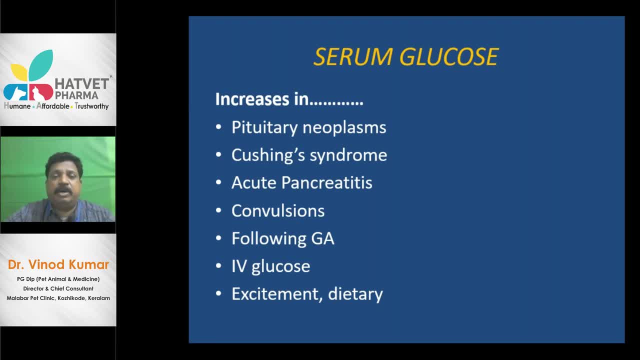 Because it is a master organ, It is a computer, It needs lot of energy as ATP for processing, storage etc. So if there is a hypoglycemia or reduced glucose, All the functions of the brain will go impaired And metabolic arrest and cell death occurs. 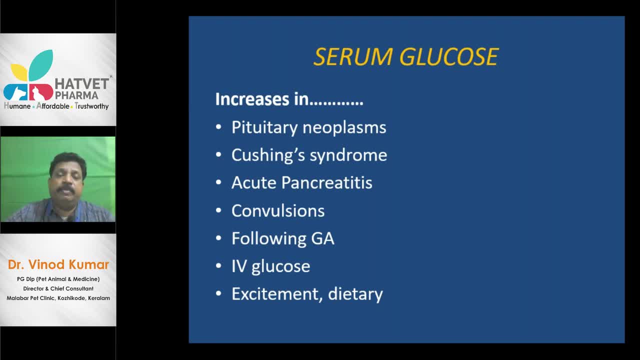 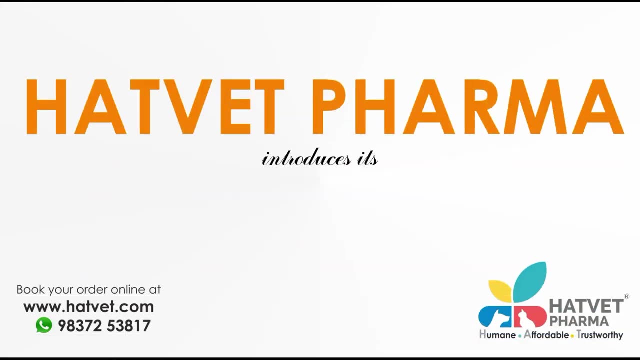 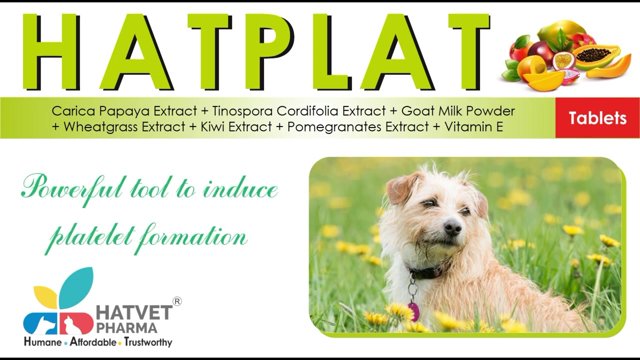 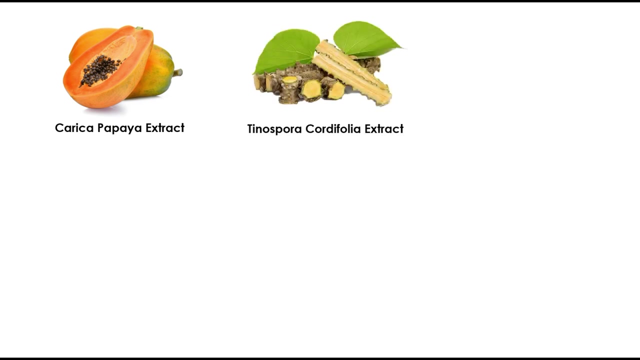 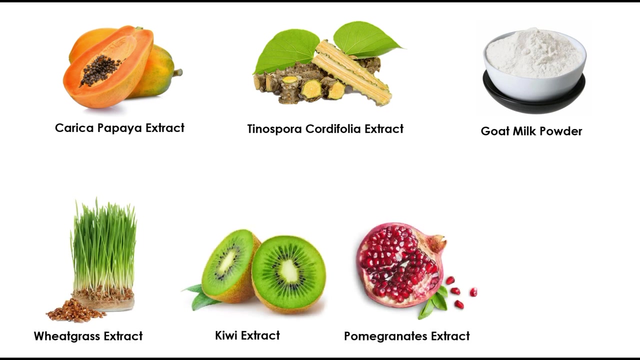 So, when there is a depression of these brain cells, As in the case of general Anastasia HATBLAD Tablets, Powerful tool to induce platelet formation. Carica papaya extract, Tenospora caudifolia extract, goat milk powder, wheatgrass extract, kiwi extract, pomegranate extract and vitamin E tablets. 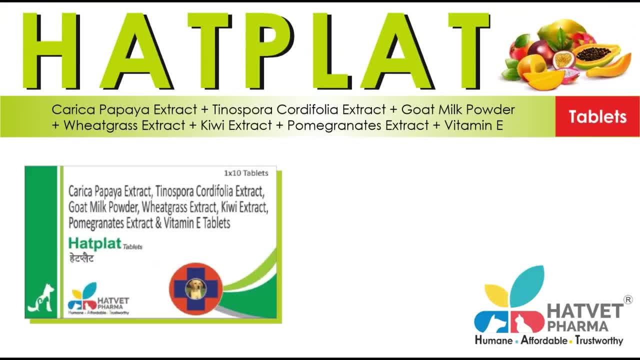 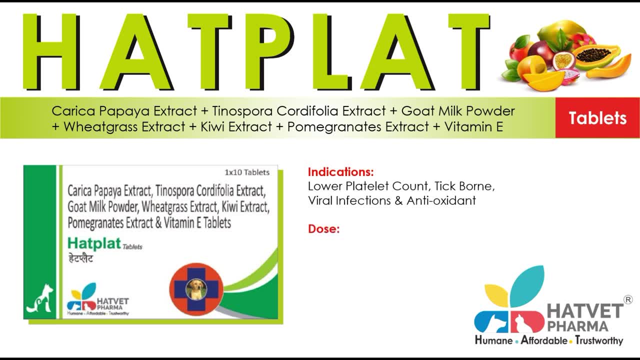 HATBLAD Tablets. Indications: Lower platelet count, Tick borne viral infections and anti-oxidant Dosage for dogs- Body weight less than 10 kg. 1 tablet once a day. Body weight more than 10 kg. 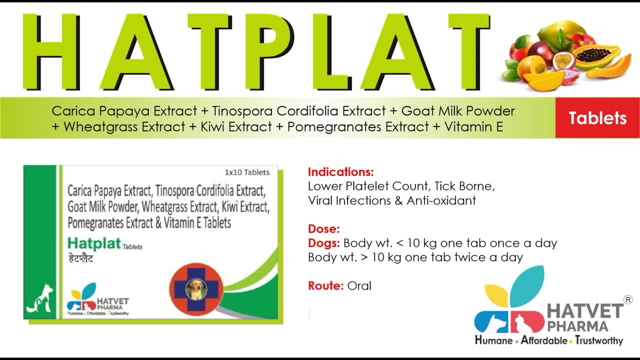 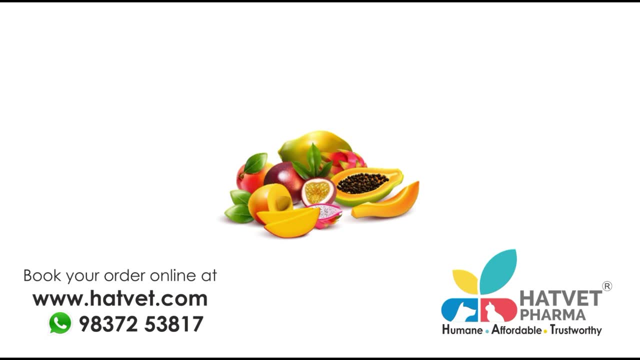 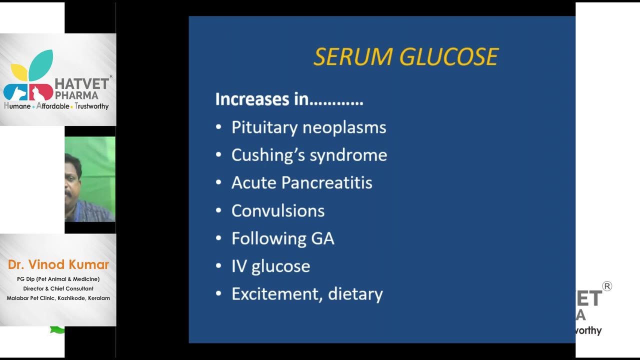 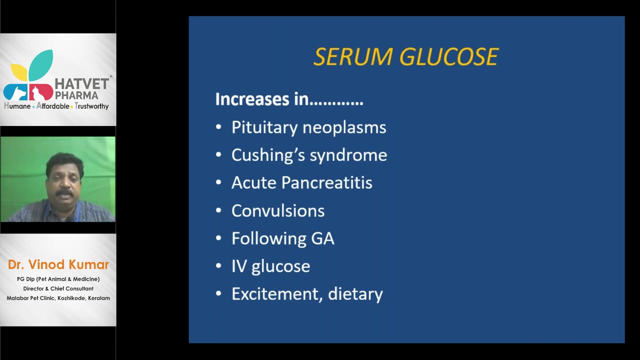 1 tablet twice a day. Root Oral Presentation: 1 x 10 tablets. You can book your order online at wwwhatbladcom, Looking forward to a long lasting business experience. Thank you. There will be slowing down of glucose metabolism through the pentose phosphate pathway. 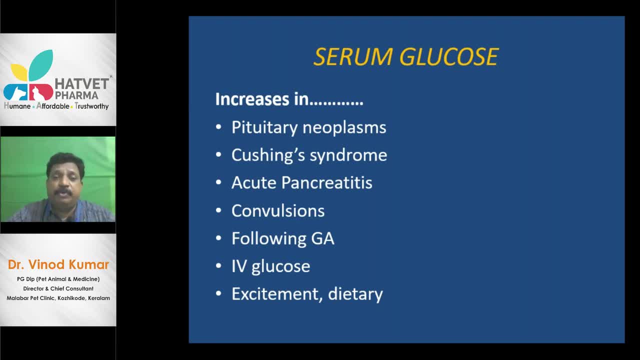 As a good quantity of sugar is being metabolized through the pentose phosphate pathway, And when it slows down, There is definitely A chance for Accumulation of this sugar in the blood, And this occurs Quite naturally, And that is why 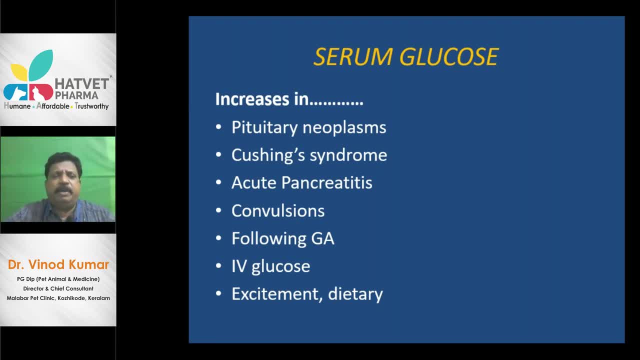 During brain depression, Like whatever it be, Maybe a coma Or could be general anesthesia. There will be Hyperglycemia, So let us ask you something regarding it. Let us come to it. See, in your clinic, A labrador is presented. 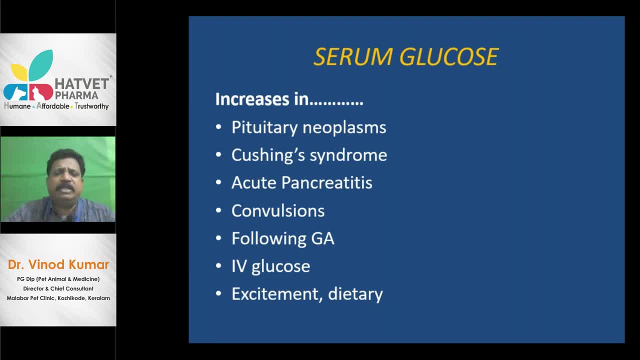 You suspect. See the labrador is having Polyuria polydipsia. Look at PUPD. You are happy. PUPD is a classical indication of Hyperglycemia And you need to know What is the cause of this hyperglycemia. 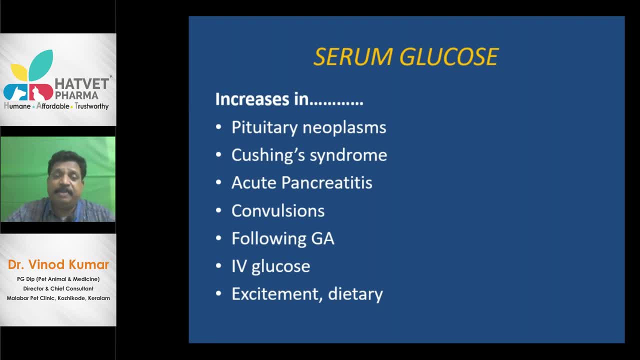 Suppose the dog is having Some skin lesions like Thin skin, Calcinosis, cutis, Hyperpigmentation, Pruritus, Lichenification, Allopathy, etc. What will you think? All these are classical Signs of Cushing syndrome. 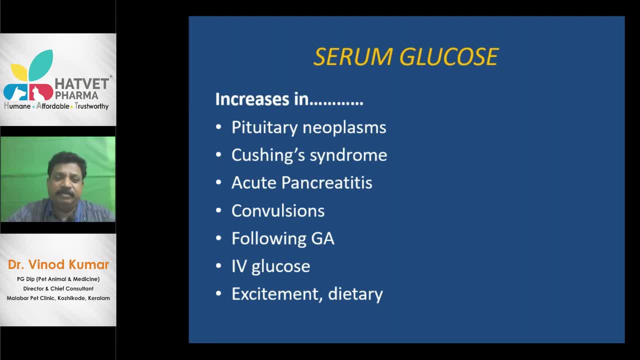 You need to take the blood. You are very happy. Well, Happily, You go near the dog, You will take the forelimb of the dog Without any pain, Without any muscle, Simply you will poke And you will draw the blood. 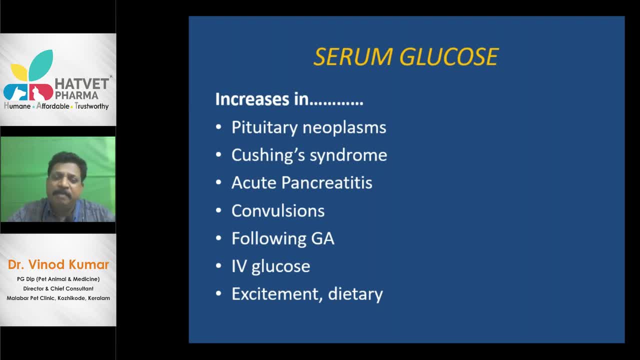 The dog won't do anything Because it is a labrador. You are very happy, The clinician is happy, The client is happy, Everybody is happy. So what about the condition In a biting, ferocious Rottweiler? 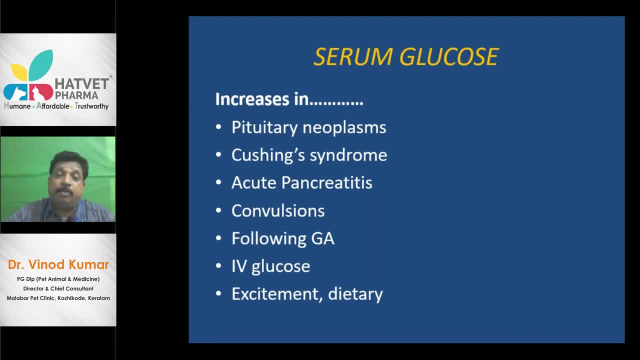 Can you do that? Suppose he is very aggressive and ferocious, You need to check the blood. What will you do? Generally what we used to do: We will sedate the animal. We have our international drug, Psilocine, Then another international drug. 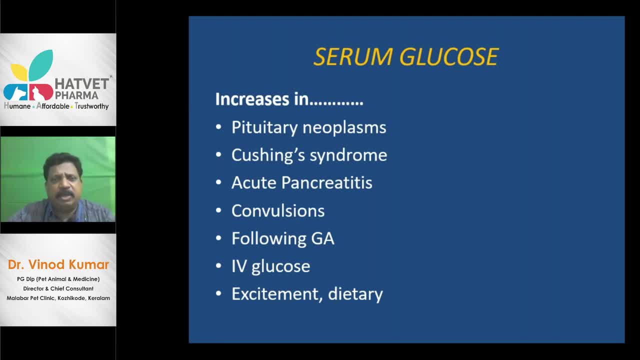 Ketamine. These are the commonest drugs used for sedation- And also Anastasia. We need not sedate it Because it is Rottweiler. We anesthetize it Anesthetize by giving the blood. It is an intramuscular injection of. 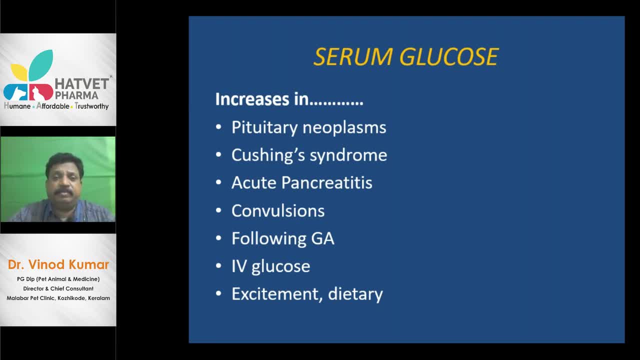 Psilocine And sometimes ketamine. So after that we will take the blood. What will happen When we take the blood And estimate the glucose? What will happen In this case? You find Hyperglycemia. You say 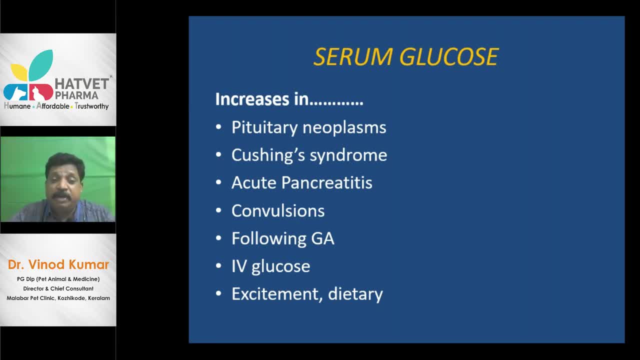 Oh, you are right, What you thought were right. This hyperglycemia Is only because of Your sedation Or Anastasia in the dog, And it will reverse After, when It has become normal. So here Our viewers may ask. 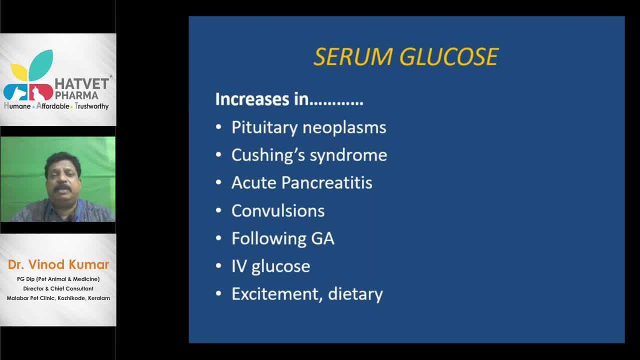 Then what is The next option? No option at all. If it is a Very big, ferocious Rot wheeler, Then better You put it inside the squeeze cage. Squeeze it well At the time you go near it. 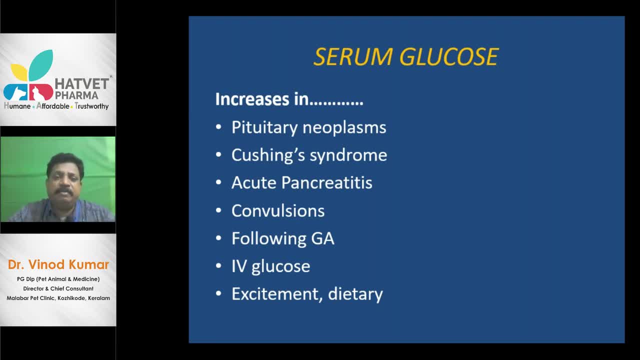 Take out the limb, Then take the blood. We used to do it. That is the only way. So, following general Anastasia, There will be a hyperglycemia. Then, Following IV glucose, Yes, It will produce Hyperglycemia. 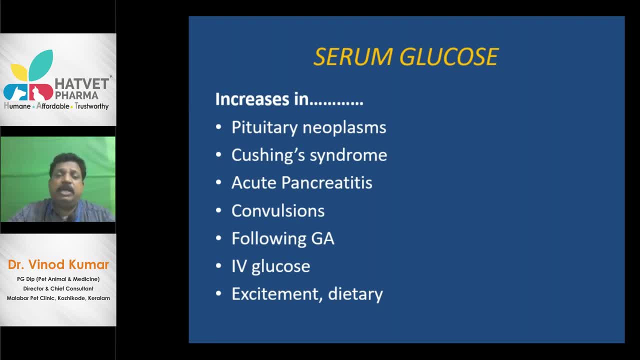 That is why in my fluid therapy course I said: Don't give any glucose containing fluid In A recumbent Death impending patient Which is in a critical condition. So don't give glucose In such a critically ill dog. 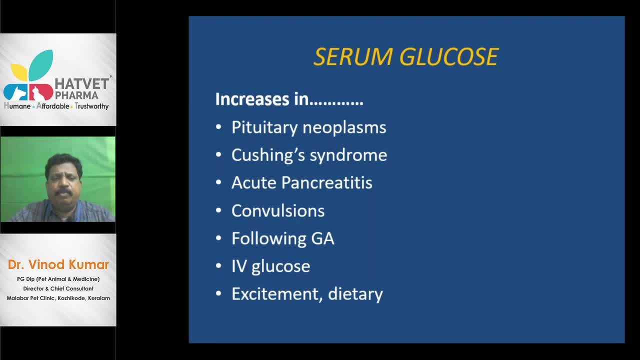 It may die. It may die Why It exacerbates the Hyperglycemia, Because already it is Going to die And the body itself will release Corticosteroids As a measure to save the animal, As a measure to increase the 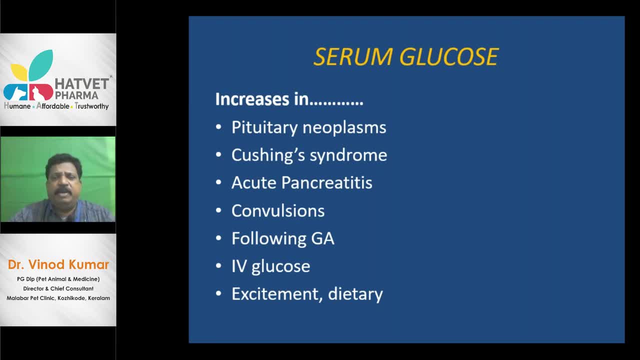 Blood glucose and save the animal. And during that time, Before death, There will be a hyperglycemia. And during that time You are again giving Glucose containing fluid. What will happen? The hyperglycemia Will exacerbate. 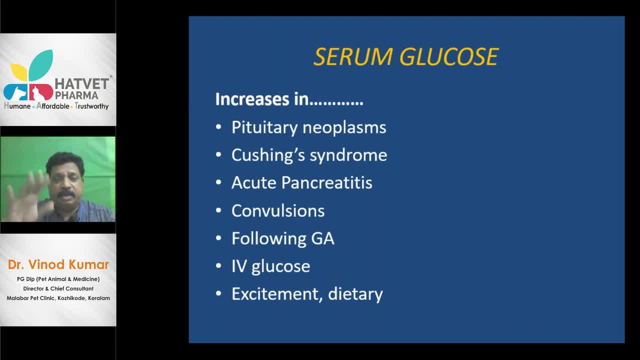 And the patient will die Only because of your Faulty fluid therapy. Okay, So IV glucose always Produces hyperglycemia, But In a normal animal There will be hyperglycemia For some time. Just for minutes. 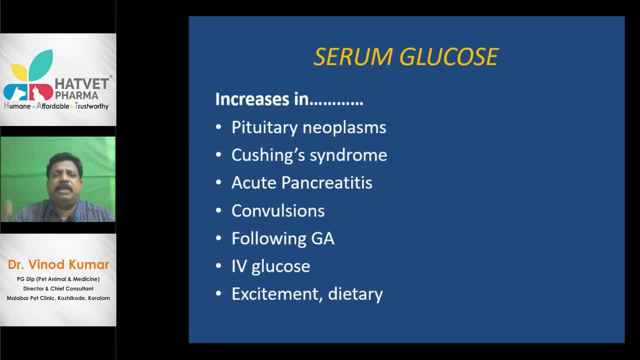 And then It will be disappearing suddenly Because it will be easily metabolized. Then Hyperglycemia occurs In excitement, Of course Highly substantial, Because during excitement There will be The release of catecholamines Pure. 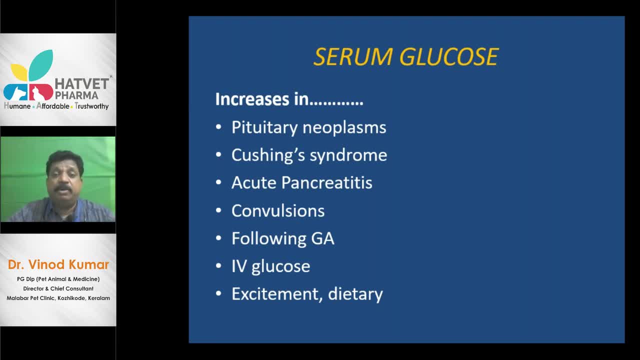 We have the Flight Hormone, That is, epinephrine Adrenaline. It is being released So In excitement and fear, There will be a transient hyperglycemia Because Catecholamines Will split. 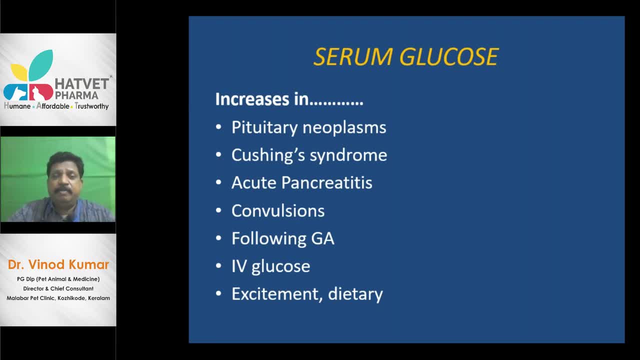 The carbohydrate And There will be An increase. See for the flight Flight etc. There should be A high glucose level of blood, So A transient hyperglycemia In excitement occurs, So also dietary hyperglycemia. 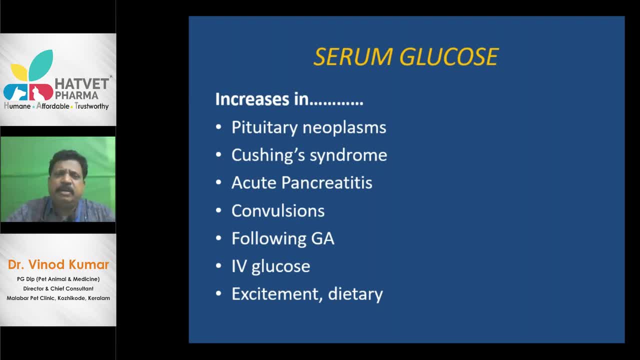 Of course It is a universal concept that If you eat 5 jalebis For Definitely after half an hour, Your blood glucose level increase. It is quite natural, Highly substantial. It is known as Dietary hyperglycemia. 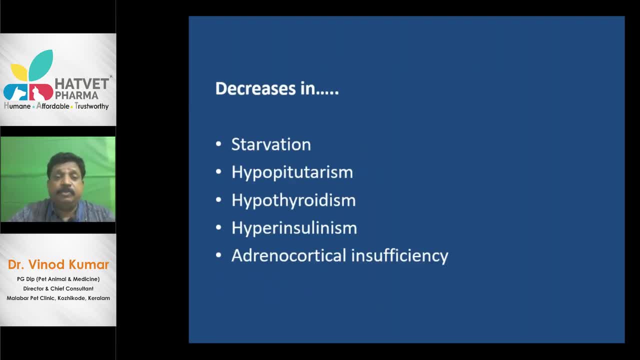 There are certain conditions Where The blood Glucose level decreases, Which is known as Hypoglycemia. It occurs in starvation, Of course. In starvation occurs Because We are getting Our sugar From the food. 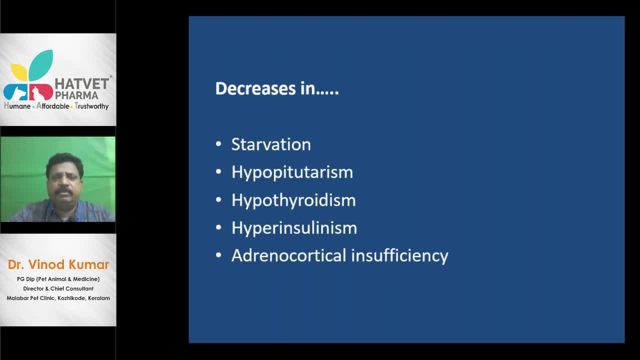 From the water. there is nothing From the food As complex polysaccharides Or starch. It is being converted to glucose In the ruminants. we know They can convert Cellulose to glucose, But we do not. 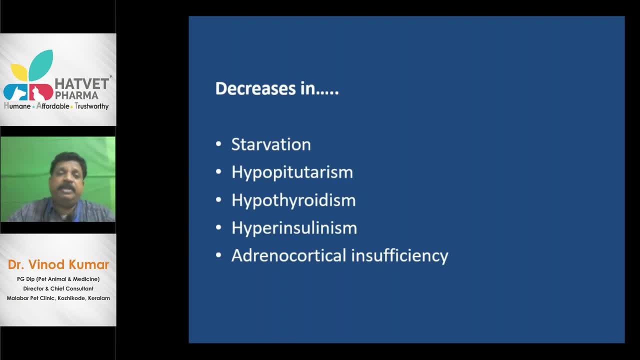 We do not have such a Efficiency, Such an efficiency, Because We have a non-ruminant stomach. We, the dog, The humans, The cat, The horse, Everybody Anatomy And cannot convert Or digest Cellulose. 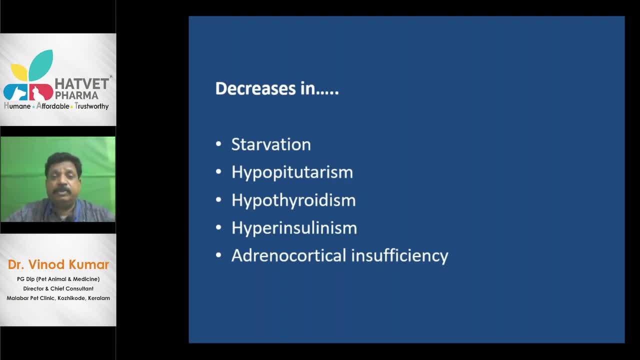 But we can digest Carbohydrates such as Starch. So in starvation All these will be restricted And hypoglycemia Occurs- The same as Hypopituitarism. What happens in hypopituitarism? 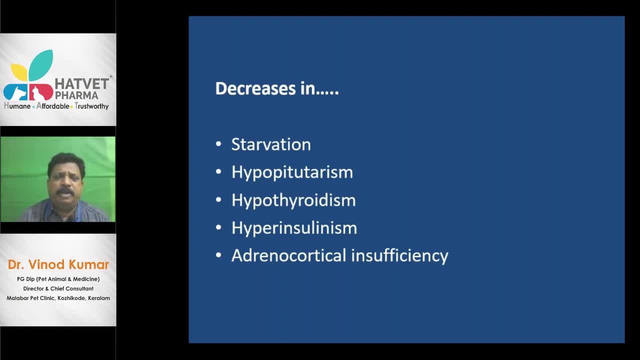 Just The same as Ptutri Or Ptutri Neoplasia. There will be Less release of ACTH There by The adrenal cortex Will not be stimulated, So less Amount of Corticosteroids. 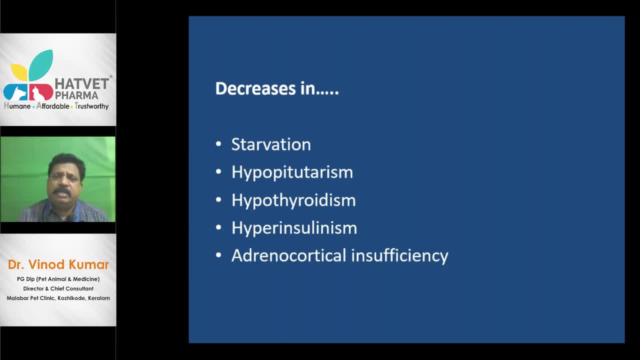 From the adrenal cortex, Less gluconeogenesis And less blood sugar- Quite natural- And blood sugar level Sometimes decreases in Hypothyroidism. Of course We have Described these things In our Dermatology class In hypothyroidism. 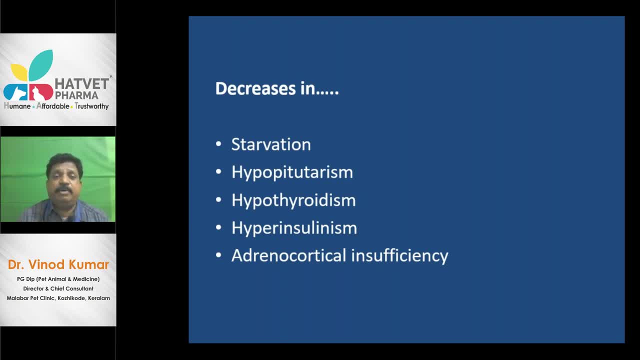 We know Thyroxine hormone is essential for Glucose metabolism. If Thyroxine hormone is low, Several things go: Hypo, hypo, hypo, hypo, hypo, hypo, Hypotension, Hypoglycemia, Reduced cardiac output, Reduced peripheral circulation. 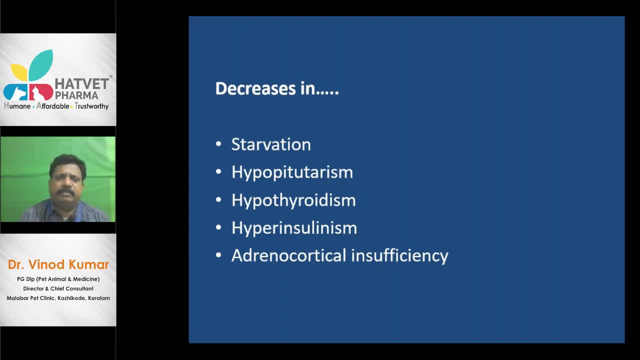 Etc. So when there is Hypotension In hypothyroidism, Number one is Reduced Gluconeogenesis, The number two is The animal itself Will be lethargic, And so There will be oligophagia. 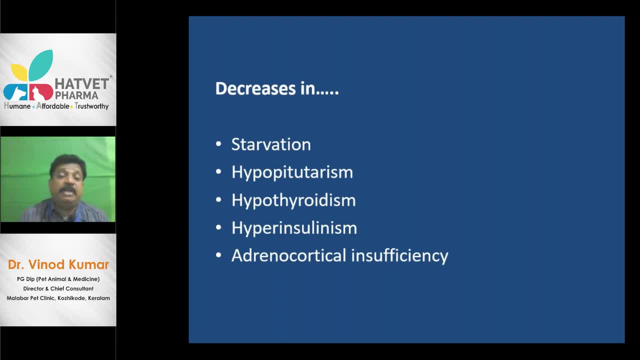 It's not anorexia. Anorexia and oligophagia are Little bit different. Anorexia means No hunger at all. It is A central Or An organic Dysfunction. But Oligophagia means: 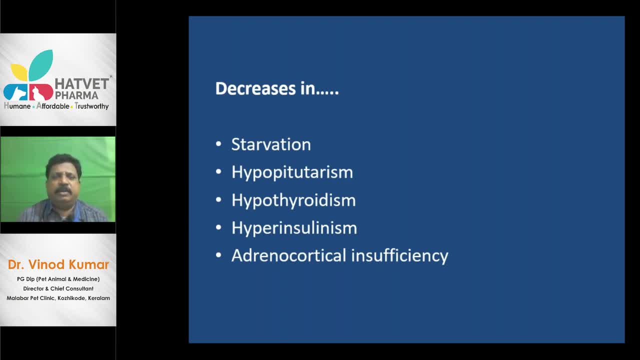 It is eating less. Anorexia means Not eating anything at all. Oligophagia means It is eating less Due to some factors. Maybe it is having Painful lesion, Painful oral lesion. Maybe it is having 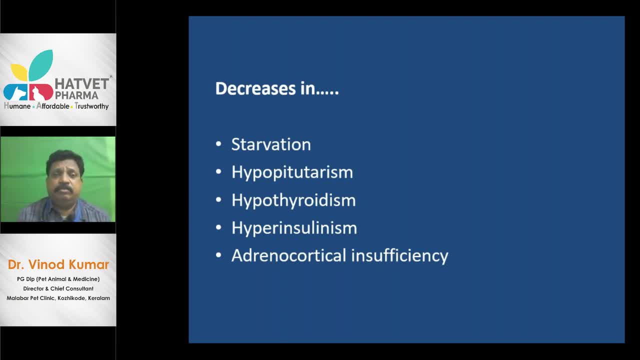 Dysphagia, Because It is having Swollen tonsils. Maybe it is having Odynophagia. What is odynophagia? Odynophagia- Painful deglutition. Painful deglutition. 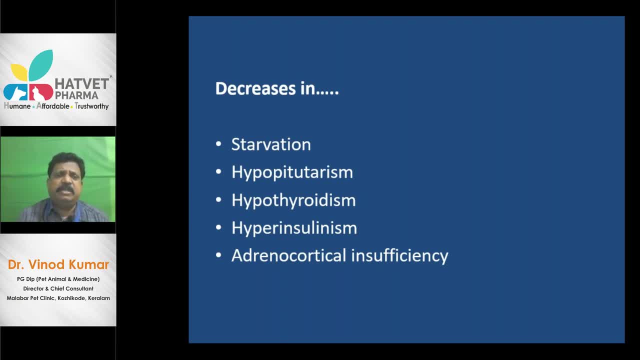 Due to Severe ulcerations Or oropharynx Painful defecation, So Oligophagia occurs. Oligophagia occurs Due to odynophagia, So all these Can lead to. 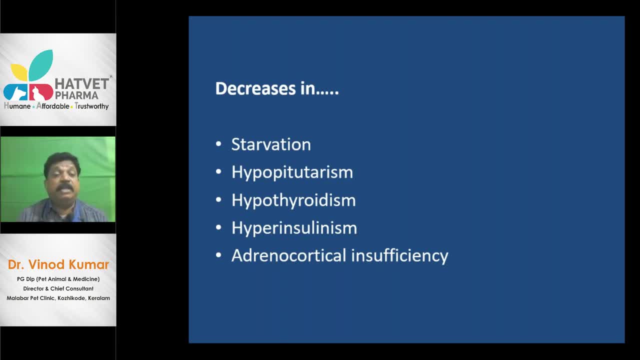 Less intake of food And also When there is hypothyroidism. The animal will always be lethargic. It cannot go even to the source of food And eat. It cannot even walk to the source of food And eat. 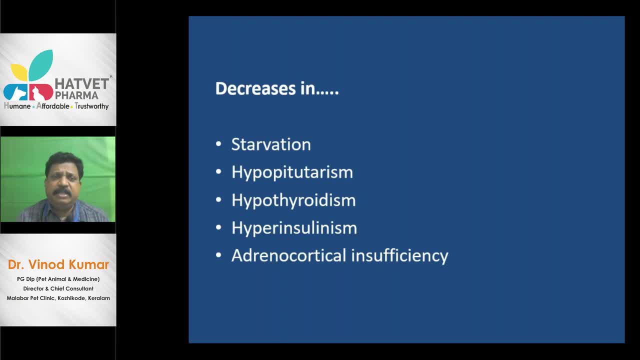 That much it will be lethargic And produces Hypoglycemia. Got it Then In some pituitary, In some pancreatic tumours. There is a condition known as insulinoma Is not so common That. 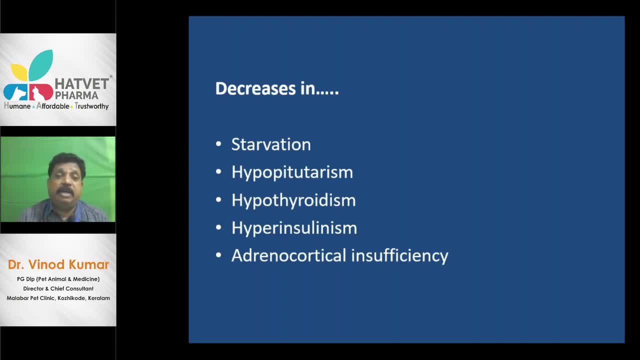 My friend, Pathologist of Phukot veterinary college, Has Diagnosed a case of Insulinoma in a dog Very recently, Dr Hamza, And so This insulinoma can induce Hypoglycemia. 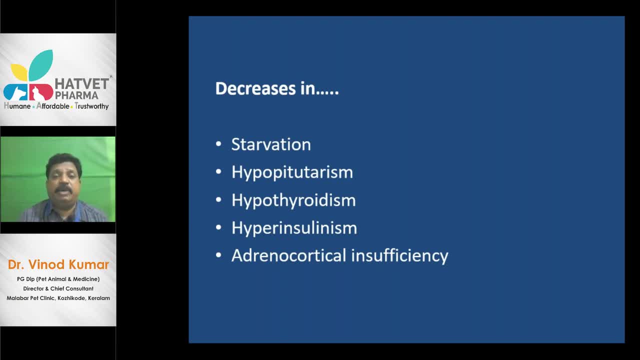 By releasing More quantity of Insulin. Insulin is glycolytic, So produces Hypoglycemia, Then Adrenocortical Insufficiency. See It is substantial In adrenocortical insufficiency. 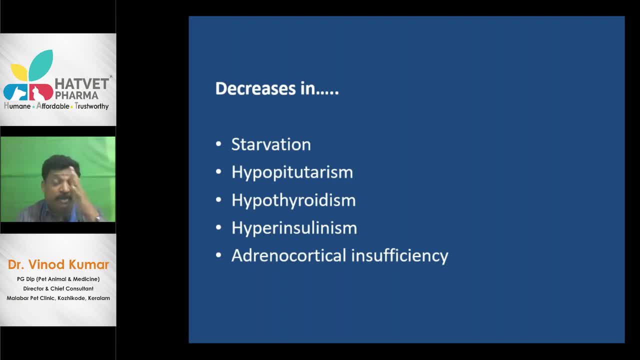 The adrenal cortex, Which has the Glycosidata, Will be deficient To produce Corticosteroids. It can happen As an idiosyncratic disease There by. You can induce it By certain drugs, For example. 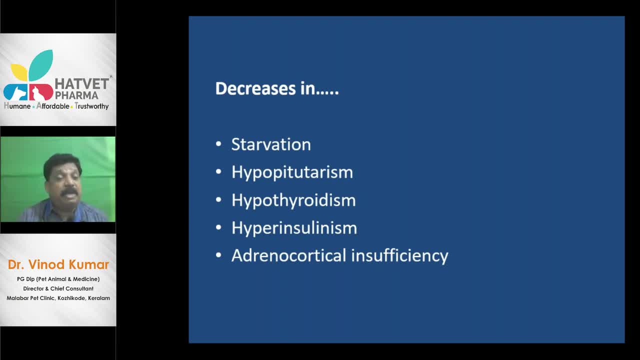 The drugs used against Cushing syndrome. We have discussed about it: The mitotine And even Ketoconazole. I have a case of such a Such a disease I have mentioned in my Dermatology class Where A retired headmaster presented his 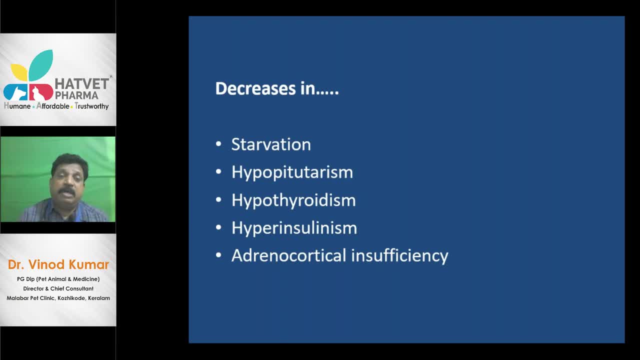 Labrador With polyuria polyphagia. Ultimately I diagnosed it as Cushing syndrome. I asked Ketoconazole For 20 days And then come back. He gave it for 5 or 6 months. Came back. 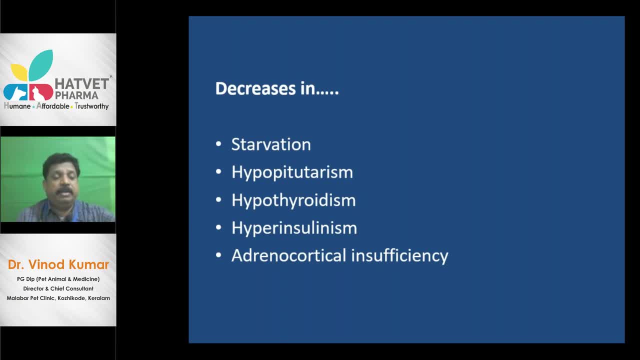 With severe depression, Severe vomiting, Catechsy, etc. The fatty labrador, The obese labrador, Was looking like a Doberman During that time When he presented A second time. So This Cushing syndrome. 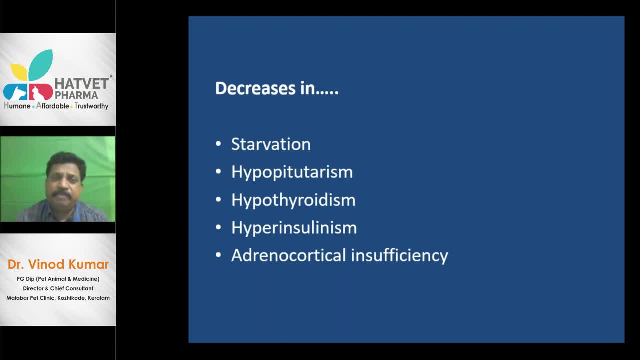 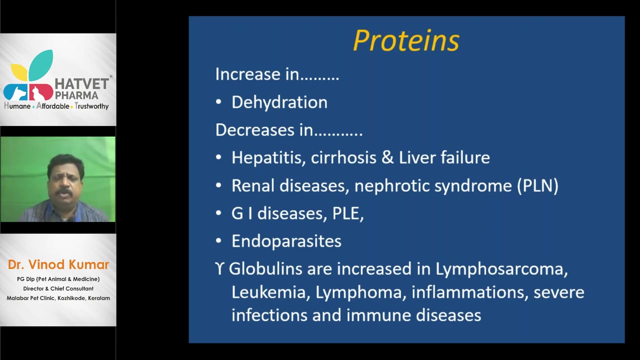 Was converted to Addison's disease By this Retired headmaster By administration of Ketoconazole Orally. So It produces Hypoglycemia. There are Proteins in the blood. We know the proteins. 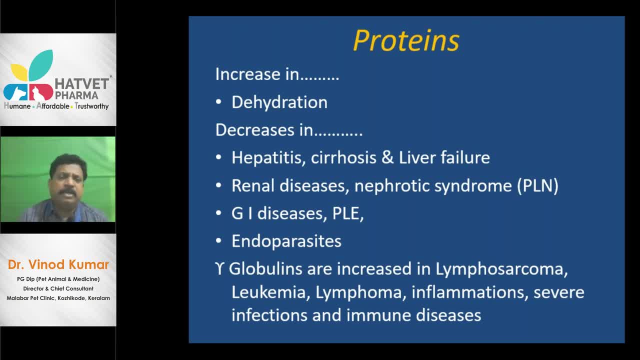 Of course we have The total proteins. Mostly we take the total proteins Or we take the protein fraction As the albumin And the globulin. If we are, We take the Globulin fraction again, Like the alpha globulin. 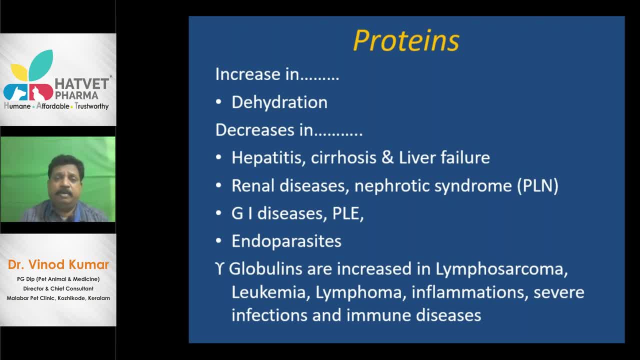 Beta globulin Or the gamma globulin. But we need not, We, the practitioners, Need not go after all these things. Just the total proteins And the Albumin globulin ratio And If the total proteins Will increase in. 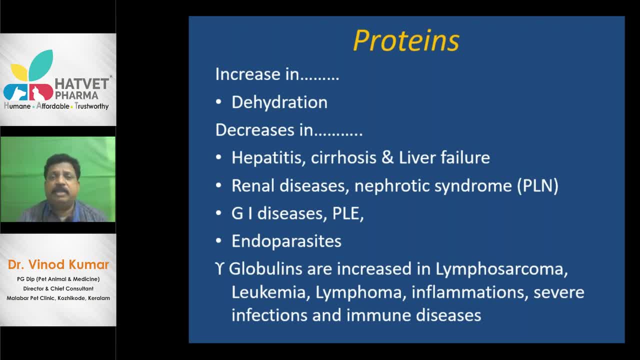 Dehydration. Of course It is Substantial, Because there will be hemo concentration, Plasma concentration, Total solids Will not be lost, But the plasma will be lost And so the proteins will be concentrated And there will be increase in protein content. 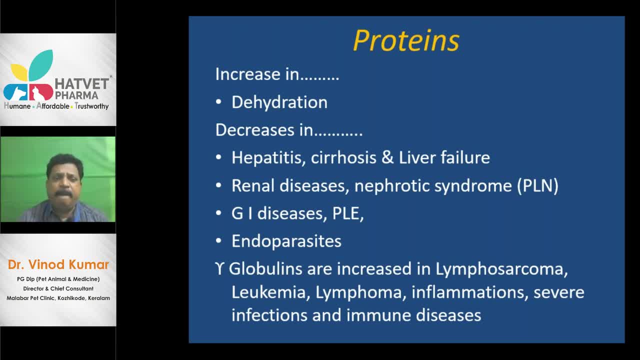 That is What is happening in Dehydration, But proteins Decreases In several conditions. We all know that Proteins are being By the liver, So If there is a hepatitis Where The hepatic cells, The parahematous, 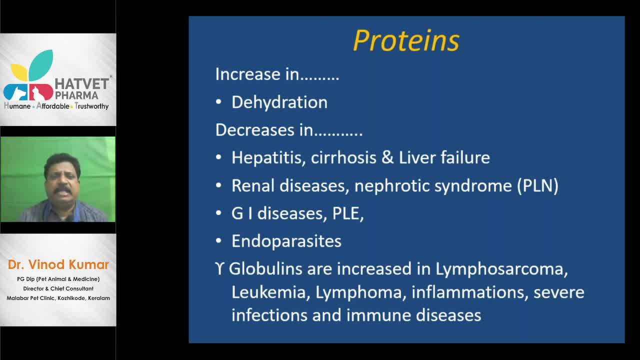 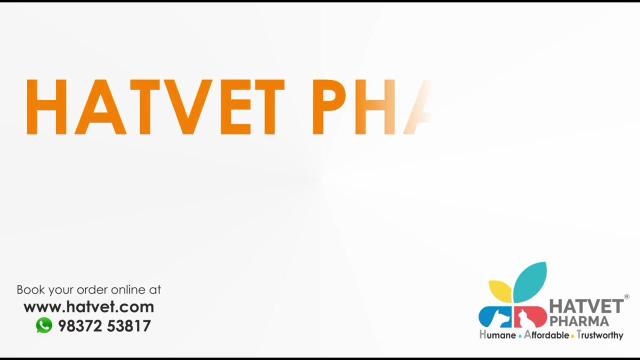 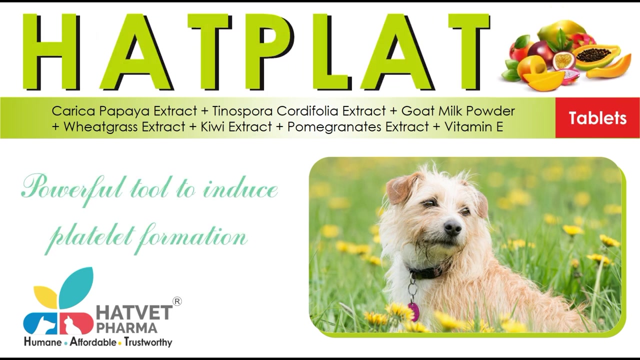 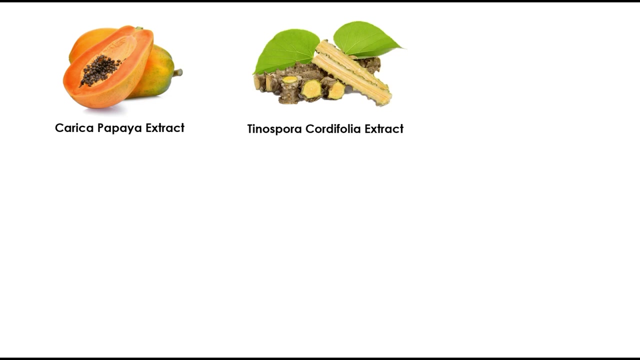 Cells of the liver Are destroyed Or, in cirrhosis, When The complete architecture of the Liver itself has Been destroyed. Liver is the Main seat of Protein synthesis. The liver can be Dehydrated. What's? 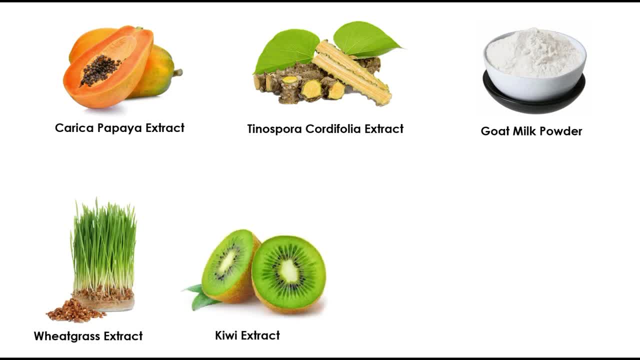 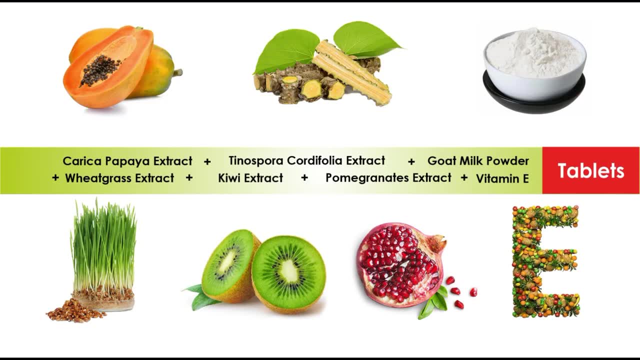 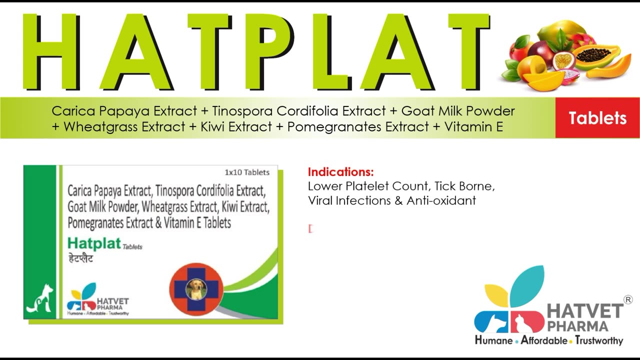 This. That is Some Medicine And What is The Earth? Loss Of Protein: kg 1 tablet once a day. Body weight: more than 10 kg 1 tablet twice a day. Root Orel: 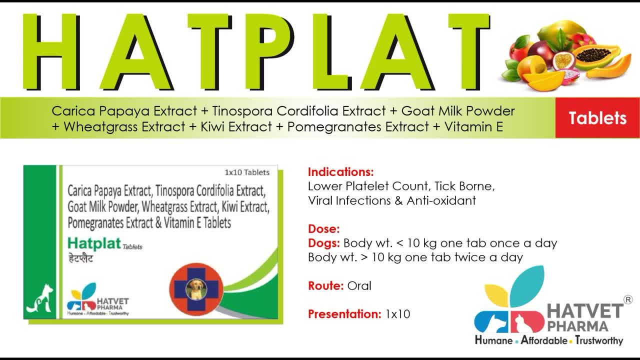 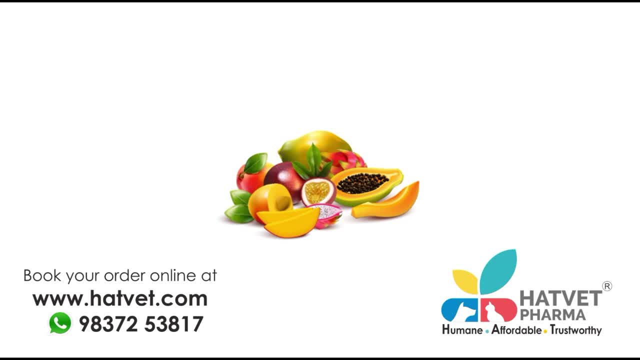 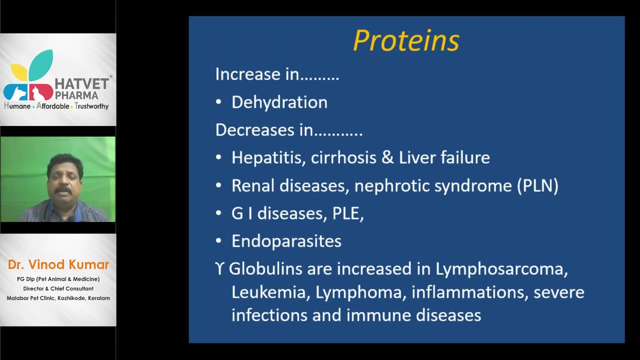 Presentation 1 into 10 tablets. You can book your order online at wwwhatredcom. Looking forward to a long lasting business association. Thank you, It is quite. it is substantial that in chronic functional defects of the liver, such as in. 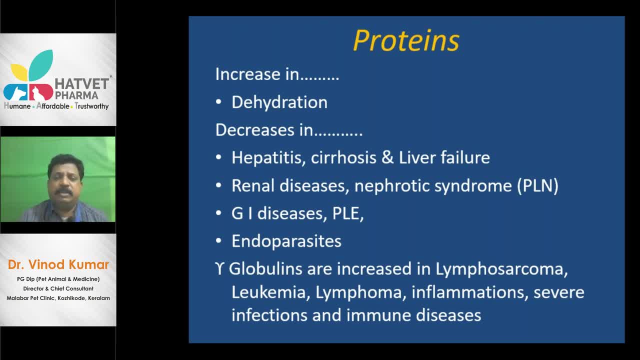 hepatitis or cirrhosis and concomitant liver failure. there is hyperproteinemia. So we know the outcomes of hyperproteinemia: The difference in the specific gravity of the plasma, Extravasation of the plasma, formation of third-space edemas, that is, ascites, etc. We 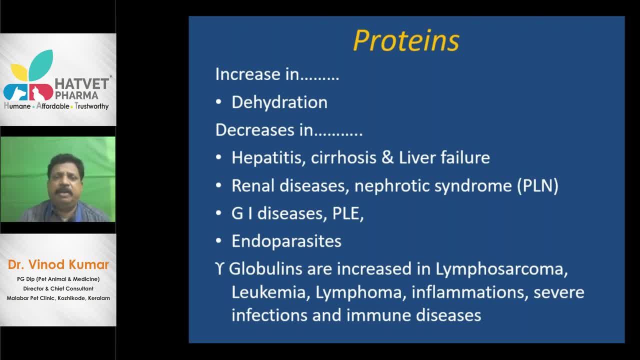 all know it. What happens in hyperproteinemia, Then in renal diseases- nephrotic syndrome, but not in all types of renal diseases, Mainly polyuric renal diseases where more amount of protein will be lost through urine. There was a case of a Labrador which was presented and the client says that it is lethargic, all. 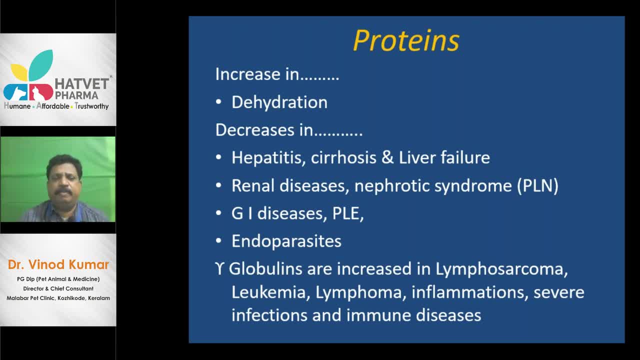 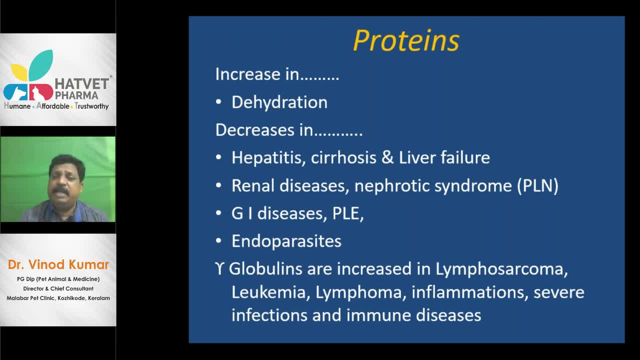 nothing was abnormal, But in that there was a slight decrease in total proteins, Assuming that, see, there were no other findings like the PE findings. the physical examination findings was also unremarkable. Nothing was there. What can we do? He says it is lethargic. 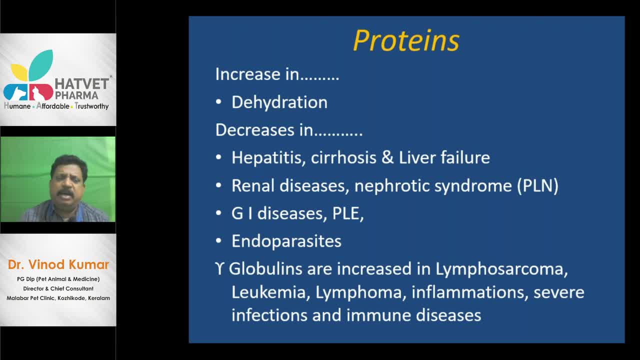 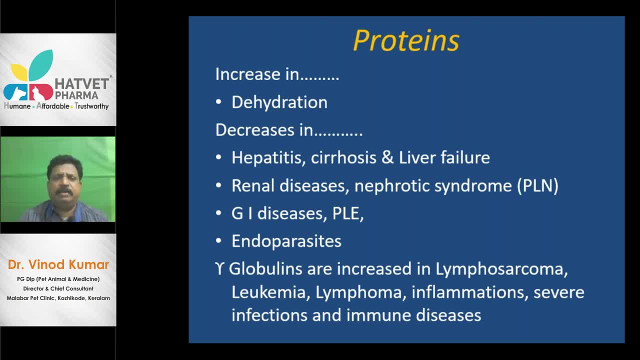 there was no bile salts, no bile pigments, no blood, no ketone bodies, nothing at all. But the proteins was 3+. There was proteinuria, Proteinuria, And so I have to see what the cause of proteinuria is. Now I got the clue. Now I got the clue. 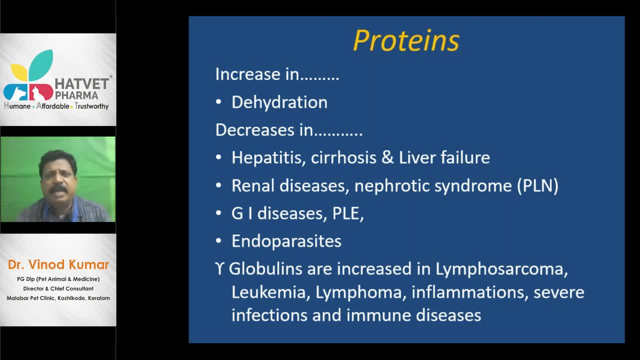 There is a 3% proteinuria. In that case I have to determine the cause of proteinuria. I hope by this time I could get a clear diagnosis. Yes, I subjected the kidney for other tests. Now I know that there is a problem with the kidney. I subjected the kidney for 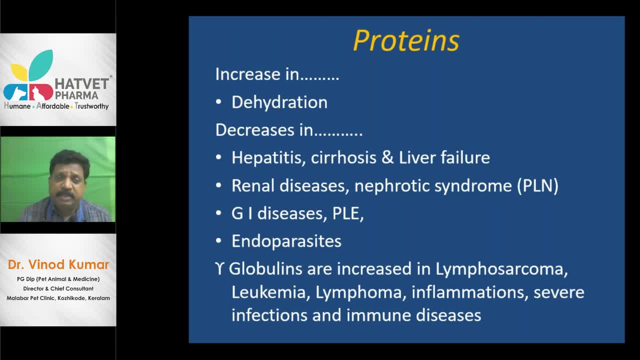 different tests Company. amongち probability for different tests statisticians. 好 Tian激agua D 쉬 16, Sun loyalty Zone analysis. 龏龍 e Di vertex. like a kidney function test crash returns a random result: Crescent deaths, severe kidney. 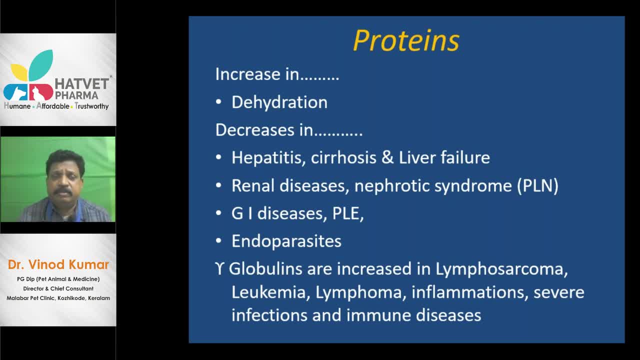 growth and death of 10%. these factors will be documented after the test Here: J鈸s, creatinine, blood urea, nitrogen, uric acid, all these things, And I saw nothing. Everything was normal. It was ultimately subject to ultrasound examination. On ultrasound examination only. 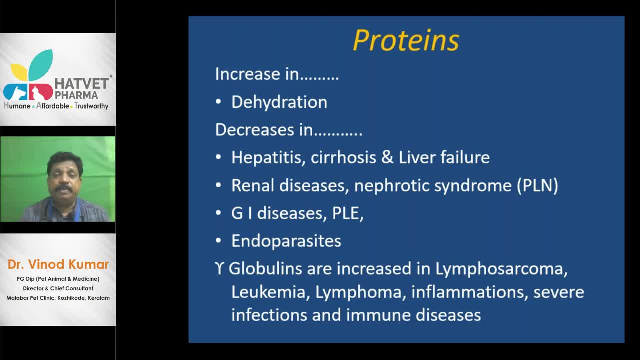 on close kidney observation I could find that there is mild to moderate cortical edema. So ultimately it was diagnosed as a case of developing immune mediated cortical nephritis- glomerulonephropathy- See. it is written in textbooks also In my art of pathological clinical practice also. 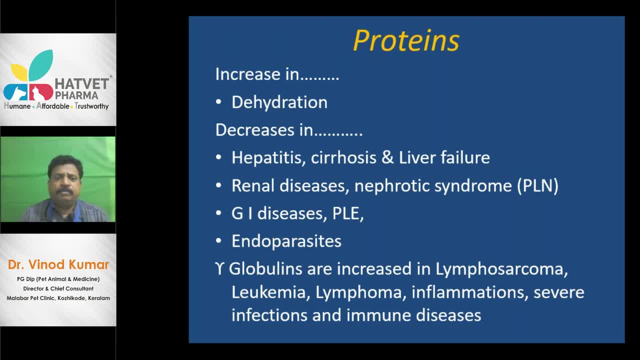 I have written this case. So why? there is a 3 plus proteinuria. It is known as a PLN, a protein losing nephropathy. So in renal diseases, in nephrotic syndromes, etc. there will be protein losing nephropathy. 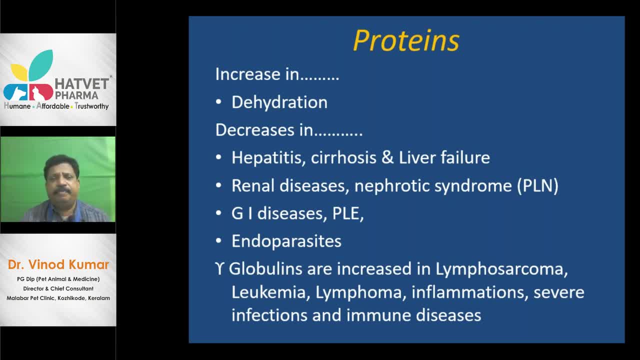 So in renal diseases, in nephrotic syndromes etc. there will be protein losing nephropathy. So in renal diseases, in nephrotic syndromes etc. there will be protein losing nephropathy producing hyperproteinemia. Then in GI disorders, any erosive GI disorders, for example in acute 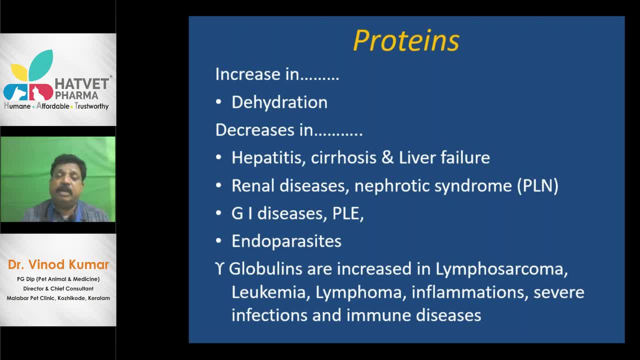 parvoireal enteritis, there will be severe protein loss through the loose tools. Thereby we call it as a PLE protein losing enteropathy. That is why we are giving aminobutans- aminobutans. 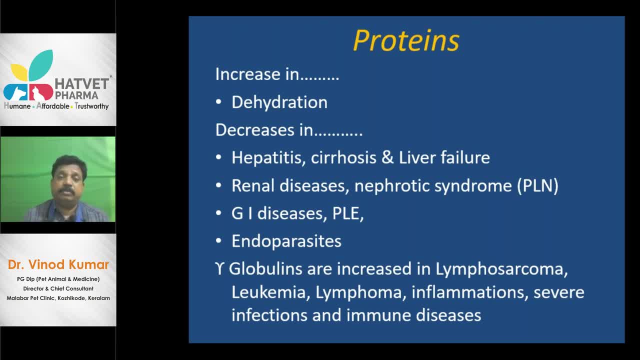 and amino acid infusion in parvo. So that will be hyperproteinemia in parvoireal enteritis, Then in endoparasitic diseases it could be ankylostomes, could be toxicara, it could be diphalidium tapeworms. 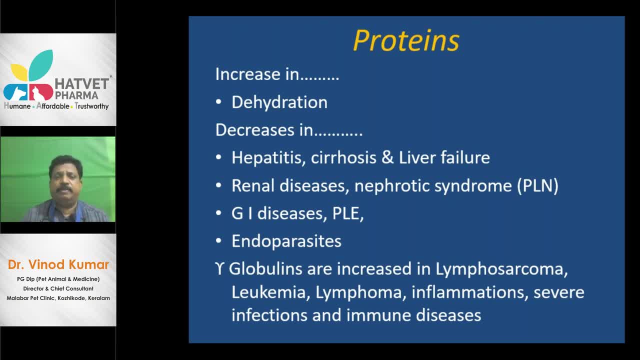 Nematodes are hookworms. The commonly found nematodes are the roundworm, that is toxicara canines, the hookworm that is ankylostoma caninum, the pinworms, that is trichuris vulpes, and the sestauts, the tapeworms. 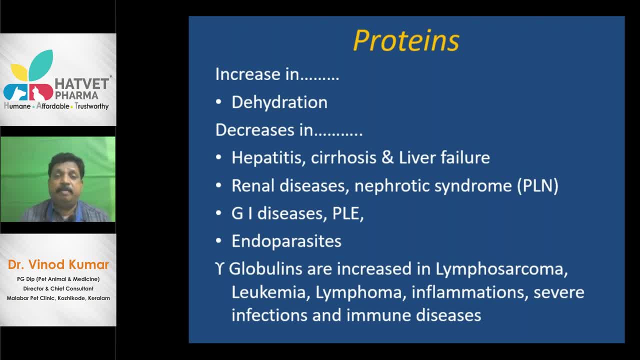 The pinworms, that is, trichuris vulpes, and the sestauts, the tapeworms. They are the three: diphyllidium caninum, diphyllobothrium latum and echinococcus granulosus. 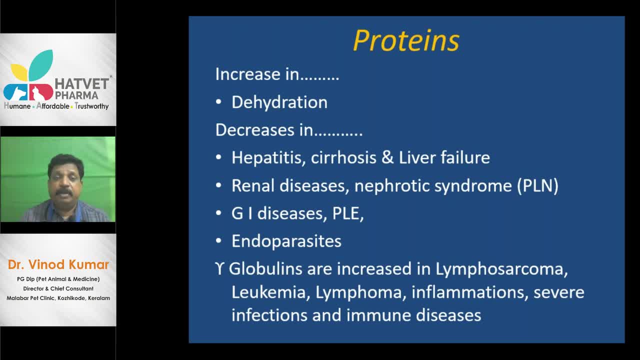 especially this diphyllidium caninum infestation Among sestauts. that is the most dangerous one, which produces severe protein loss. Dietary proteins will not be absorbed by the protein. Then hookworms. and coming to the globulin part, the gamma globulins are nothing but the immunoglobulins. 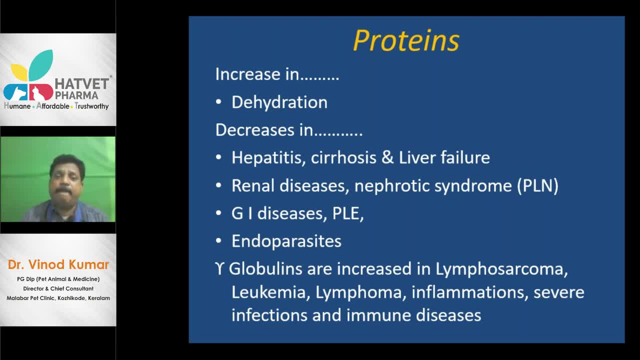 They are increased in malignant disorders. We have all these very commonly found malignant disorders, Hemopoietic disorders. We have all these very commonly found malignant disorders Such as lymphosarcoma, lymphoblastic and lymphocytic leukemia, lymphomas or malignant lymphomas, etc. 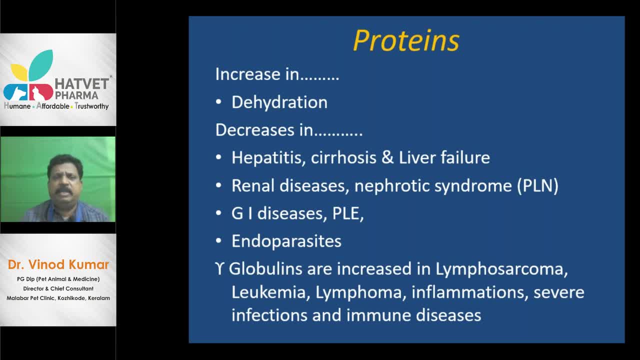 See, I have diagnosed all these conditions At least 8 or 9 times. I have diagnosed lymphosarcomas, leukemias, different two types of leukemias and lymphomas. In all these conditions gamma globulins will increase. Otherwise, in inflammations, severe infections and other immune diseases also, gamma globulins will increase. 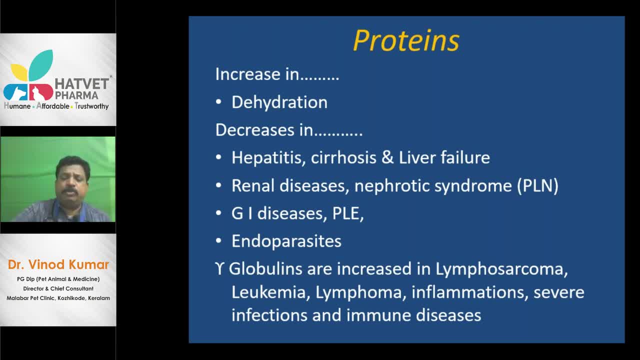 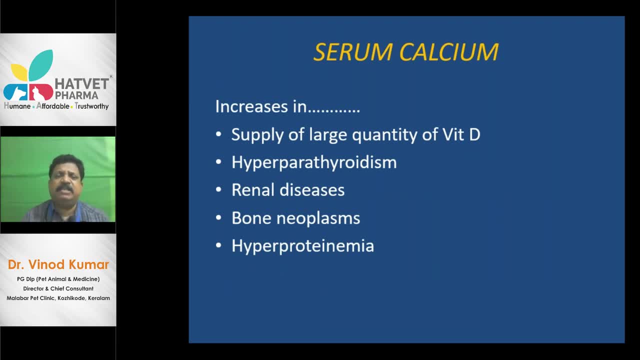 So that was something regarding the proteins. Now we are going to the next element: calcium. Increase in calcium is known as hypercalcemia. Decrease in calcium is known as hypocalcemia. Calcium is a minimalism in the body which has to do a lot of things. It is in the extracellular fluid and it is 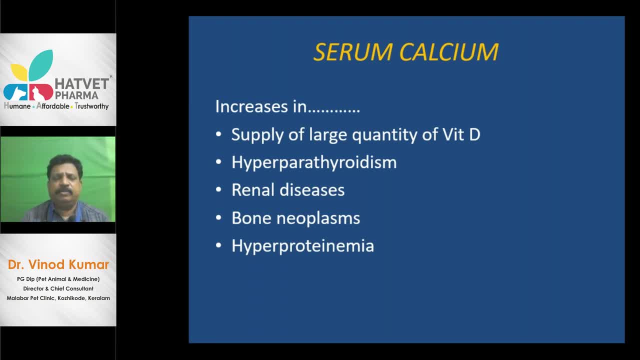 positively charged and this is increased, showing a condition known as hypercalcemia. In hypercalcemia, there will be increased calcium in the blood. Calcium is found in the blood either as protein bound calcium or as pre-ionic calcium As well. the body needs pre-ionic calcium for metabolism or for other body activities. the protein bound 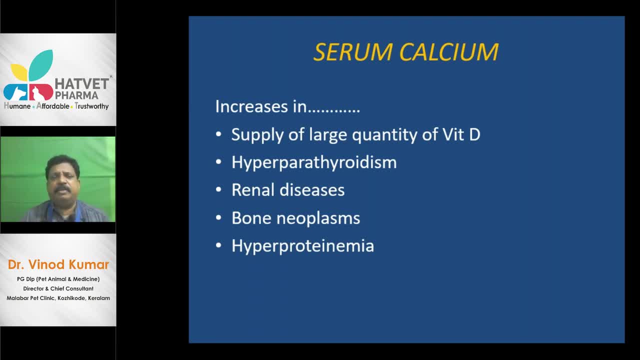 calcium will be released from the protein molecule and given to the system for assimilation As pre-ionic calcium, And the blood calcium increases in certain conditions, Of course. if you supply a large quantity of vitamin D, it can increase. Vitamin A, D, E, etc is. 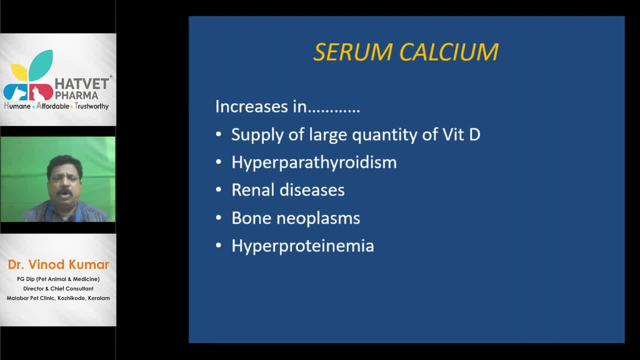 very commonly added to any oral feed supplement or a diet supplement for the dog. So it can be added to any diet supplement. So it can be added to any diet supplement for the dog. So it can be added to any diet supplement for the dog and the cat. So if you supply large quantity of vitamin D, that 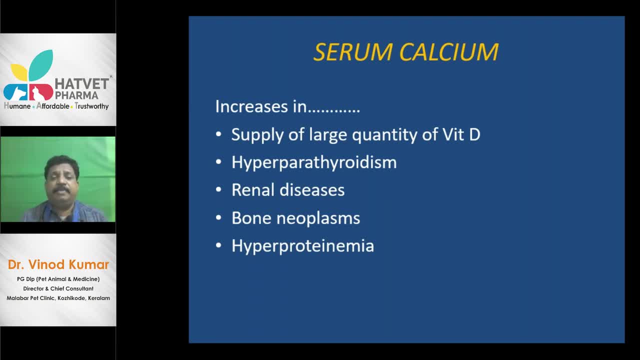 itself inside the gut can increase the absorption of calcium So that there will be a hypercalcemia. But mostly this hypercalcemia is transient or temporary, And this excess calcium will be excreted through the renal tubules, So also. number two is hyperparathyroidism. 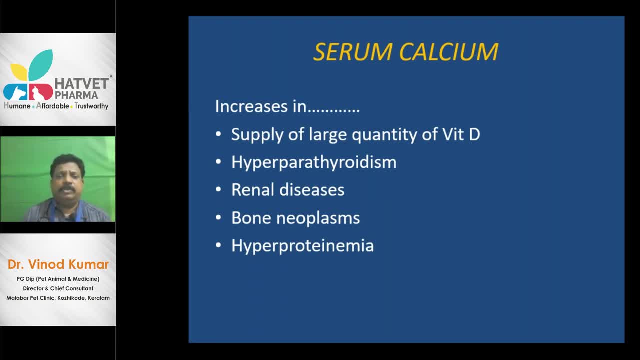 In hyperparathyroidism we have the parathyroid glands, For example. we know that this is all-meat syndrome. All-meat syndrome. It is very commonly found in dogs, especially in long-legged breeds such as the Dobermans, Great Danes, Tottweilers, Dalmatians, etc. In all these breed fast-growing. dogs in pups, the fast-growing pups In all these breed fast-growing dogs in pups, the fast-growing pups In all these breed fast-growing dogs in pups, the fast-growing pups In all these breed fast-growing dogs in pups, the fast-growing dogs in pups, the fast-growing. dogs in pups, the fast-growing pups. I will quote an example. When I was working in Trivandrum city, I went to a breeder's house. He was breeding all Dobermans only. he breeds Doberman only. 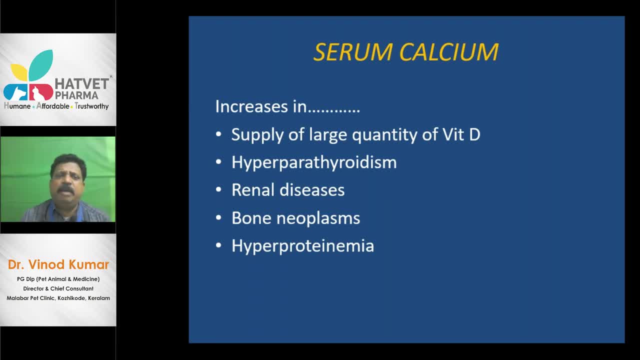 When I went there the client called me only because his new generation of all the pups have left again limb abnormality. Somebody mentioned that it is hip dysplasia and I was called there. I went there. I saw it was not hip dysplasia. Two, three, four months old pups- all are having. 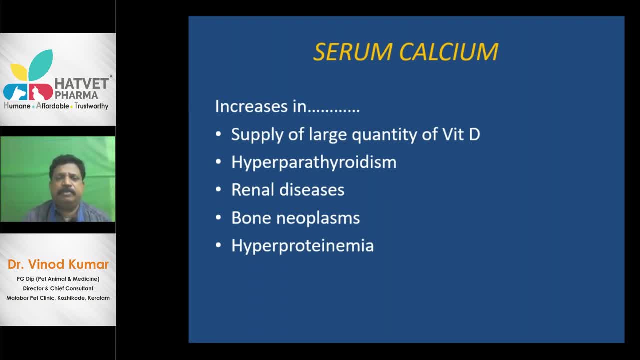 both limbs bracketed, both limbs. It was very easy for me to understand that this gentleman's brother owns a meat shop And in that meat shop he gets lot of meat- raw meat- And this raw meat was enormously expensive. So what happened? Meat contains practically no calcium, But it is rich in phosphorus. 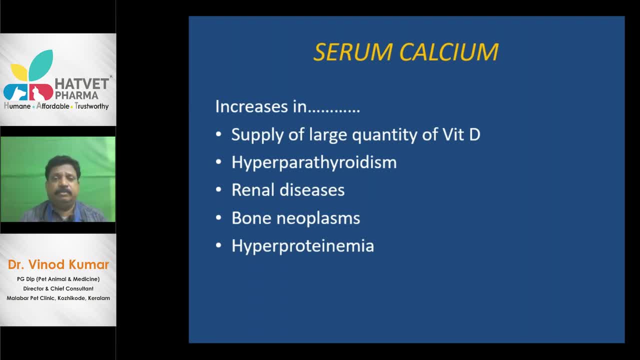 So hyperphosphatemia occurs. So what happens when there is a hyperphosphatemia? The homeostatic mechanism of the body has to maintain the normal serum calcium Phosphorus ratio. the blood calcium phosphorus ratio has to be maintained in a ratio of 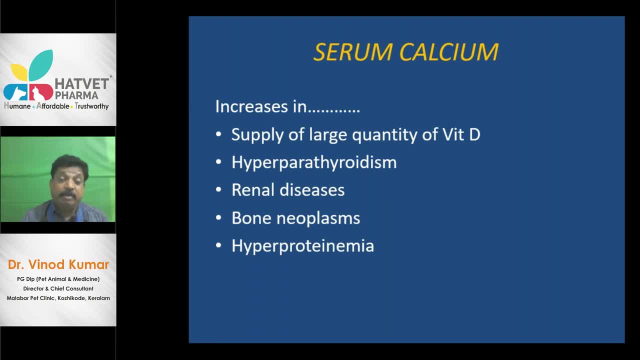 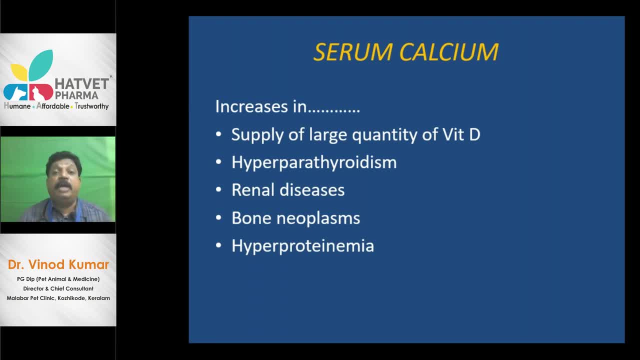 blood sugar And in this point the blood cell-richness has also reduced. That's the point, actually Very exciting. And he says the brain is going to show the book The natural Right central nervous system, which is that of the three octol, gradually. 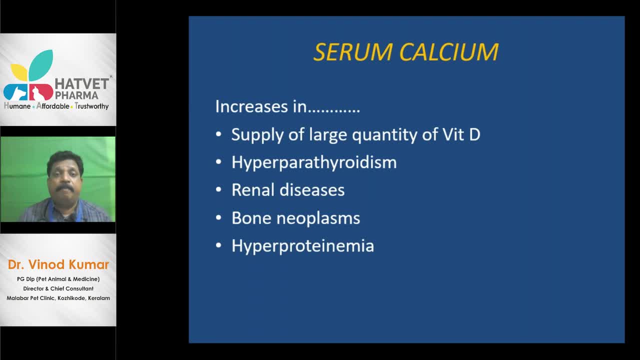 savails One, because naturally the brain grows numb. The brain turns it into a medical instrument and went through all of these physical urination mechanisms, andvoices and exercises and reintroductions. The parathyroid- Hello, Mr Parathyroid, Become active, Send some parathormone. So what will happen? The parathyroid gland becomes active and it will release some parathormone. What this parathormone will do, The body will sense it. What is the blood telling? There is no calcium. There is no calcium. Phosphorus has increased, like anything. 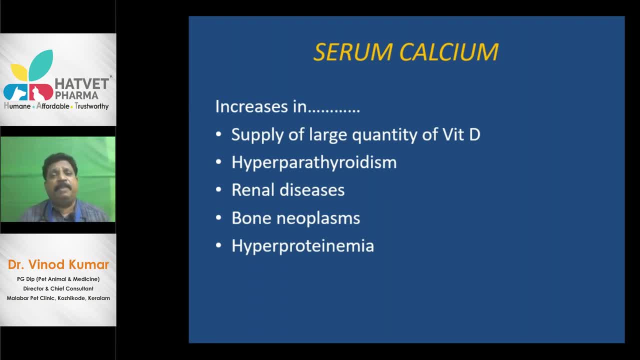 There is no. the dog is not at all eating any calcium. They are not giving any calcium, But the phosphorus is increasing like anything. Okay, the brain will sense it. There is no calcium. The puppy is not eating any calcium containing food. It is not being fed any calcium syrups or supplements, Nothing of that sort. But somehow the blood calcium phosphorus ratio has to be maintained. So what will it do? 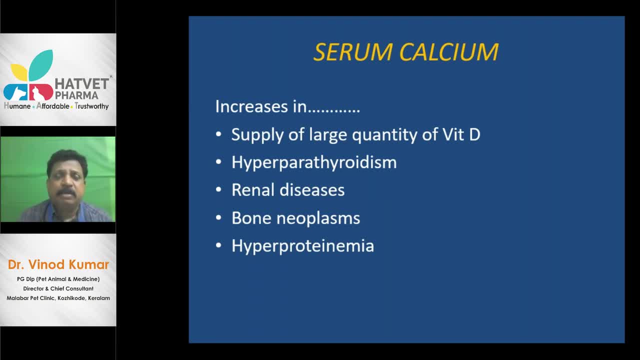 Then the blood will announce or order or command the parathyroid gland to produce or release some parathormone. It will be released and the parathormone will in turn mobilize calcium from the bone to the blood. So what will happen? There will be a hike in calcium. Initially there will be a hike and then it becomes normal. So we can see that there is a hike in calcium. 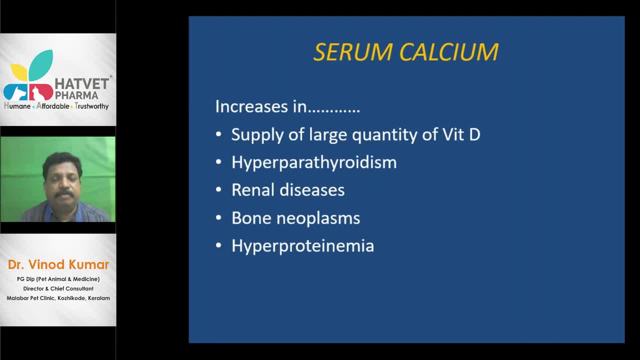 namely for聯, the blood producing hypocalcemia, hypercalcemia. here There is an increase in calcium in renal diseases. Calcium is excreted through the kidneys, We all know it, And so when there is a renal impairment, where there is oliguria, 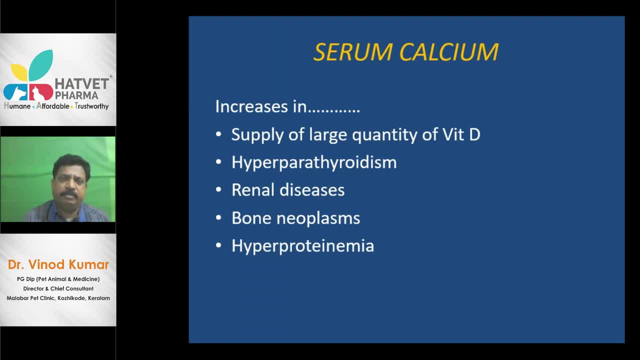 such as anuria or oliguric renal failure. there is accumulation of calcium in the blood producing hypercalcemia. It is ostensible In neoplasms of the bone. a very good example is osteogenic sarcoma. Severe osteosarcoma produces neobond formation- hypermineralization. 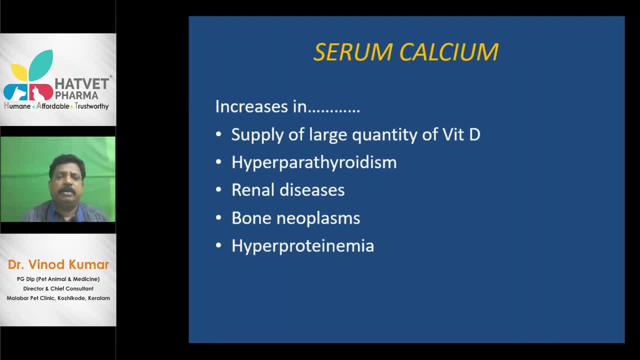 of the bone And for that there will be lysis of the bone and hypomineralization occurs And this calcium will be mobilized to the blood, producing hyperglycemia. That is osteogenic sarcoma. In osteogenic sarcoma, the radiographic finding itself is: 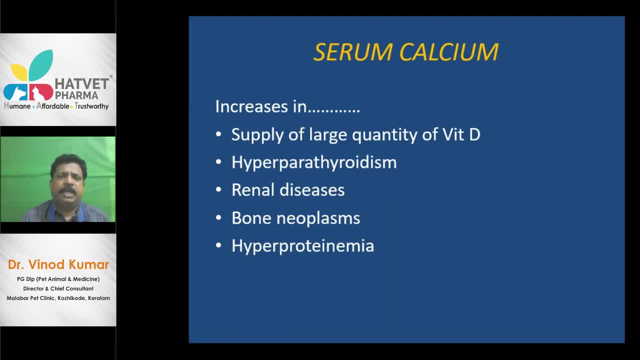 very important. It shows osteolytic reactions. It shows a sunburned osteolytic appearance Where, Where, Where In the mane, The blood is being rich with calcium which is being mobilized from the bone. Then another cause of hyperglycemia is hyperproteinemia. When there is increased protein, the chance 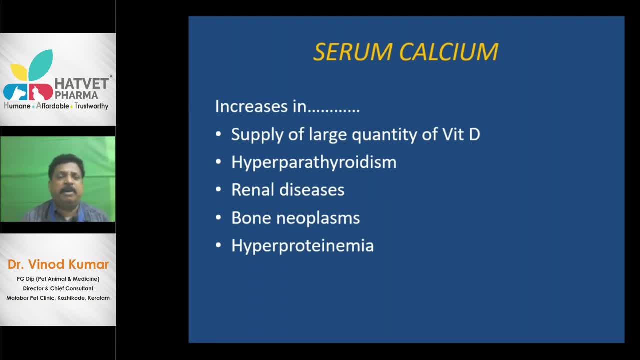 is very low When there is increased protein in the blood. this is also a good thing. It These proteins are attached to the calcium, as I said, a protein bound calcium. As I said, there are two types of calcium: the protein bound calcium and the free ionic. 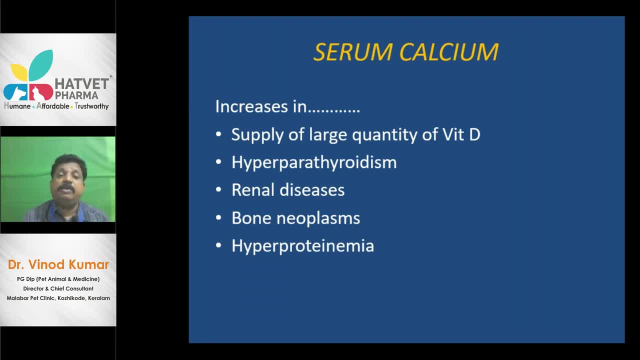 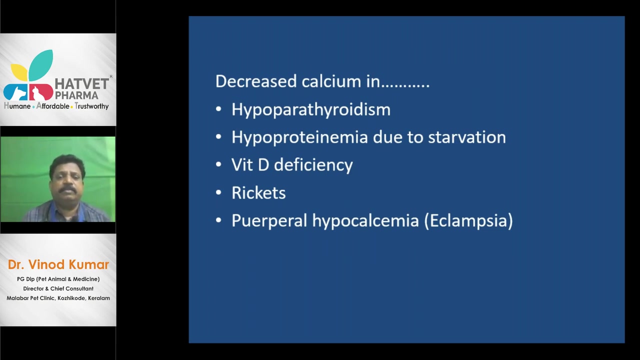 calcium And the protein bound calcium will also increase when there is high amount of protein. it will be attached to too many molecules of calcium and so there will be natural there will be hypercalcium. here got it. Then sometimes calcium becomes less. 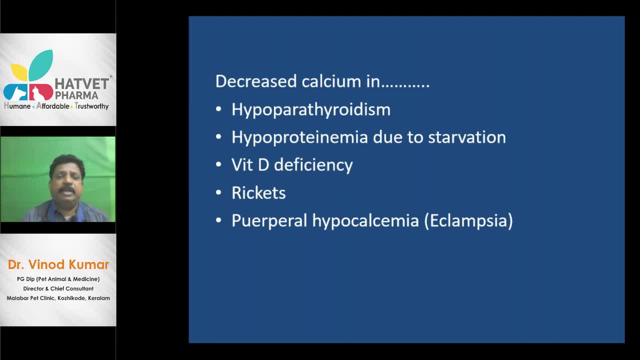 We have seen that blood calcium increases in hyperparathyroidism. But what about in hypoparathyroidism? Hypoparathyroidism is extremely uncommon. It is common in dogs, but it is a cause for hypocalcemia. 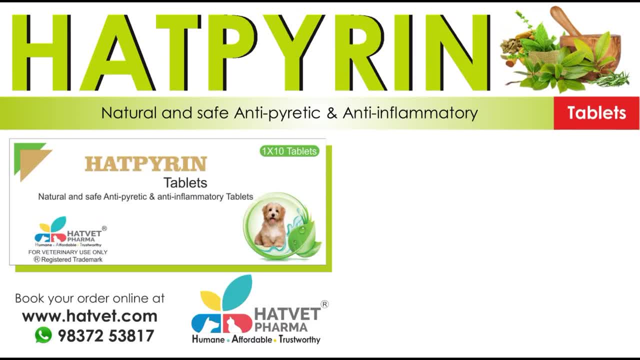 So we have seen in the past that some people have hypoparathyroidism, But in this case it is common. How many types of calcium is there in the protein? 1. Type 2. Type 3. Type 4.. 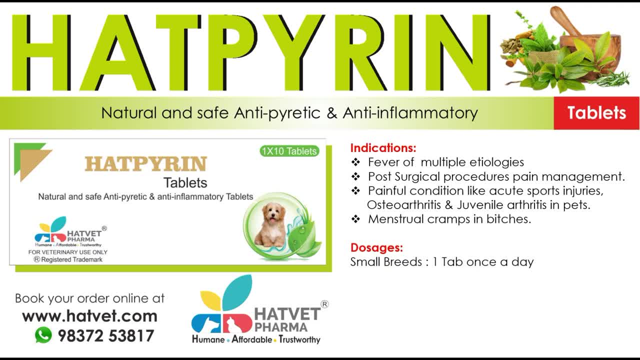 Type 5. Type 6. Type 7. Type 8. Type 9. Type 10. two tablet once a day for cats. half to one tablet once a day. root oral presentation 1 into 10 tablets. you can book your order online at wwwhatwoodcom. 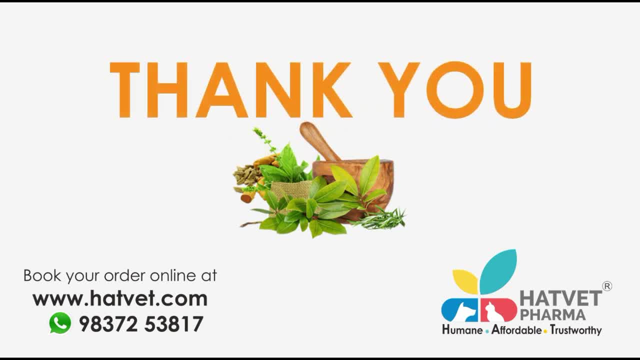 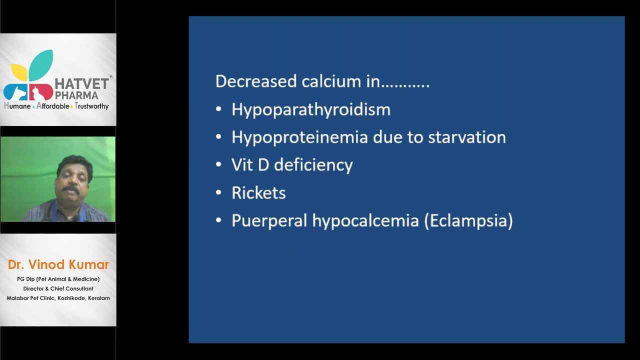 looking forward to a long-lasting business association, thank you. then in starvation there will be a hyper proteinemia wearing. the protein molecules are not sufficient to be having and impair the pair of the bearing with calcium ions, and so it protein bound calcium cannot be established, producing hypocalcemia that is. 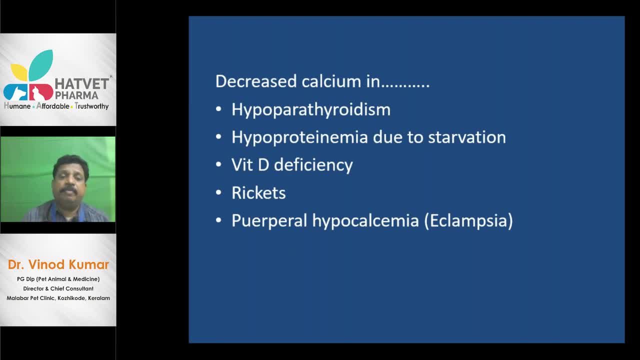 hypocalcemia. hypocalcemia due to hypoproteemia, which is due to starvation. there is vitamin D deficiency. yes, absurdly. vitamin D is necessary for the dietary absorption of calcium from the intestine. if it is deficient, the calcium will be lost through the feces and absorbed. so a hypocalcemia. 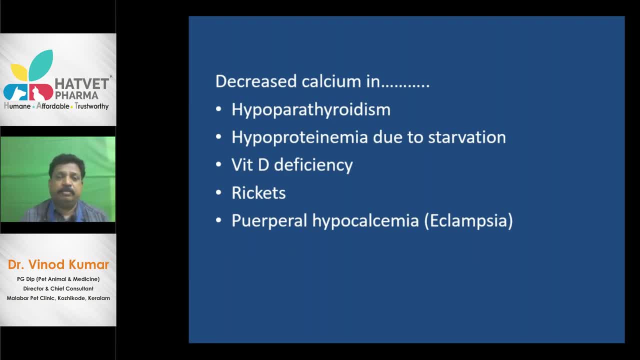 occurs then in rickets? we all know there is rickets, rickets, even what happens, why there is bowing of legs and rickets, especially when I said I explained, regarding the nutritional hyperparathyroidism, why there is a bowing leg. it is a growing pup. it has been fed with large amounts of meat which contains or which 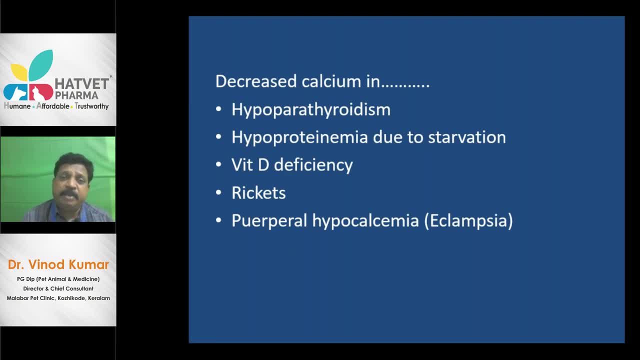 is rich in phosphorus. hyperphosphatemia induces hyperparathyroidism. okay, in hyperparathyroidism, what happened? there was rickets, rickets, rickets, rickets, rickets. what is happening? there is hypo mineralization of the bones, that is, the bone density decreases. 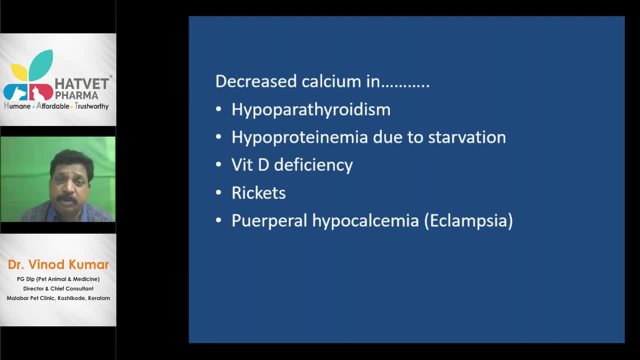 bone becomes more soft and brittle. the condition is known as osteomalacia. osteomalacia due to osteomalacia, it is a growing bone. it is long bone, like the radius ulna etc. especially the forelimbs, the pectoral limbs. there is more weight on the pectoral limb than the pelvic limb. the pectoral limb means 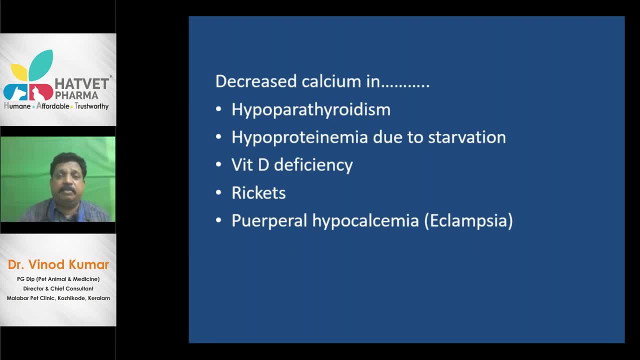 anterior limb, that is forelimbs. it is a expensive limb. in the pectoral limb the weight of the head, neck, thorax, etc. part of the abdomen also will become. but the hind limbs, that is pelvic limb, carries only the weight of the hind quarters plus the tail, that is all, and the pectoral. 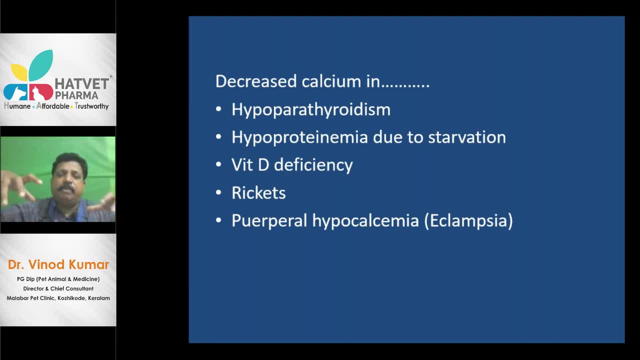 limb is more important. So the complete weight of the body will be on the pectoral limbs. and what happens to radius and ulna? It will undergo bowing bending. so due to the weight, it will bend. That is the reason for bending of the forelimbs only. 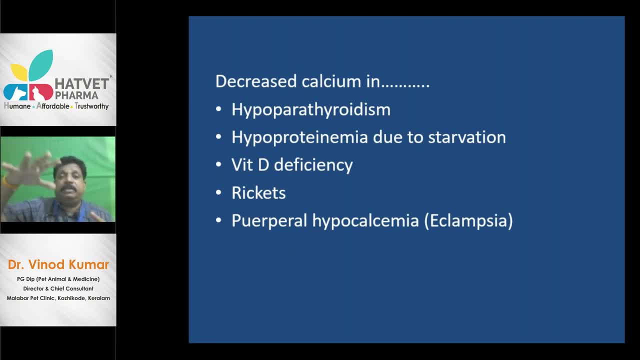 And also what happens to the rib cage. There is weight over the rib cage because everything is putting their weight on the sternum Through the ribs. it is putting the weight on the sternum, So sternum is joining the rib, is joining the costal cartilage. 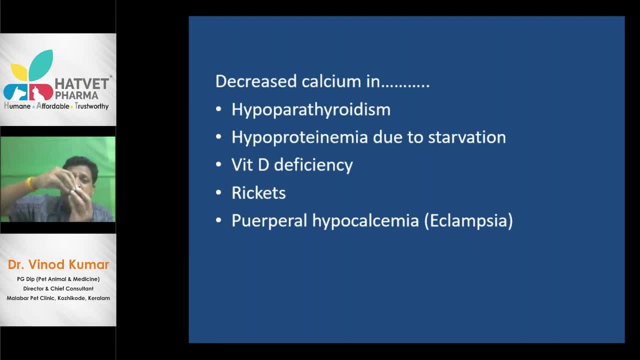 So it is joining and at this joint the body weight will come and there will be enlargement of the costal chondral junction and the costal chondral junction will swell up. That we can palpate. That we can palpate as a bead. 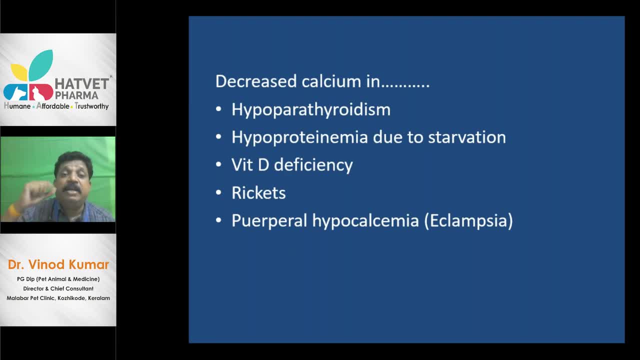 That we call it as racquetic rosaries. So that is why we say racquetic rosaries- and arching or bowing of the forelimbs. This is the reason, for only forelimbs is affected. So there is another question: will not the hind limbs are affected? 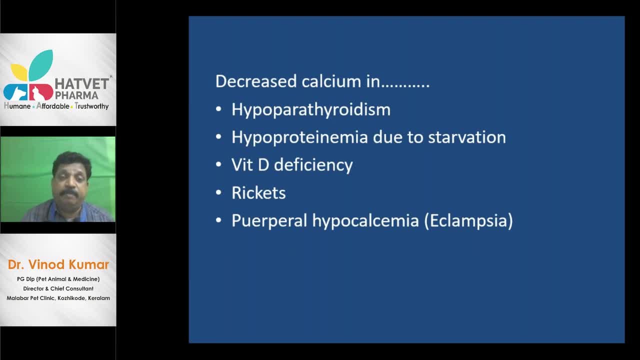 Yes, the hind limbs can be affected, especially the acetabulum. It shows an acquired dysplasia of the hip, Sometimes show painful bones of the hind limbs, Sometimes show shivering of the hind limbs. So these are the clinical signs shown. 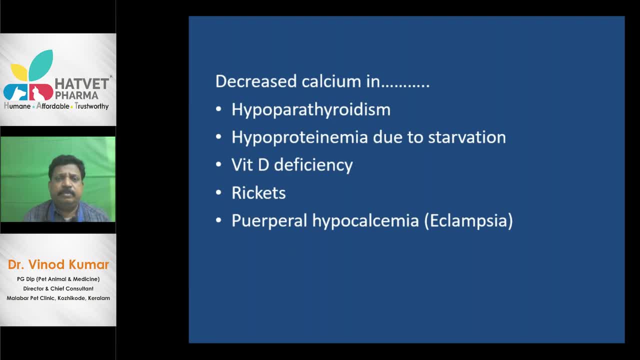 That is in rickets, Then in peripheral eclampsia. Yes, Yes, Yes, Yes, Yes, We all have encountered. I myself have encountered several times. We have in the cow post departure and hypo-calcemia. All the eminent doctors in our webinar knows very well, especially the mixer practitioners. 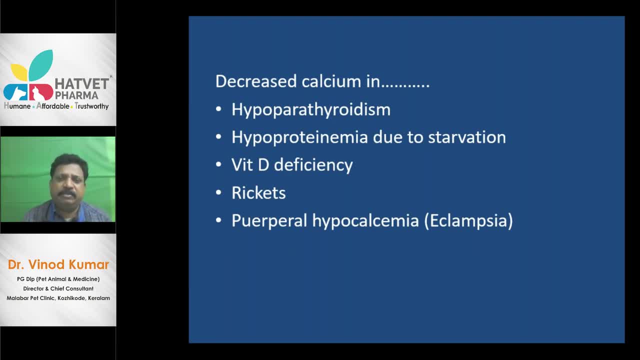 Large animal medicine is a very good medical science. of course, most of our doctors are mixer practitioners and we all know about post-departure in hypocalcemia. it is due to excessive drainage of calcium from the body and produces at the pathognomonic symptom. 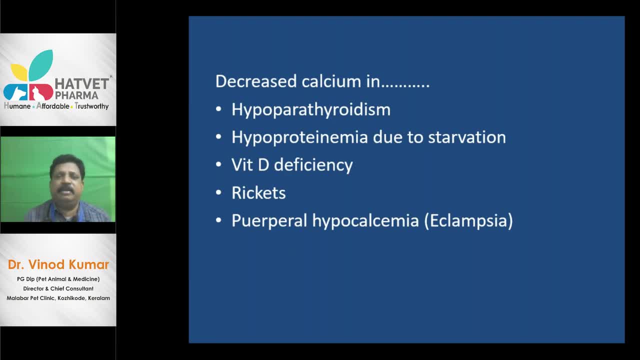 like thinking of the head looking at the flank, placing the head on the flank- is that the only symptom in the cow? know that there is a stage of excitation before that. then there is a stage of sternal recumbency, then there is a stage of. 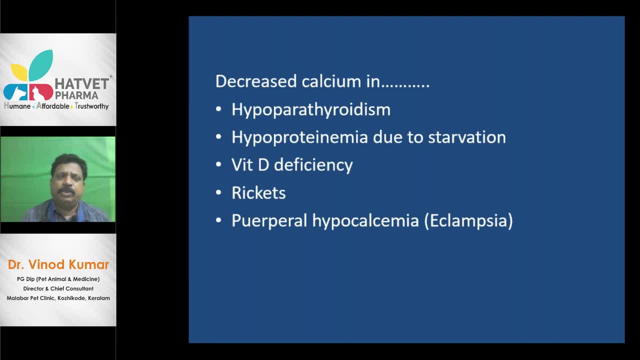 tinging of the head. so in the cow the ultimate or the presented symptom is a paralytic syndrome, paralytic symptom, but in the dog it is a form of paralysis. but in the dog it is a form of paralysis. It is not like that Calcium deficiency, like this after post whelping syndrome in pets. in dogs it produces excitatory symptoms and this excitatory symptom is known as a Clampsia. 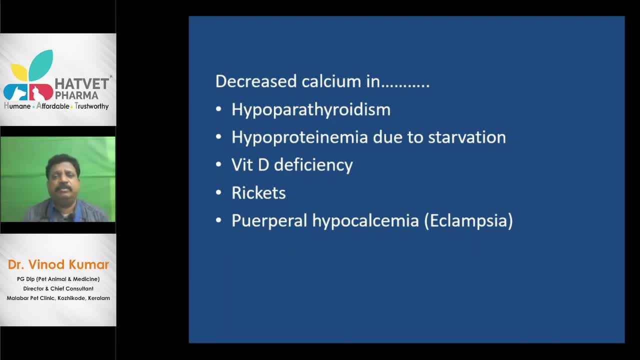 The clinical finding is it produces convulsions, shivering, hyperthermia etc. When there is shivering and convulsions, definitely there will be hyperthermia. So it is very easy to find it out. If the dog has whelped recently, there itself is a clue that it is hypocalcemia. 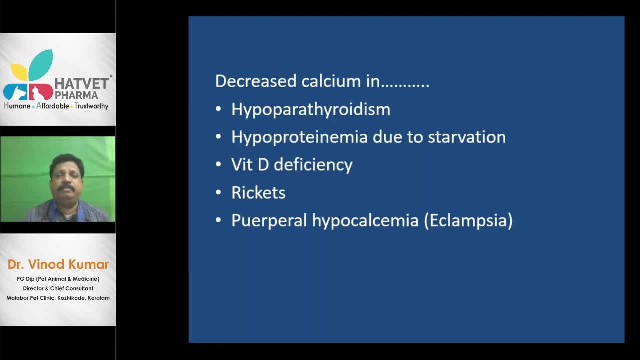 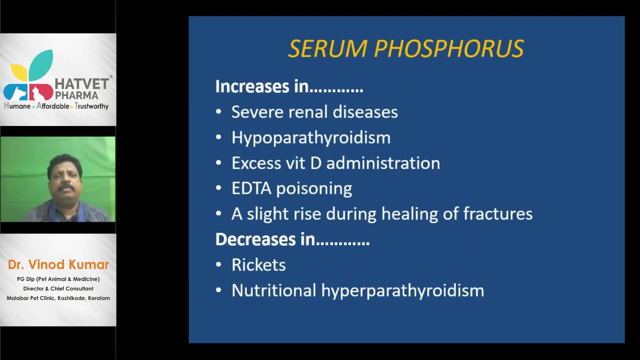 It is hypocalcemic tetany or hypocalcemic eclampsia or peripheral eclampsia in the beach. Then we are coming to blood phosphorus. Increase in phosphorus is hyperphosphatemia and decrease in phosphorus is hypophosphatemia. 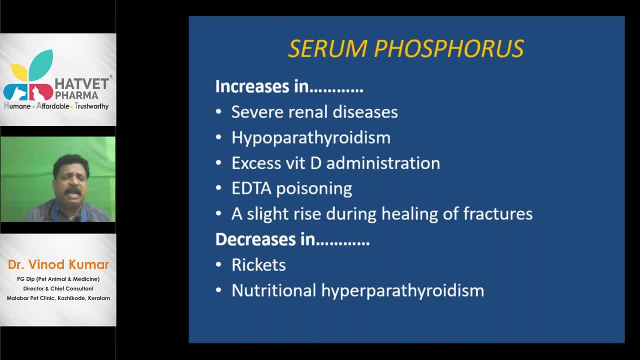 It is almost the same. It is almost the same Same to calcium, because calcium and phosphorus are almost seen as a pair, especially in the bone and teeth. The phosphorus is also excreted through the kidneys and that is why in a chronic renal failure there is hyperphosphatemia. 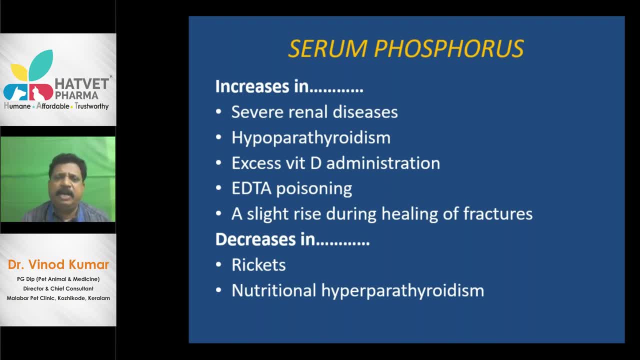 Very recently also, I got a case like that. In chronic kidney diseases hyperphosphatemia occurs and this hyperphosphatemia itself can induce hyperparathyroidism. It produces mobilization of calcium from the bone to the blood so that the bones become brittle and osteoma issue occurs. 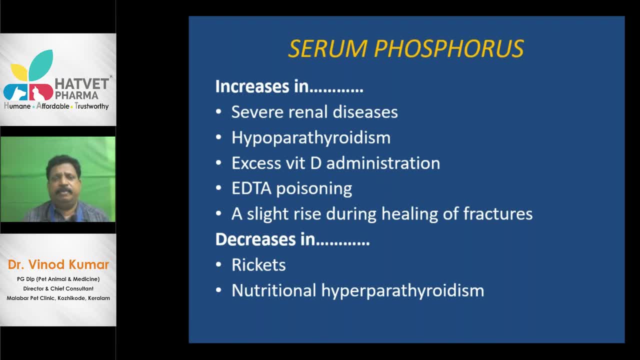 Especially in the cat, such osteoma issue occurs and there will be demineralization or hypomineralization of the jaw bones, that is, the mandibles, And the mandibles will become so rubbery and you can just simply twist the mandibular bone. 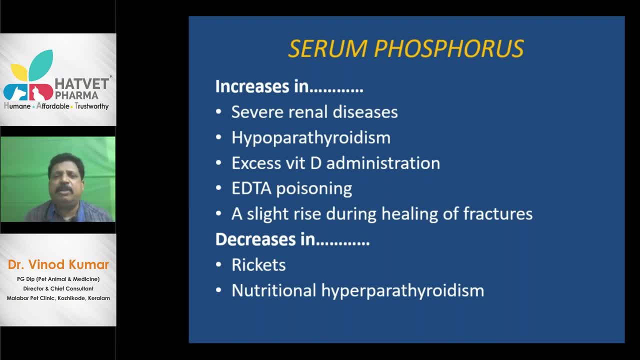 You can simply pull out the teeth of the mandible. The mandibular teeth can be pulled out. It will be shaking and it will be moving, So mandible will be having osteomalacia. It is known as a rubber jaw syndrome. 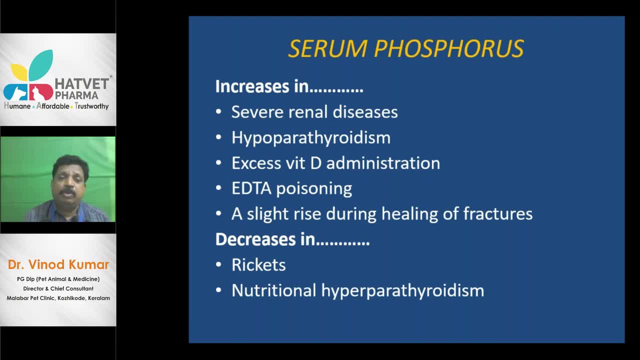 So hyperphosphatemia occurs in chronic kidney disease And hyperphosphatemia occurs in hypoparathyroidism. Of course it is ostensible. You see, high phosphorus induces hypoparathyroidism And hypoparathyroidism induces high phosphorus. 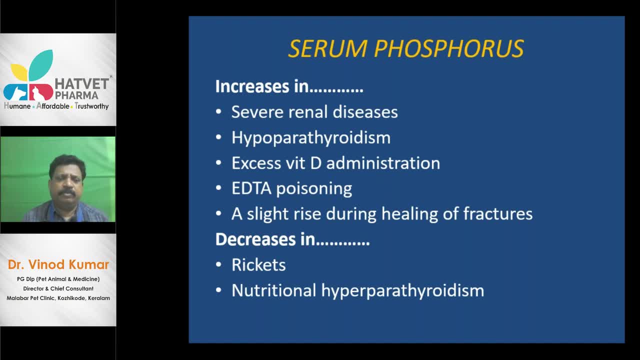 It is ostensible. Then excess vitamin D administration In order to maintain the calcium phosphorus ratio. The calcium increases and also phosphorus increases, And so there is hyperphosphatemia. Then we know about EDTA- EDTA poisoning. 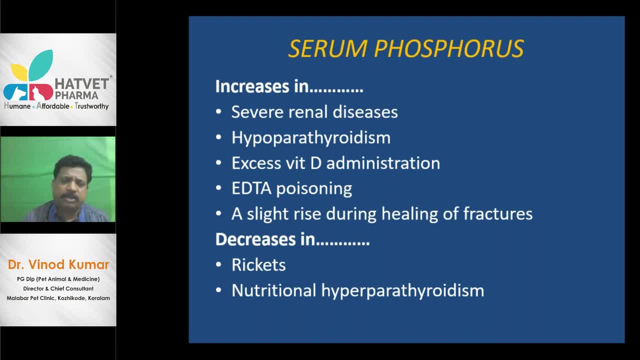 As in textbooks. it is not so common in dogs, But it is written First. when I was preparing this slide, I was really wondering whether to include this or not. Ultimately, I included it, And so when there is EDTA poisoning, 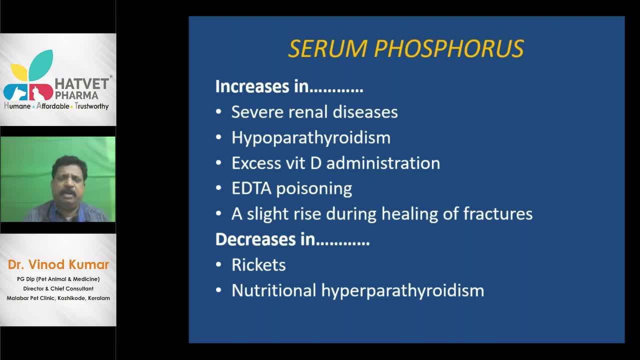 EDTA comes to the system, It will chelate the free ionic calcium. So what will happen? There will be a hypocalcemia. When there is a hypocalcemia, There is more need of calcium, And so there will be hyperparathyroidism. 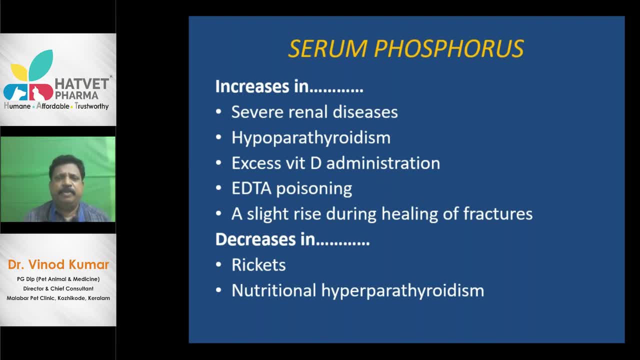 Which in turn mobilizes calcium from the bone. Along with that, phosphorus also will be mobilized, And so a hyperphosphatemia occurs in EDTA poisoning. Then there will be a slight temporary rise of blood phosphorus during healing of fractures. 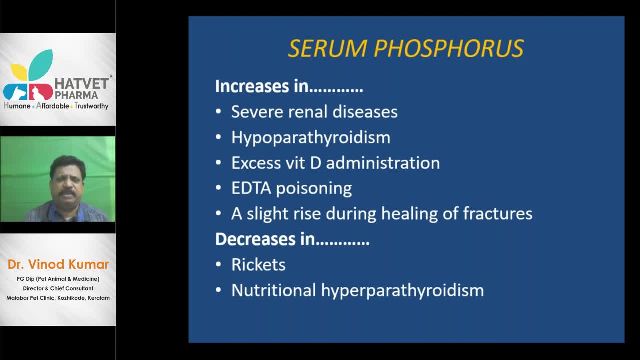 Highly substantial Because bone is made up of calcium and phosphorus, So it is needed, And phosphorus decreases, in RIG case, Highly substantial. All these are related with bones, Because the bones are made up of calcium and phosphorus. 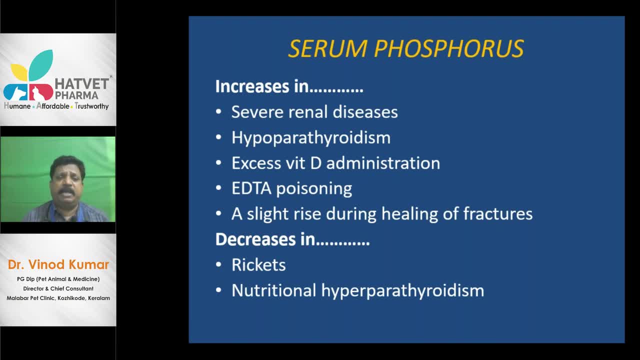 Then in nutritional hyperparathyroidism It decreases Because there will be enough calcium will be mobilized And the serum calcium phosphorus ratio then will be maintained, Reducing the serum or the blood phosphorus level, And chief excretion of phosphorus is through the urine. 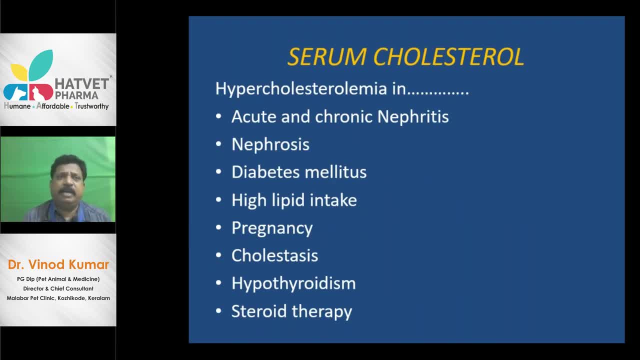 Then We have to study something about serum cholesterol. When I went to Imphal Manipur To take a session After the session, After the seminar, The doctor there had already advised his clients To bring all their pets Because a popular doctor from Kerala has arrived. 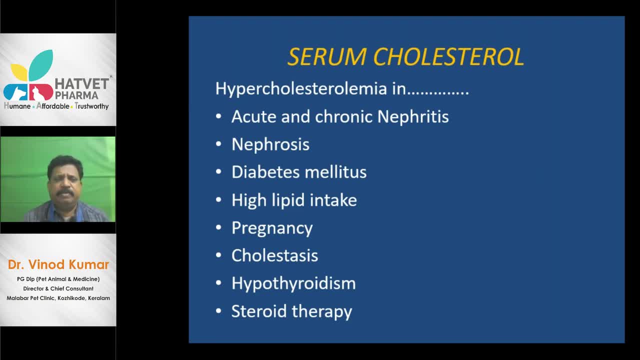 He made a system like that And lot of pets were presented there With different, especially skin lesions. I was going through all those skin lesions And a human doctor with MD general medicine came there. He asked me regarding giving egg to his pet. 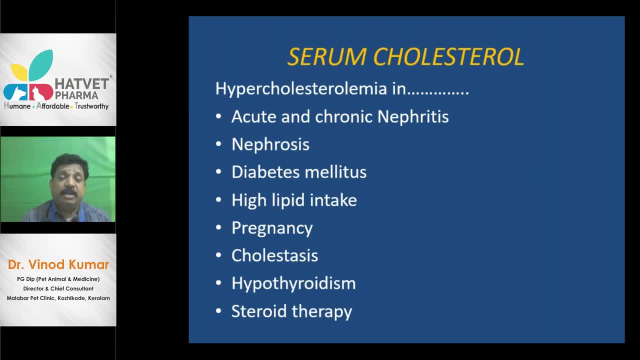 He said he is afraid to give more than half an egg a day. Why? Because he is worried about cholesterol. I said nothing to worry. It is not like in human beings. There is no hypercholesterolemia, Especially dietary hypercholesterolemia, in dogs. 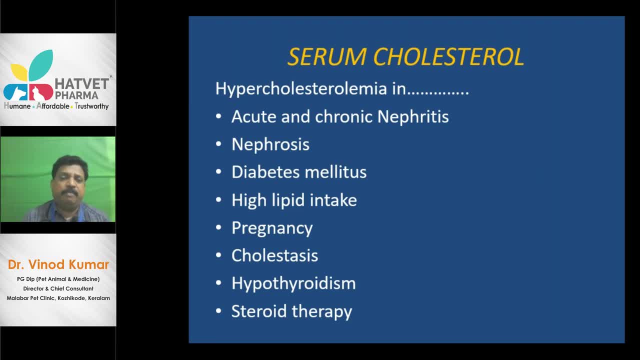 Nothing will happen. You can give lot of eggs a day. He was wondering: Will the cholesterol not increase? I said no, Cholesterol increases in the blood Due to these factors. In acute and chronic nephritis, Hypercholesterolemia occurs. 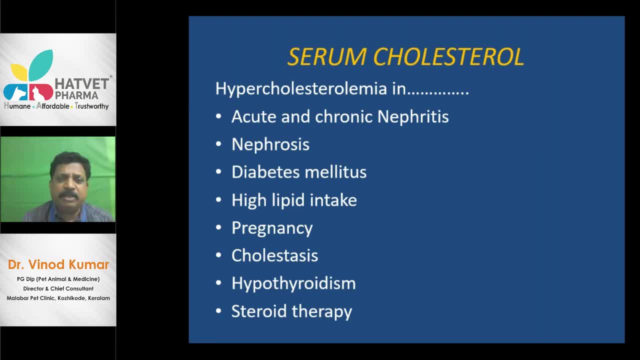 See, it is a rule, Because cholesterol excess is being eliminated or excreted through the urine Filtered through the kidney, And so when there is an oliguric renal failure, There is hypercholesterolemia, So also nephrosis. 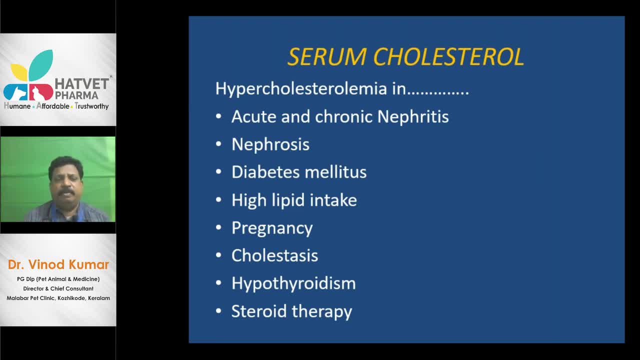 The same can be attributed: If there is oliguria in nephrosis, There will be hypercholesterolemia, Diabetes mellitus. Of course, The excess sugar in diabetes mellitus Will be converted to cholesterol And hypercholesterolemia occurs. 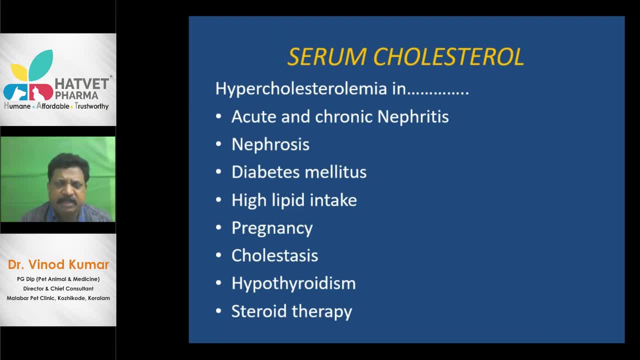 That is why People with diabetes mellitus Have high cholesterol levels. But human hypercholesterolemia And canine hypercholesterolemia Are entirely different. The low density lipoproteins of Human cholesterol Can segregate. 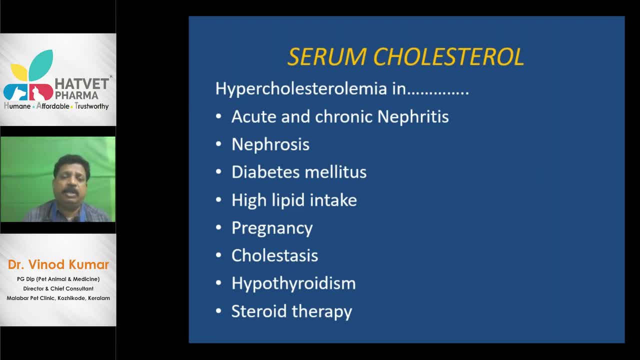 And deposit Onto the Interiors of the Wall of Arteries and arterioles And can produce Arteriosclerosis Or atheromatous plagues, Atherosclerosis And Complete obliteration of the 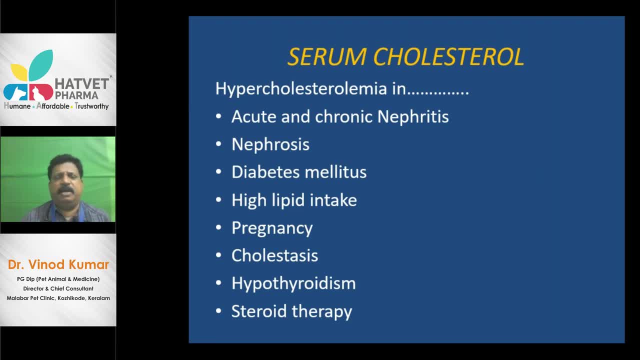 Vessels producing End ischemia. That can lead to Myocardial ischemia Or ischemia anywhere, Especially Myocardial ischemia, But there is no such Case in the Dog And for the human beings. 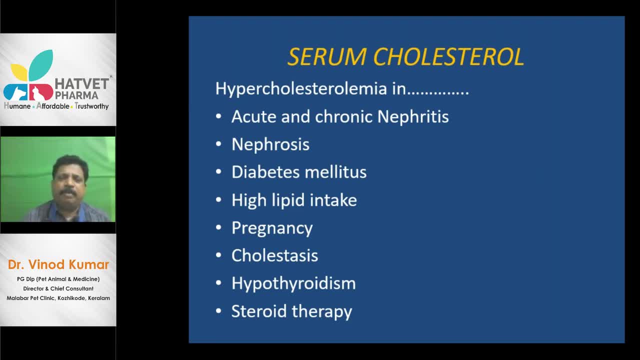 They used to give For preventing this segregation. They used to give Anti-segregating drugs such as Clopidogrel, But there is no such case in the dog. Need not give it. So High cholesterol is seen In nephrosis. 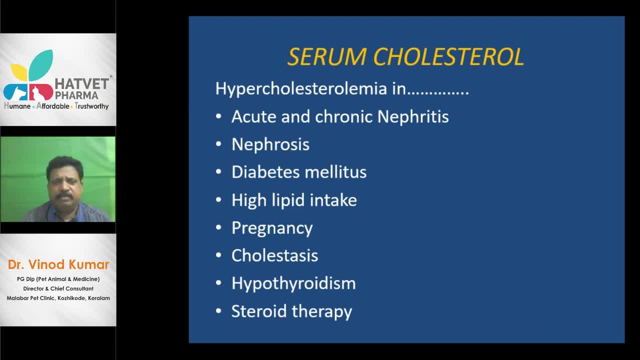 In diabetes mellitus. The thing is that Cholesterol Almost 80% is being Synthesized in the liver. Dietary cholesterol is Coming around only 20%. We need not worry about Dietary cholesterol, Especially in human beings also. 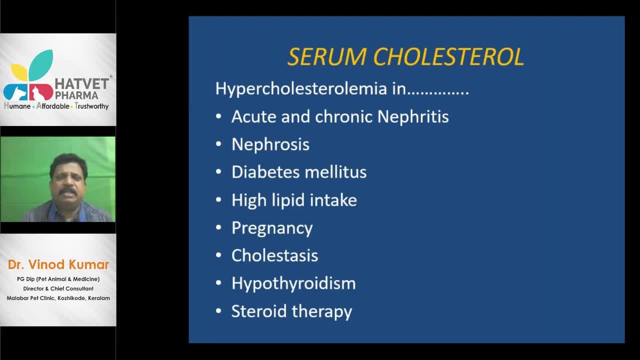 The Statin companies Make this hell of problems. These companies are Dispensing The atorvastatin, Simvastatin, Etc. They have a Crores and millions and millions of Business For their business. 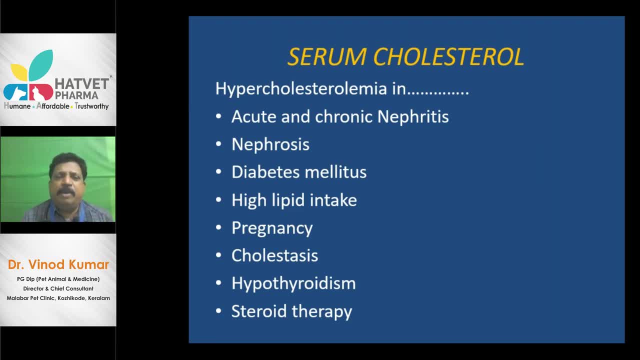 They always say that The normal cholesterol level Could be Inside 200. And they always Frighten the people Who is having 220. Or 230 cholesterol that, Oh, this is very big, Is very much, Is very high. 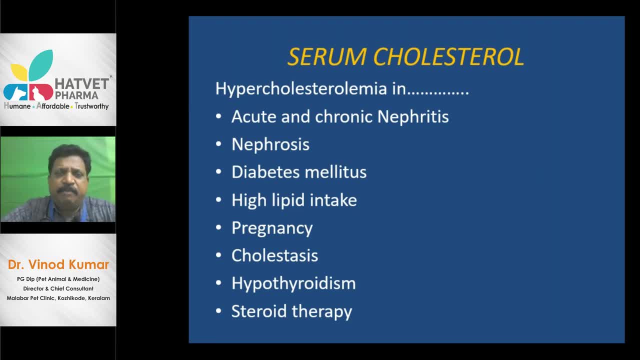 And you will get strong Or atherosclerosis Or myocardial infarction, Will be died all of a sudden. No, nothing will happen. Cholesterolemia: Cholesterole is being synthesized And utilized in the body. 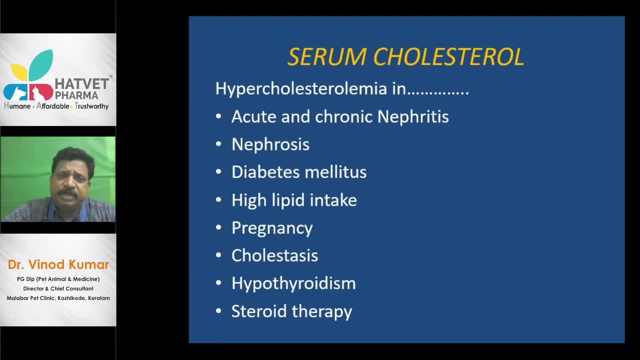 Of course, for all our activities, Especially for the brain functions, Cholesterole is needed. For all Production of all the types of hormones, Other complex proteins In the body, Cholesterole is needed. And even if Dietary cholesterol is nothing, 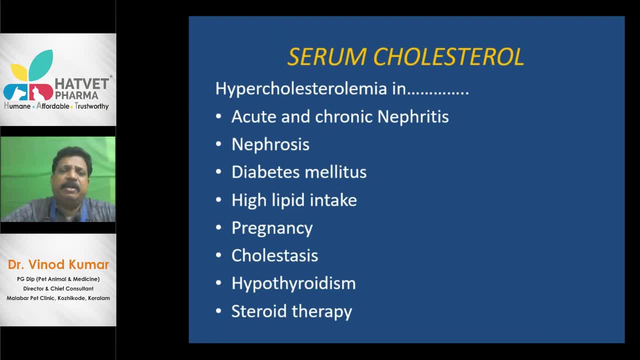 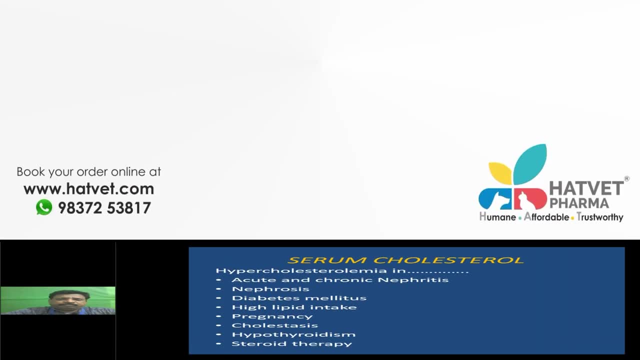 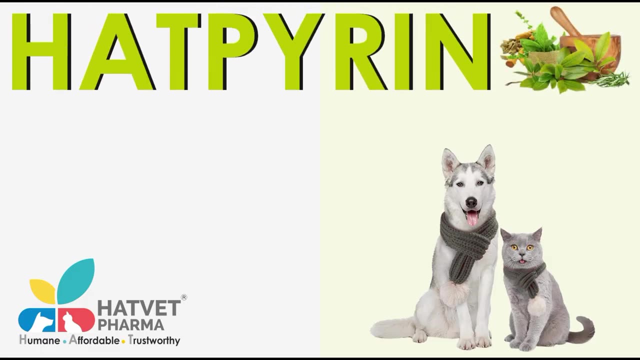 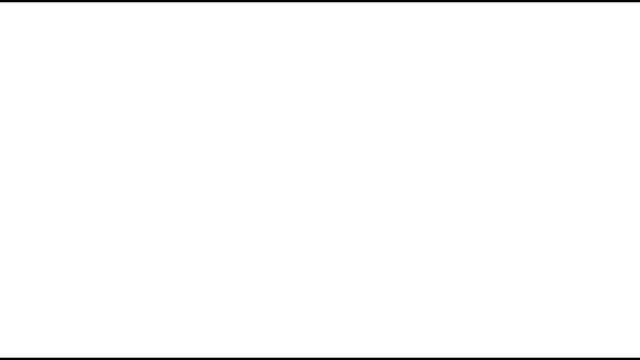 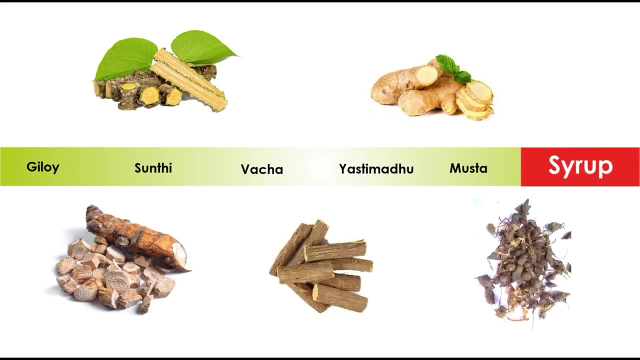 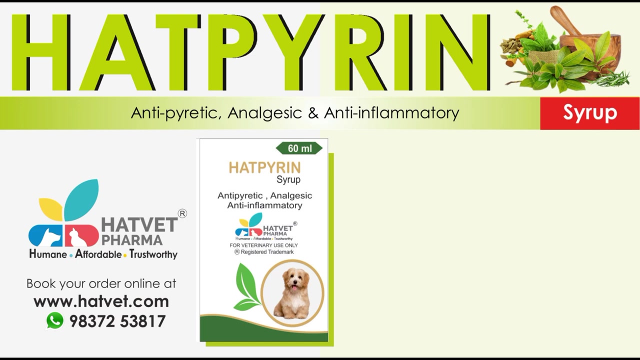 Everything is being Synthesized in the liver For the normal body activities, Then why should we worry about it? Cholesterole is used. It's for the overall health And the main Why it is being It is Cholesterole is used. 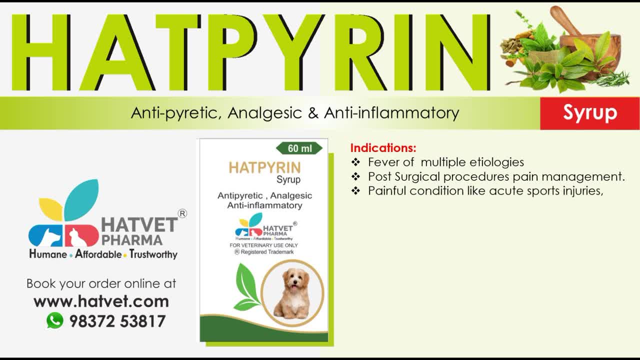 For the Diabetes An anti inflammatory syrup. Had pyran syrup. Indications: Fever of multiple etiologies, Post surgical procedures, pain management. Painful condition like Acute sports injuries. For large breeds, 2 to 4 ml twice a day. 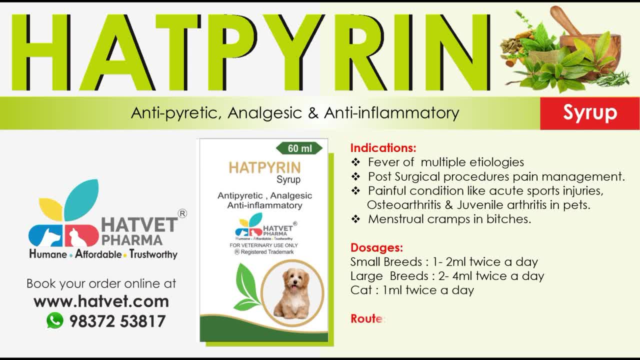 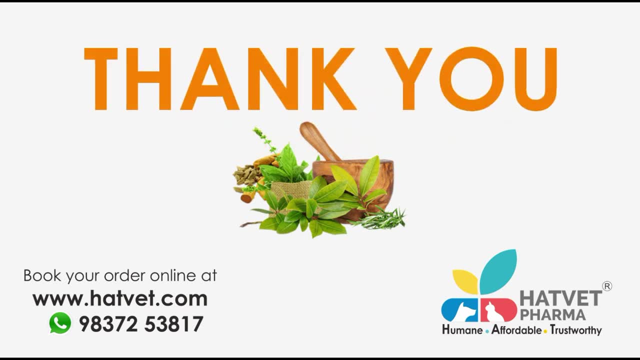 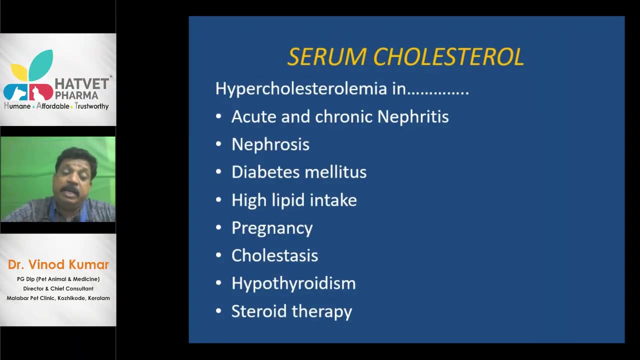 For cats: 1 ml twice a day. Root oral Presentation: 60 ml. You can book your order online at wwwhatwitcom, Looking forward to a long lasting business association. Thank you. Of course, high lipid intake will produce a transient or a temporary hypercholesterolemia. 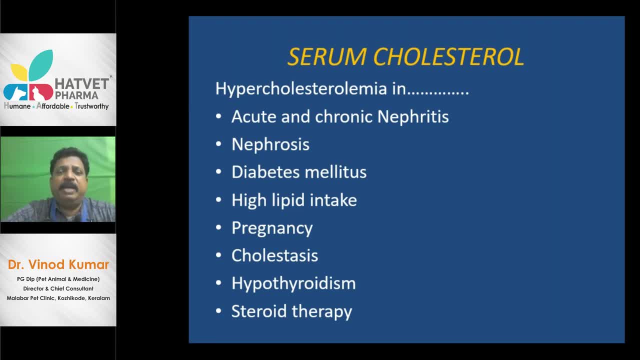 See, after a lipid heavy, fatty diet, heavy lipid rich diet, you take the serum triglycerides, it will be very high. Then in pregnancy, In pregnancy it is Necessary, it is mandatory. That See, it is not only the mother. 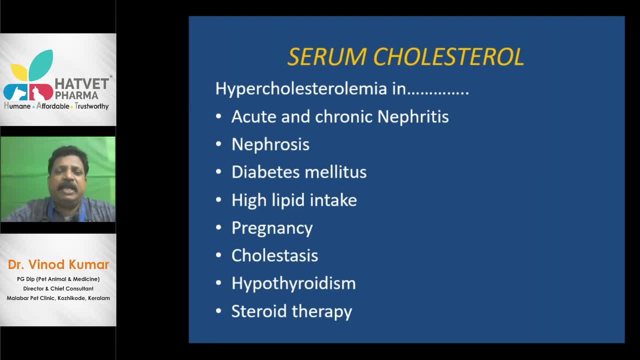 There is a baby growing inside, Whether it is a canine baby or the feline baby or the pig baby Baby is growing inside. the fetus is growing As for the development of their natto cord, development of the nervous system. 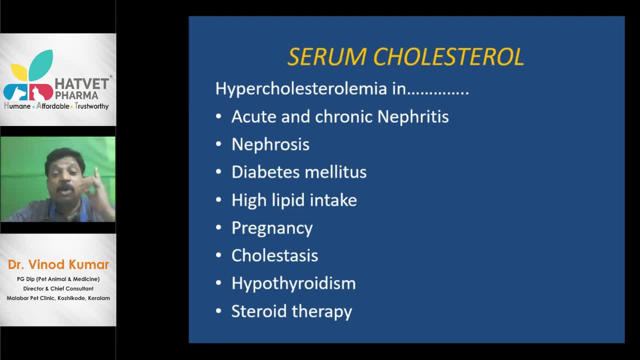 cholesterol is needed. So what the God has given, God is a good engineer, The greatest engineer. Progesterone is always needed for cholesterol synthesis, And so we all know that during pregnancy, a corpus luteum is being maintained. 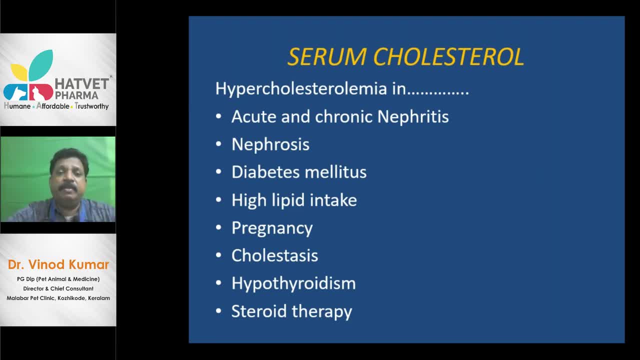 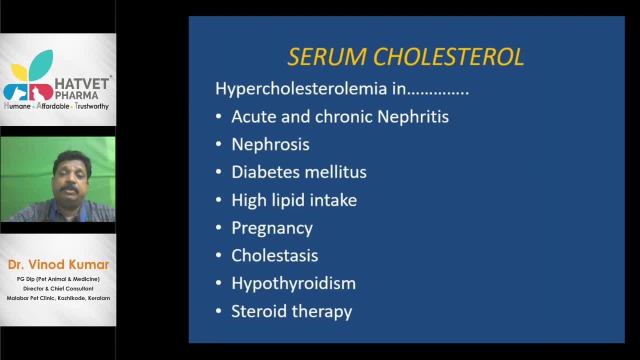 And this corpus luteum releases progesterone, always for the maintenance of pregnancy, produce an early fetal expulsion. So that is under the glute. So during pregnancy the corpus luteum produces progesterone and the progesterone is needed for the progesterone. 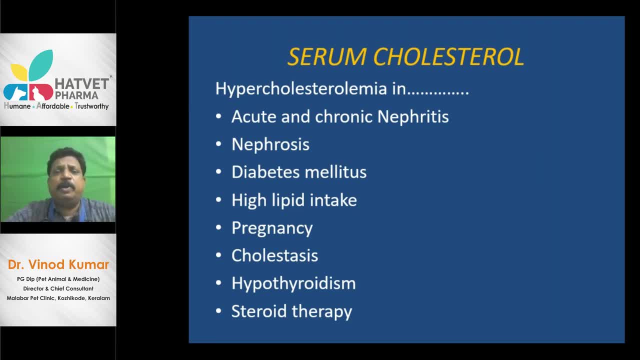 itself will produce, induces the liver to produce more amount of cholesterol and there will be a transient hyperglycemia till welping Then in cholestasis. why in cholestasis there is hypercholesterolemia? It is so simple: Cholesterol is being synthesized in the liver. 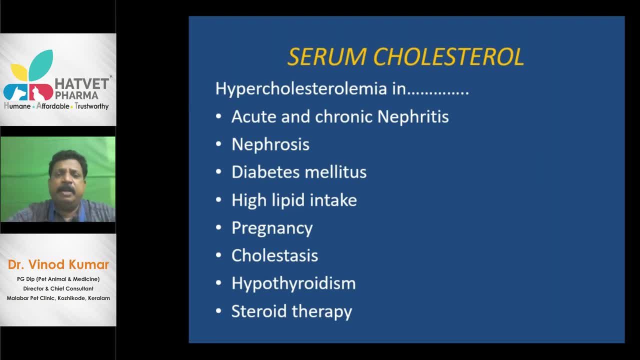 In the liver there is a small type of primary activation, but it has to be activated inside the duodenum for a menstruation Major or a secondary activation. For that this cholesterol will be mixed with the bile and excreted into the duodenum via the bile duct. So if there is a bile duct obstruction, 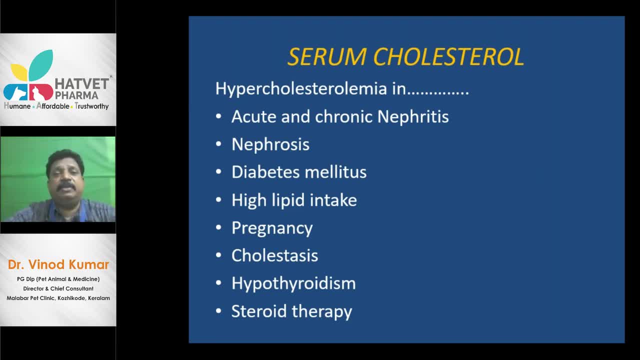 like a cholestasis, like a stone inside the bile duct or a tumor inside the bile duct. what will happen? There is cholestasis and the inactivated cholesterol will be inactivated. Cholesterol is being reabsorbed due to stasis and hypercholesterolemia occurs. 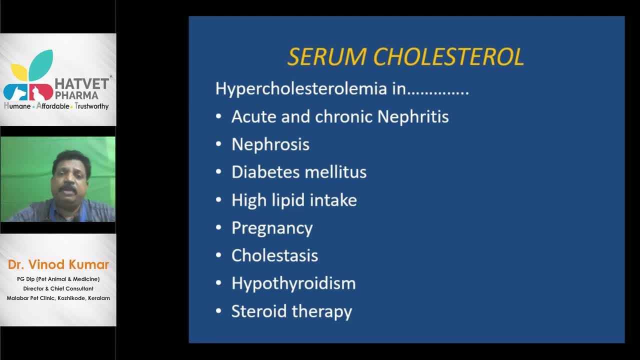 Then hypothyroidism. For the metabolism of cholesterol, thyroxine hormone is invariably needed. That is why, if there is hypothyroidism, there is increase in serum cholesterol, Then in corticosteroids therapy, the same as in diabetes mellitus, there will be increase. 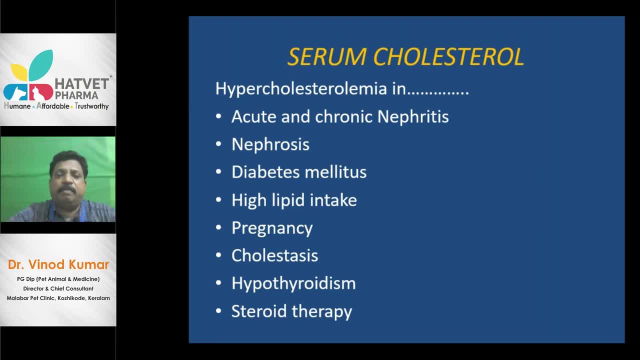 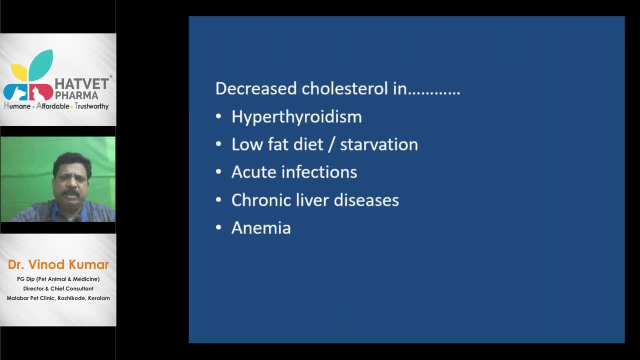 in BGL, that is, blood glucose level, producing hyperglycemia, and some amount of sugar will be converted to cholesterol, producing hypercholesterolemia. Sometimes you can see decreased cholesterol. There are some things which we should correlate in the clinic. In hyperthyroidism there is 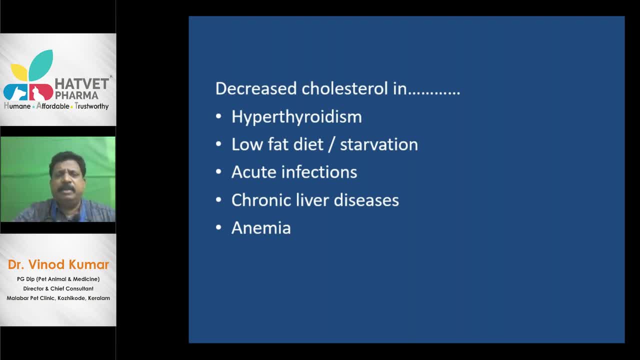 decreased cholesterol, because just now I said that hyperthyroidism is not a feature of dogs and hypothyroidism is not a feature of cats. In cats, generally, we can see hyperthyroidism only In dogs. we can see generally hypothyroidism only. So in hyperthyroidism there is a decrease in cholesterol. In cats generally we can see decreased cholesterol. So in hyperthyroidism there will be increased metabolism of cholesterol and there will be decreased blood cholesterol. Then otherwise in starvation, of course starvation. 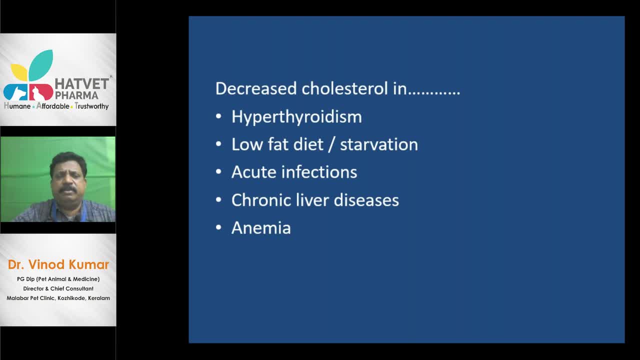 the food is less and so low fat diet, decreased cholesterol level occurs. Then high cholesterol in acute infections- not all infections, in some infections low cholesterol. low cholesterol in acute infections due to increased metabolism of the cholesterol due to infection. Then chronic liver diseases. it is highly substantiable. It is the number one test which is usually 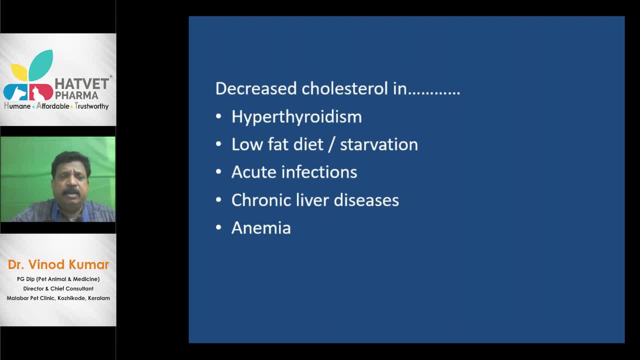 done in chronic liver diseases. Take the blood, allow to clot it, give the serum to the laboratory in chronic liver disease. you can go for any other test parallel to it- ALT, AST, whatever it be Along with that if the cholesterol is low, since the liver is the main seat of cholesterol synthesis. 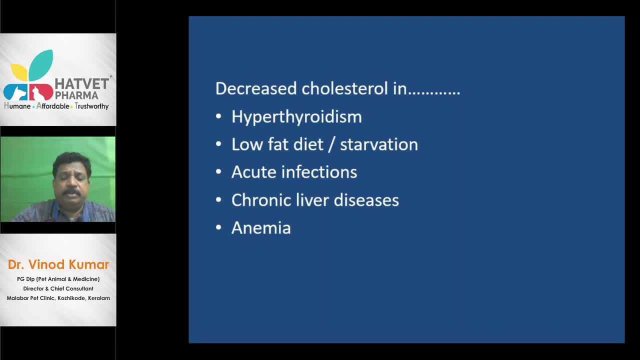 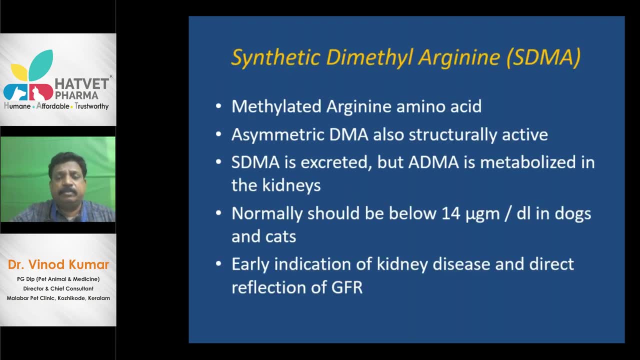 it shows hypokalistrolemia. The same thing happens in anemia, also hypocholesterolemia. Then the thing is that synthetic dimethyl arginine, SDMA. Now, most of our doctors are not much aware of this SDMA, But especially in my place in Kerala. 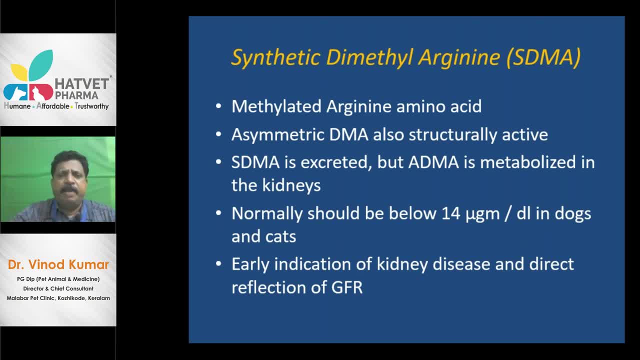 state this has not come into practice. Just, I want to tell a nutshell of this SDMA, Synthetic dimethyl arginine. It is a true reflection of the kidney function. Nowadays we are taking the kidney function tests such as blood-durian hydrogen, blood-durian hydrogen, blood-durian. 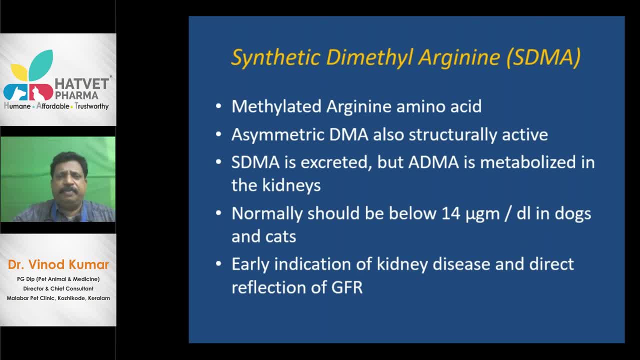 hydrogen, creatinine, uric acid etc. But we get the creatinine level at only the end stages. During the first stages the creatinine will see. we have four stages of the kidney environment. During the first and second stages there may not be much high kin or there may. 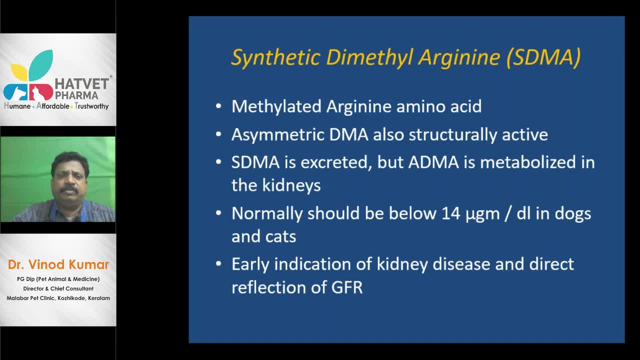 not be any high kin creatinine at all. Only during the third and third stages there may be less than 10% adult shr ballots that are scratchy And also shortly before the fourth stage there will be a steep high in creatinine and blood-durian hydrogen, But at this time 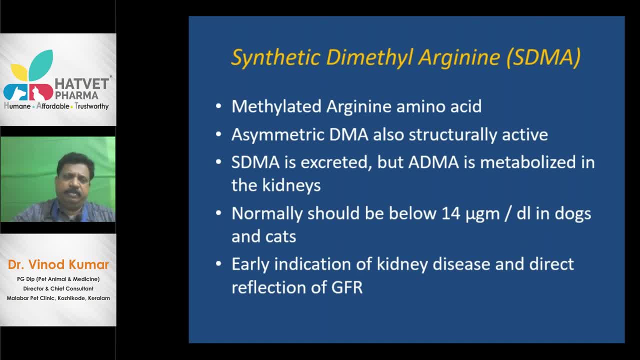 you won't be able to save your kidneys, But this SDMA can be considered as the simplest marker, the earliest marker of kidney disease. It is a methylated DNA. This will help us people. It is a stretch which is Oke and 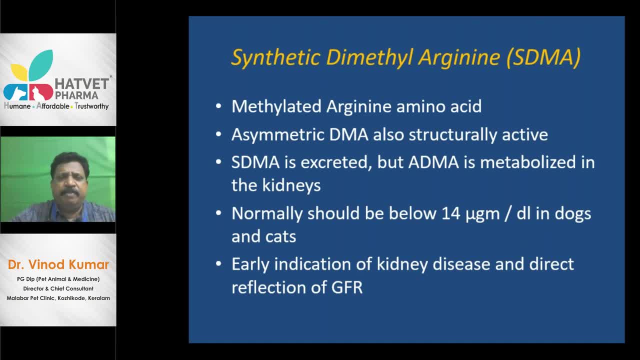 arginine amino acid. Arginine is an amino acid. It is essential amino acid. It is always conjoined with asymmetric DMA, ADMA, But synthetic DMA is excreted through the kidney and we are taking this part. Synthetic DMA is excreted through the kidney, but ADMA is metabolized. 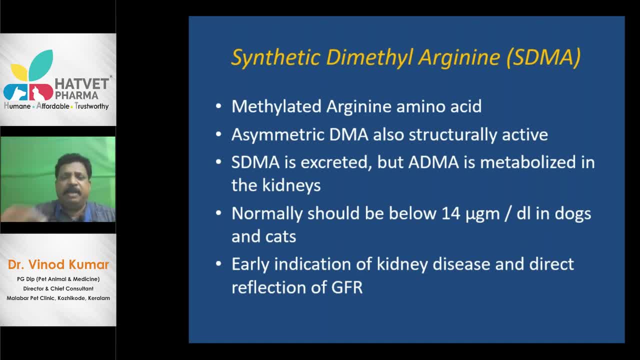 the kidney. So since synthetic DMA- that is, SDMA- is excreted through the kidney, we take it as more significant. It is inside the cells and when this is excreted it can be considered as an early detection of a kidney disease- SDMA whenever you are suspecting a kidney. 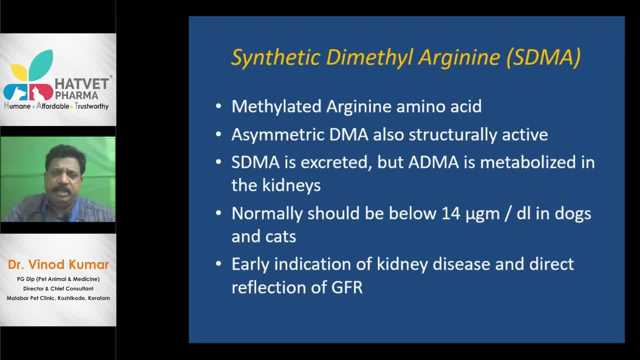 disease, it is considered as an early detection of a kidney disease- SDMA. whenever you are suspecting a kidney disease, it is considered as an early detection of a kidney disease, whether acute kidney injury or chronic kidney disease, AKI or CKD. 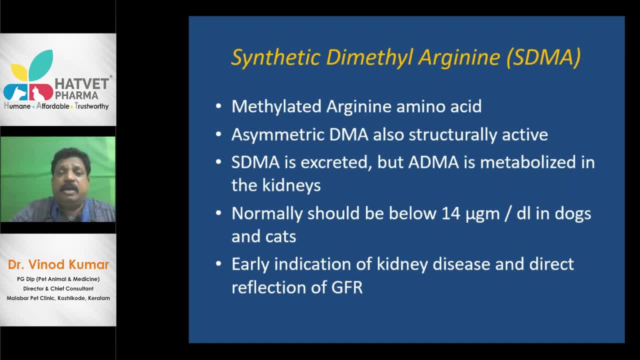 AKI is the new name of ARF and CKD is the new name of CRF, chronic renal failure and acute renal failure. Both these cases, if you want to distinguish, there is a renal impairment. the best is SDMA estimation, But unfortunately in not all the places it is available. 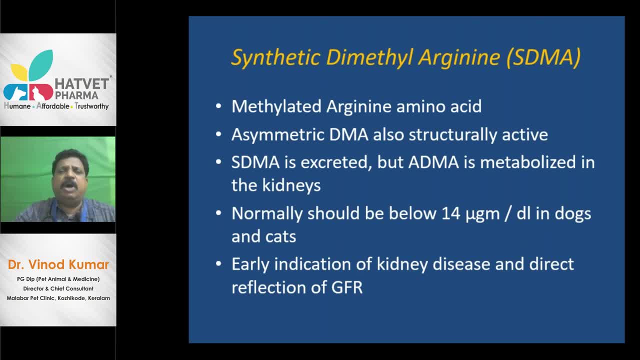 But unfortunately in not all the places it is available And generally in dogs and cats it should be below 14 micrograms per deciliter. That is a normal level. It should be below 14 micrograms per deciliter. Especially if it is a pup or a kitten, it should be below. 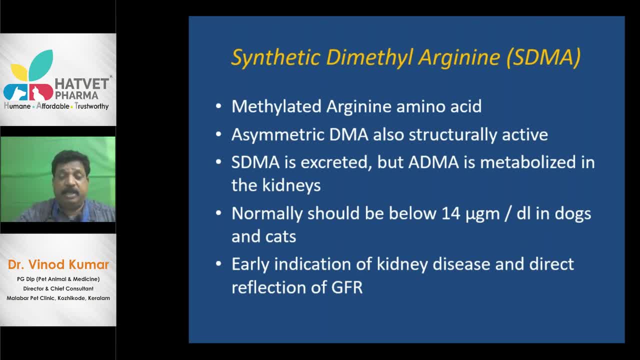 16 micrograms per deciliter. That is another thing which we have to consider according to the age. It is a pup or a kitten, But generally, if it is an adult dog, it should be below 14 micrograms per deciliter. SDMA should be below 14 micrograms per deciliter. It is. 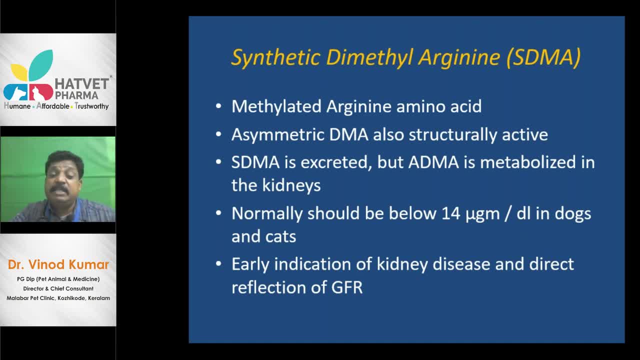 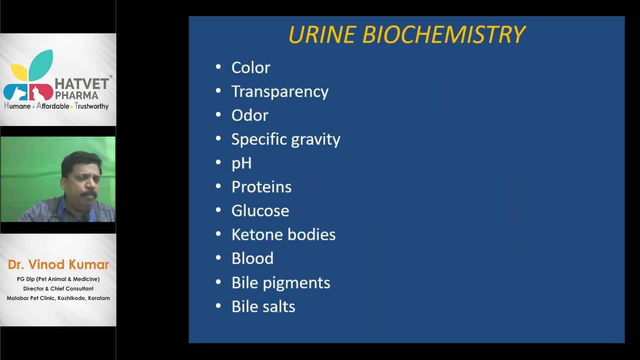 an early indication of a kidney disease and it can be considered as a direct reflection of the glomerular filtration rate. That is why it is said to be an early indicator. Just keep in this mind, Keep in your mind. Now we have completed. 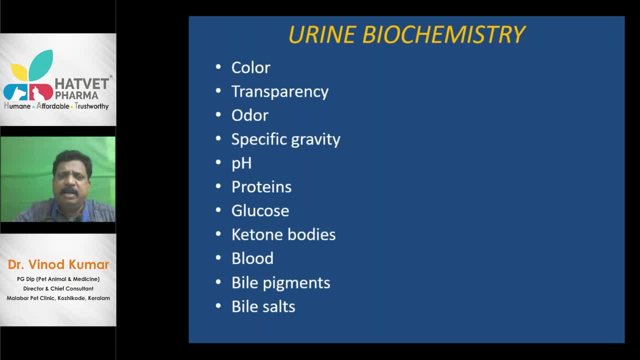 some factors in the blood which we term as the serum biochemistry. But the serum biochemistry should be always conjoined with the urine biochemistry, or at least in most of the cases. So we have to study something about the urine biochemistry also when we are studying the 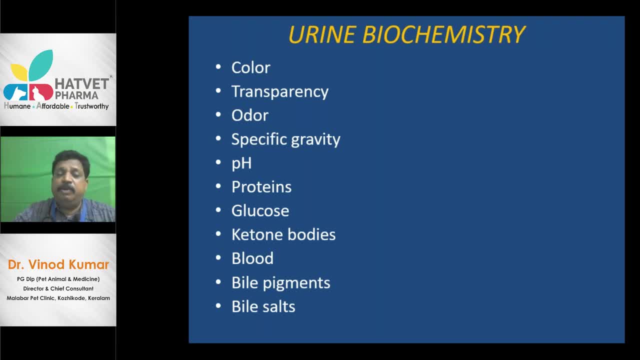 serum, biochemistry In the urine, In the urine. In the urine We are taking the color, the transparency, the order, the gravity, the pH, the proteins, the glucose, the ketone bodies, the blood, the bile pigments, the bile salts, etc. 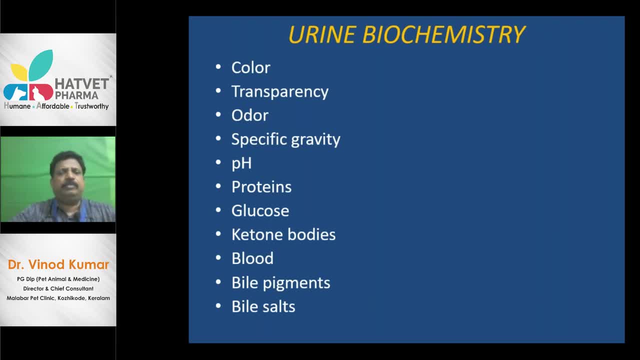 When coming to the urine color, it should be clear and, due to the chanthochrome pigments, it should be light yellowish. If it is more watery and colorless, it could be polyurea. if it is too yellowish, it could. 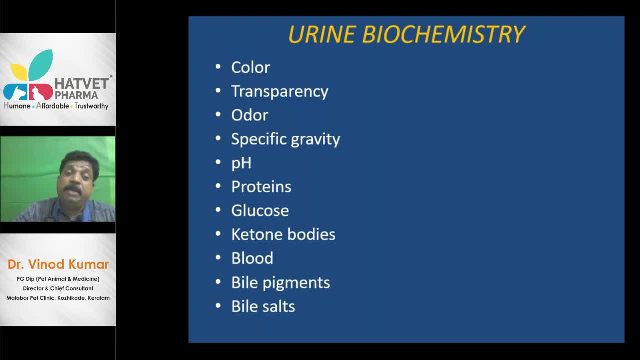 be pterurea. Red means it could be hemoglobinuria or hematuria. whether we have to find it out by centrifugation. So the next question is: what is the difference between the two? Transparency Urine is so turbid, it could be highly cellular. it could be cystitis. order generally the 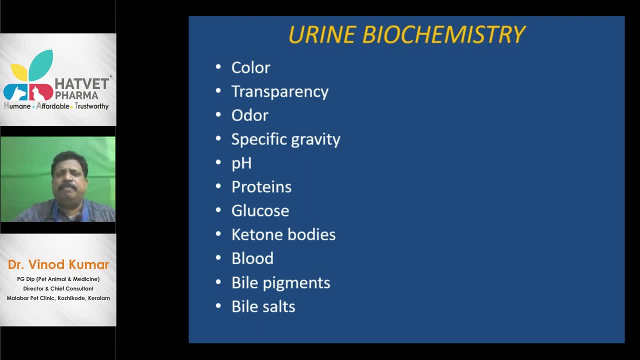 order is. it is orderless, but the order of the Dalmatian's urine is too offensive due to presence of high amounts of allantoin in the Dalmatians. In the normal dogs and human beings, protein is metabolized. ultimately, uric acid is formed. 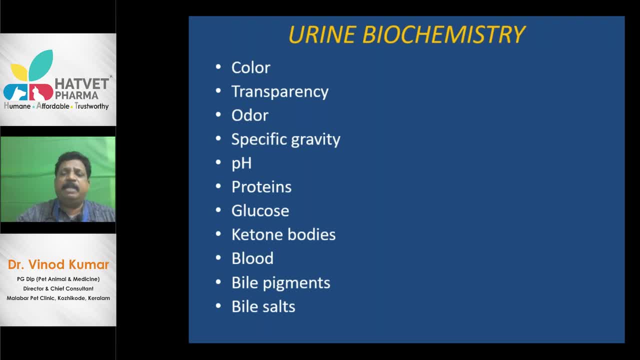 the uric acid is detoxified to urea in the liver by the enzyme uricase. But in the Dalmatian dog, since there is negligible amount of uricase enzyme in the liver, uric acid cannot be detoxified to the urea. 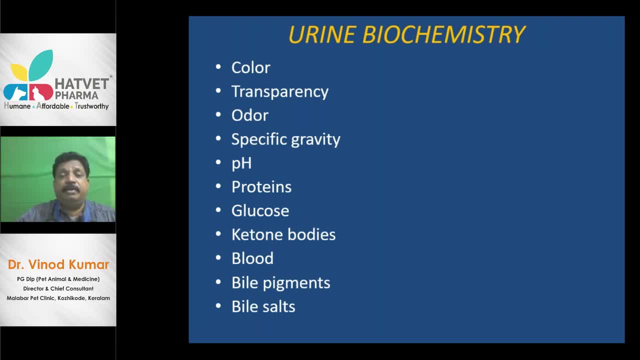 But will be converted to a toxic allantoin. allantoin has a tendency: in the presence of allantoin, all the solids may precipitate very easily. That is why Dalmatians have a high tendency of urolithiasis. 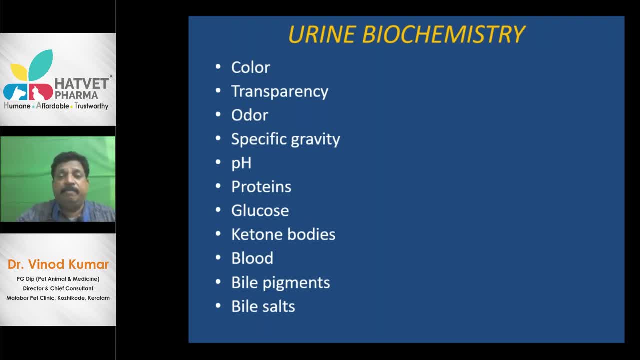 And this allantoin, when excreted through urine, it gives a very pungent offensive order for the Dalmatian's urine. Then the specific gravity of the urine. The specific gravity of the urine. The specific gravity of the urine. 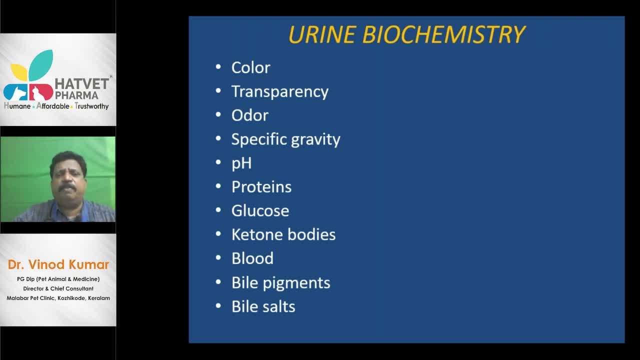 Normally it should be 0.015 to 0.03.. Any urine which is having less than 0.15, 0.015 specific gravity is known as hyposthenuria or hyposthenuric urine, and when the specific gravity is increased above 0.03, it is known. 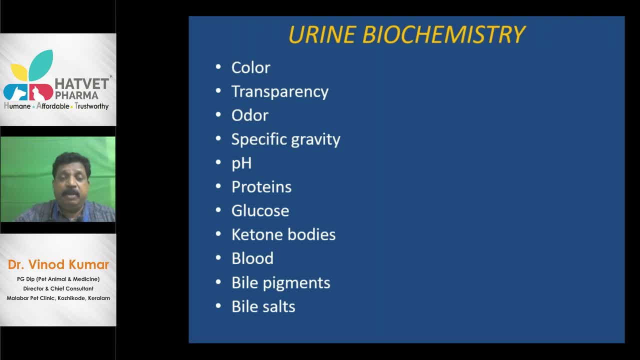 as a hyperstenuric urine. Hyperstenuria increased to 0.03.. Solids in the urine or in the specific gravity of the urine, very commonly seen in Addison's disease. Hyposthenuria is generally seen in polyuria, such as diabetes mellitus or Cushing's syndrome. 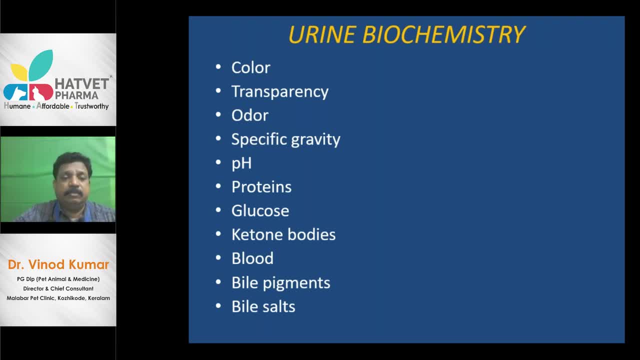 or diabetes insipidus. The pH of the urine generally- the carnivore urine and the omnivore urine- is slightly acidic. we all know If it is towards alkaline side there should be some infection Proteins in urine. it is PLN protein. losing nephropathy can happen mainly in kidney diseases. 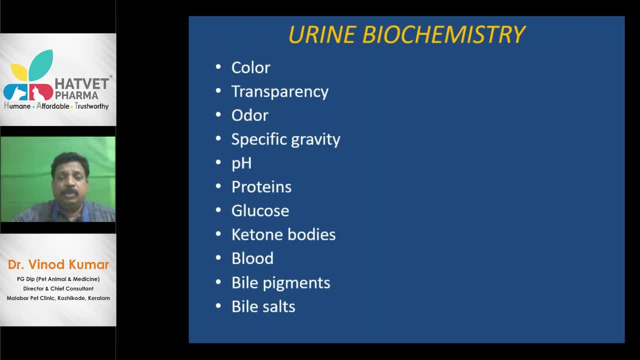 It is an indication that there is a kidney disease. Glucose in the urine: yes, that could be due to hyperglycemia, may be due to diabetes mellitus, may be due to Cushing's syndrome. If it is towards alkaline side, there should be some infection. Proteins in urine. it is PLN protein. losing nephropathy can happen mainly in kidney diseases. It is an indication that there is a kidney disease. Photocardioid-acidosis in urine is always related to Cushing's syndrome, which we have. 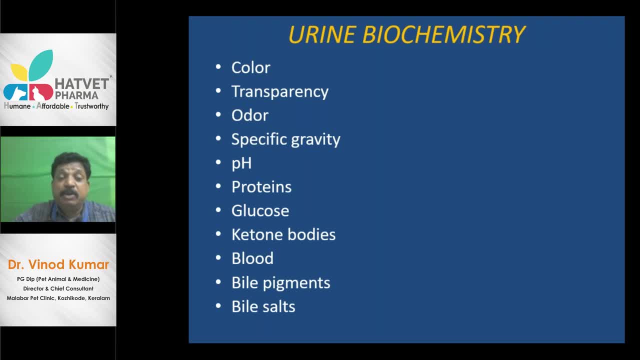 to find out. Ketone bodies could be diabetic ketone acidosis, DKA. It is a common complication of diabetes mellitus where we have to find it out. Blood in urine can be cystitis or any bleeding points, stones inside bile, pigments and bile. 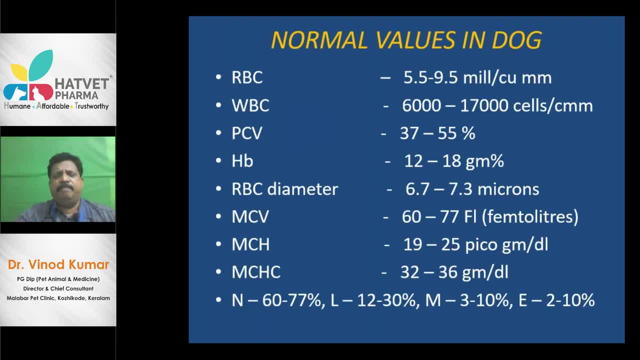 salts in Ygterus, that is, in jaundice. See, all these things we have to understand. Bile pigments and bile salts. in the ygteras Yesterday we have mentioned about all these things: RBC, WBC, PCV. RBC normally is 5.5 to 9.5 million per cubic millimetre. 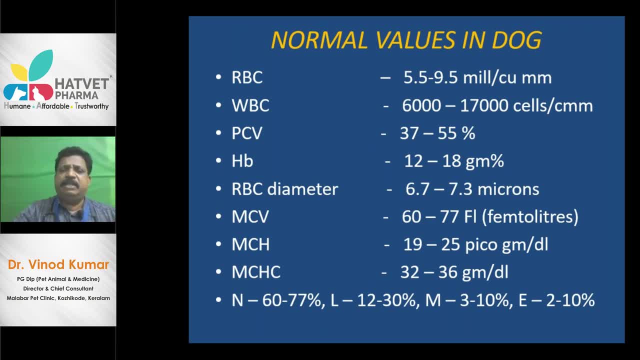 WBC normally is 6000 to 17000 cells per cubic millimetre. PCV normally is 37 to 55%. In the cat it is normally 37.. In the dog- remember my fluid therapy class- In the cat normally it is 37%. In the dog. normally it could be 45%. Hemoglobin should be 12 to 18 gram per cent. Mean corpuscular volume should be 60 to 77 femtolitres. It is FL 60 to 77 femtolitres. 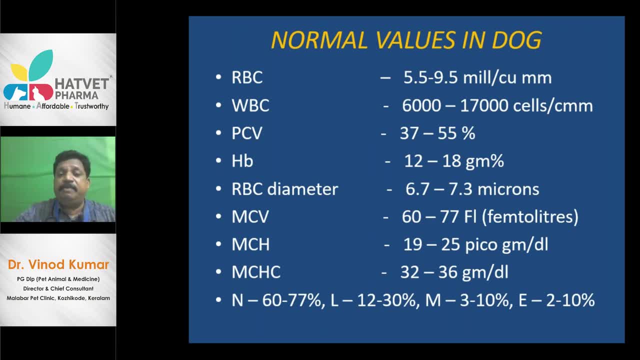 MCF. MCF is 19 to 25 picogram per deciliter. MCHC is 32 to 36 gram per deciliter. Remember our MCV class yesterday, MCH, yesterday, MCHC. yesterday MCHC is increased. 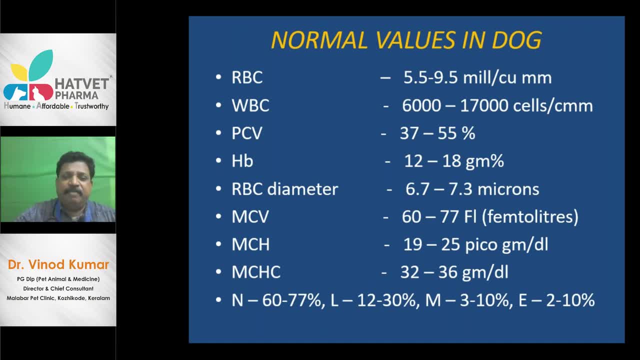 In IMHA. MCV is increased in B12 deficiency, MCH is decreased in B12 deficiency, Iron deficiency and anemia. Remember all these things. I will ask you with putting a question paper. Then the normal neutrophil in differential count: Normal neutrophil count is 60 to 77 per cent. 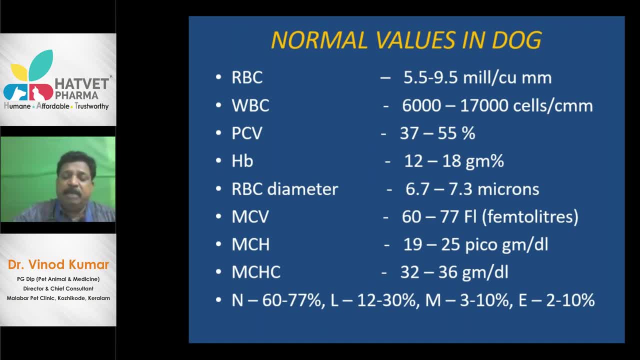 Lymphocyte 12 to 30 per cent, Monocytes 3 to 10 per cent And eosinophils 2 to 10 per cent. Okay, Then, the normal calcium level should be 9 to 11 milligram per cent. 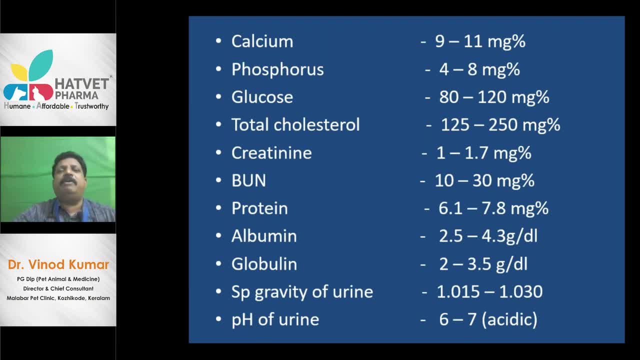 This we have to study by heart Or you have to paste it inside your room. Normal calcium is 9 to 11 per cent, Phosphorus is 4 to 8 milligram per cent. Glucose is 80 to 120 milligram per cent. 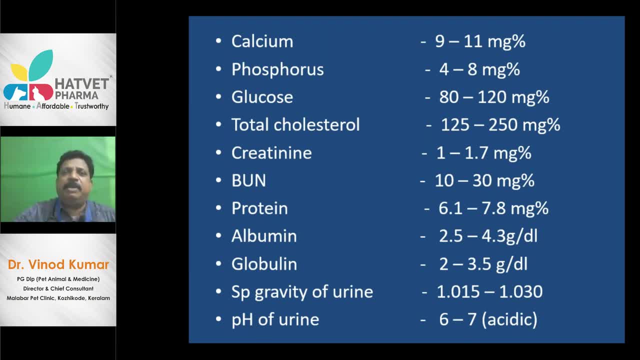 Total cholesterol is 125 to 250 milligram per cent. Creatinine is 1 to 1.7 milligram per cent. What about the SDMA? It should be below micrograms per cent. Protein and antigen should be 10 to 30 milligram per cent. 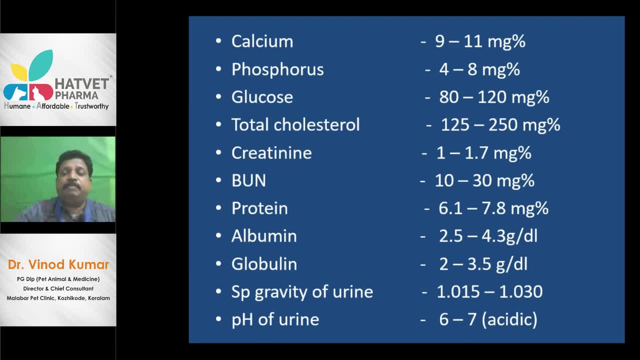 Protein should be 6.1 to 7.8 milligram per cent. Antimicrobial fraction of the protein should be 2.5 to 4.3 gram per deciliter. Globulin 2 to 3.5 gram per deciliter. 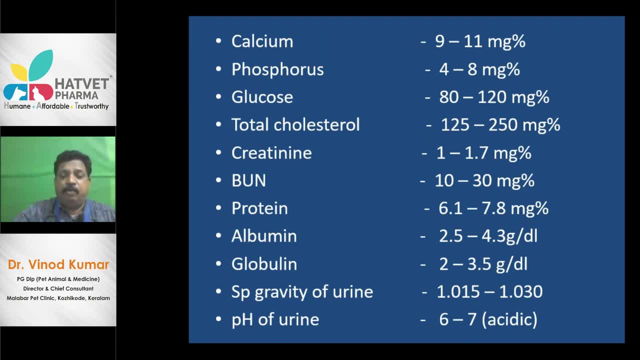 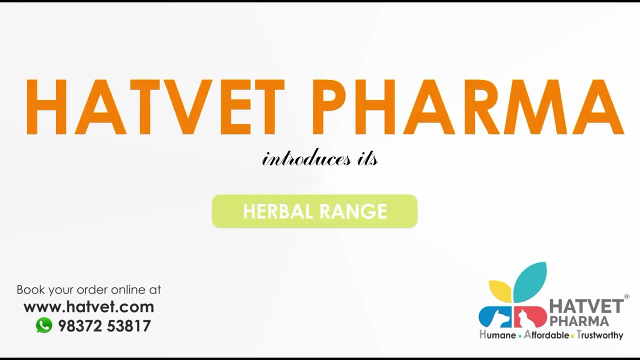 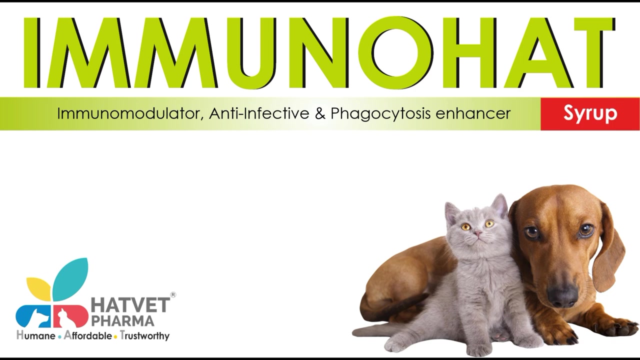 The specific gravity of urine should normally be 1 to 1.025 to 1.030.. Then the pH of urine. it should be slightly acidic, 6 to 7.. So the pH of the urine should be around 8 to 7.1 to 5.2. 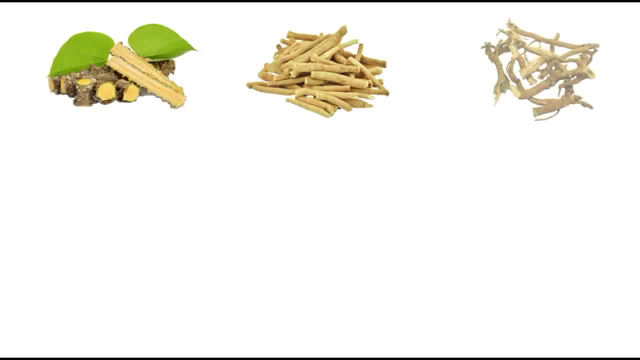 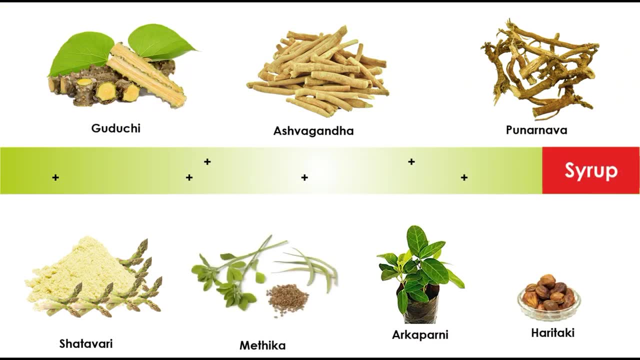 I'm not sure if I'm right, I'm not sure if I'm wrong, I'm not sure. What about the Fagocytosis enhancer? The Fagocytosis enhancer is an anti-inflammatory and phagocytosis enhancer. 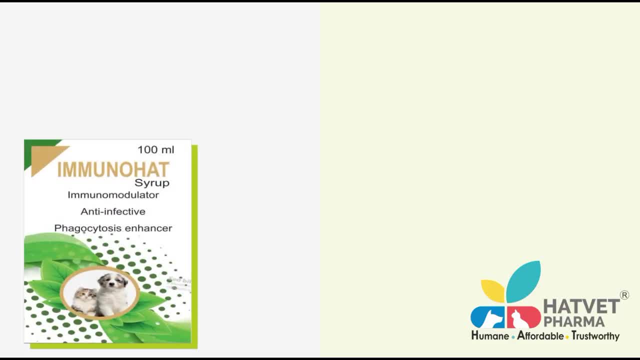 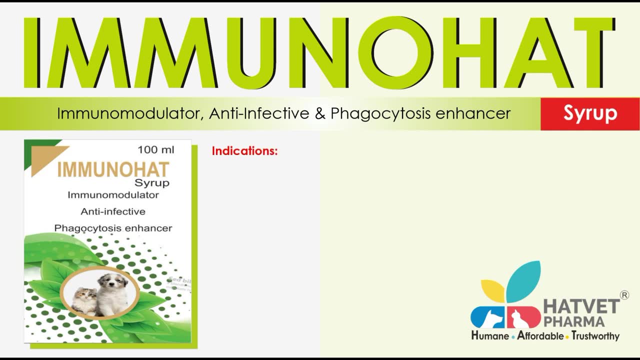 It is a natural immunity modulator, with the benefits of Guduchi, Ashwagandha, Punarnava, Shatavani, Methika, Alka-Palni and Haritaki herbs, Helps in improving the phagocytic index and results in faster recovery. 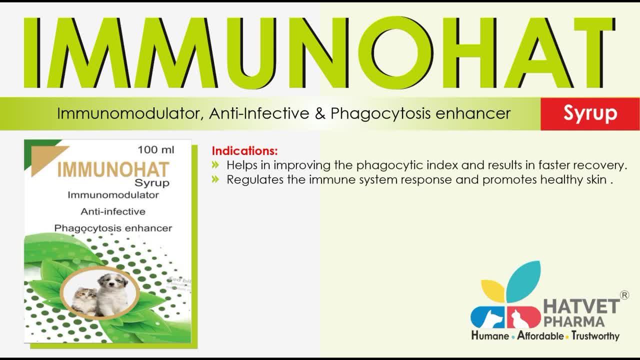 Regulates the immune system response and promotes healthy skin. Pre and post vaccination in pups and immune compromised animals. As an adjuvant with antibiotic therapy, As a supportive with steroidal therapy, specially in skin infections. Dosage for small breeds: 1-2 ml twice a day. 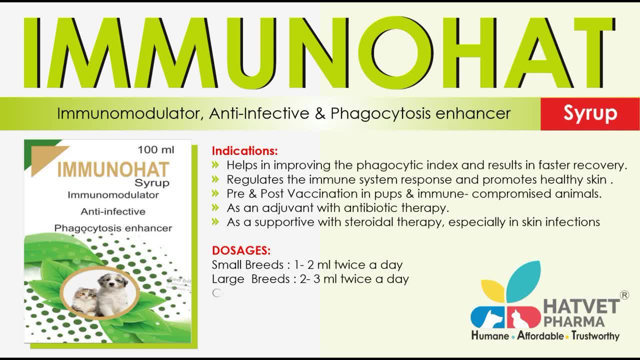 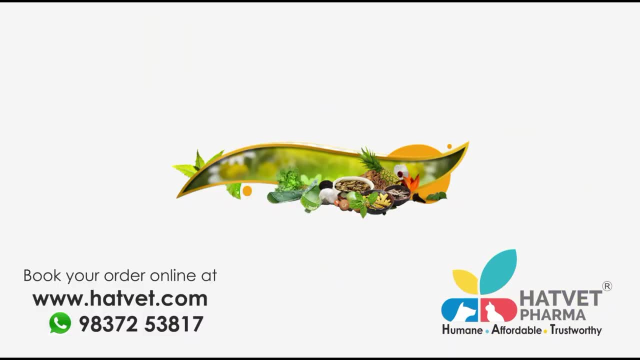 For large breeds: 2-3 ml twice a day. For cats: 1 ml twice a day. Root or Root Presentation: 100 ml. You can book your order online at wwwhatfitcom, Looking forward to a long lasting business association. 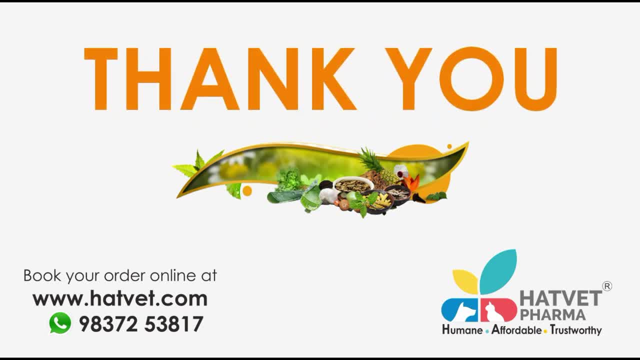 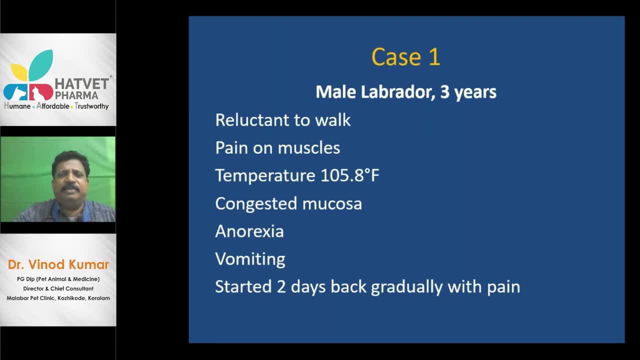 Thank you, It is normally labradors will not bite, but some male labradors may bite. Pain on muscles and severe pyositis. The temperature when I took was 105.8 degree Fahrenheit And there was a congested mucosa. 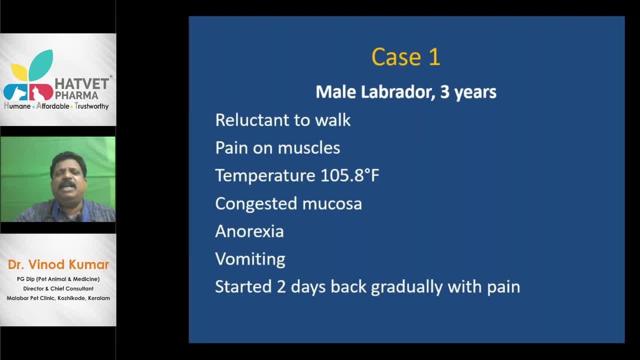 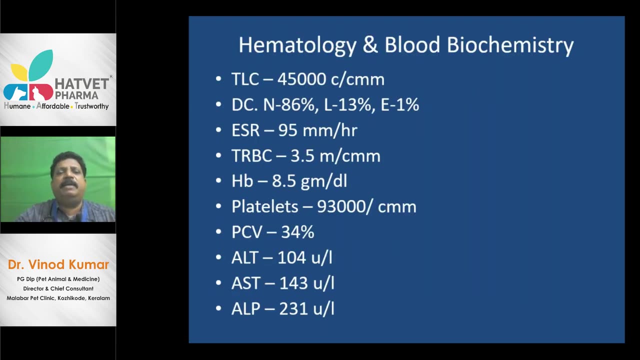 It was having anorexia and vomiting Started 2 days back, gradually with pain. It started with fever and pain and now the pain is very intense and it cannot work. It is anorexic and not at all vomiting. So I took the blood and subjected for hematology and blood biochemistry. 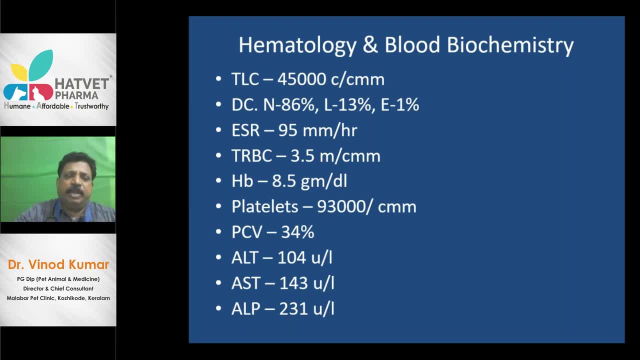 See. the total leukocytic count is 45,000 cells per cubic mm. The differential count is: neutrophil 86%, lymphocyte 13%, eosinophils 1%- See the ESR: 95 mm per hour. It is very high. 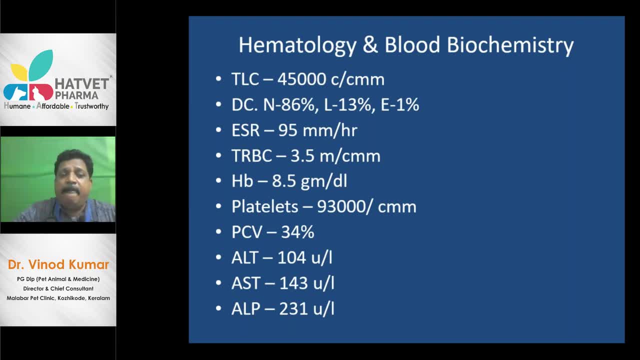 The total RBC. It is very high. The RBC is 3.5 mm per cubic mm. It is low. there is anemia. Hemoglobin is 8.5 grams per deciliter. Platelets were low. It is 93,000 cells per cubic mm. 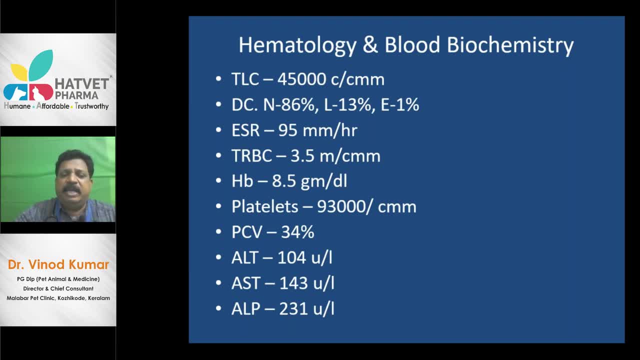 PCB is low, 34%. Then the ALT AST, ALP. of course I have not gone through it. That is why I thought next day it should be. But now ALT AST is high anyway. There is hepatic impairment, See this. 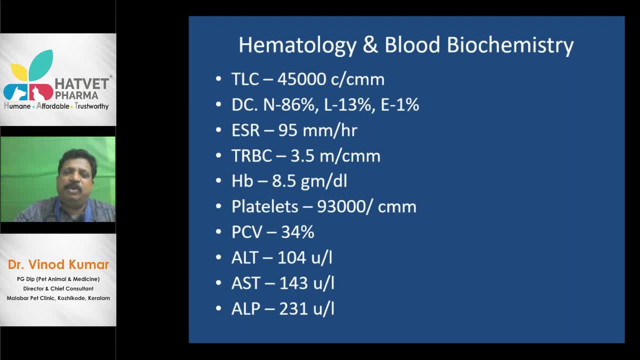 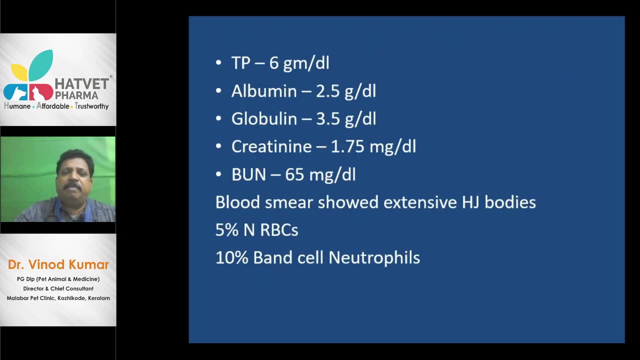 Severe leukocytosis, severe neutrophilia, ESR is very high, with anemia, thrombocytopenia, low PCV hepatic involvement And total protein was 6 grams per deciliter. normal. Albumin is 2.5 grams per deciliter normal. 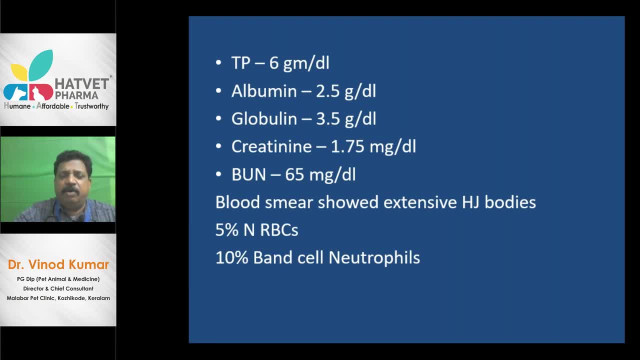 It is slightly low Globulin. normal Creatinine is slightly high or to the upper border. Blood urinary nitrogen is elevated. Blood smear showed extensive hovel jolly bodies. 5% nucleated RBCs were there. 10% banned neutrophils. 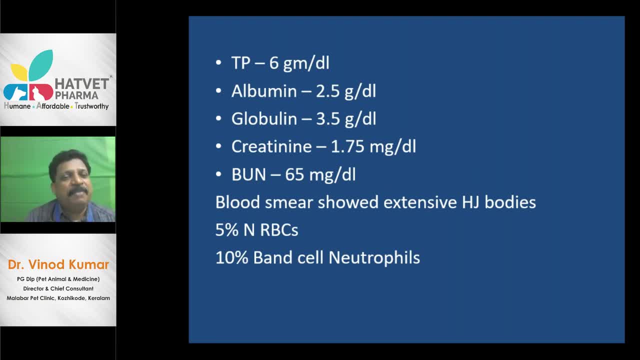 That is regionally reduced shift left. See the leukocytic count is 45,000.. 10% banned neutrophils, That is regionally reduced shift left. So, naturally, from this blood work, from this PE findings, what could be the disease? 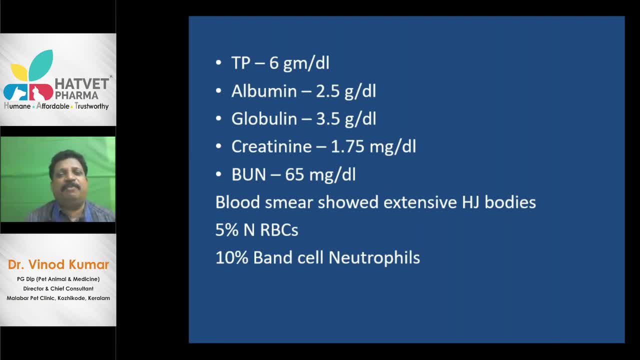 Naturally, almost 90% of our doctors definitely have the answer. I know very well. Now I will give you a clue. I gave, knowing very well the disease. I gave benzyl, penicillin and it responded very well. So now you know what the disease is. 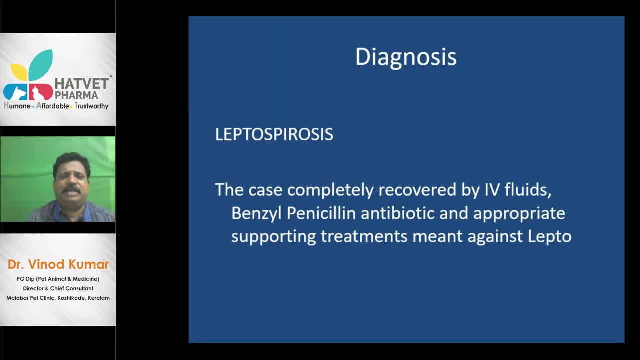 So diagnosis came. It is very easy to diagnose that it was leptospirosis. In leptospirosis there is no MAT, there is no microagglutination test in our laboratory field. diagnostic conditions: All stalwarts say we have to diagnose, mostly or only if we are in the veterinary college. 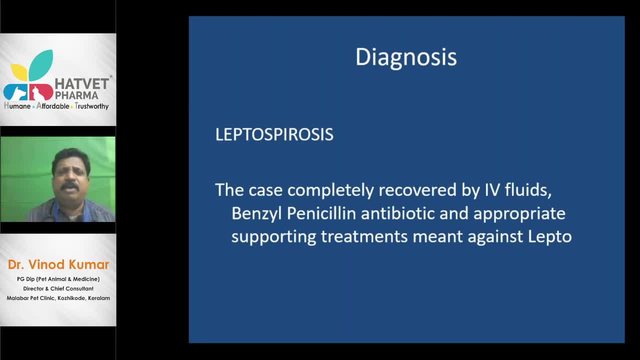 Of course we can go through the test inside the college. But we are not in the college, we are in the field. We can go through the field diagnostic methods only Here, for field diagnosis is just through hematology, blood biochemistry examinations and clinical findings. 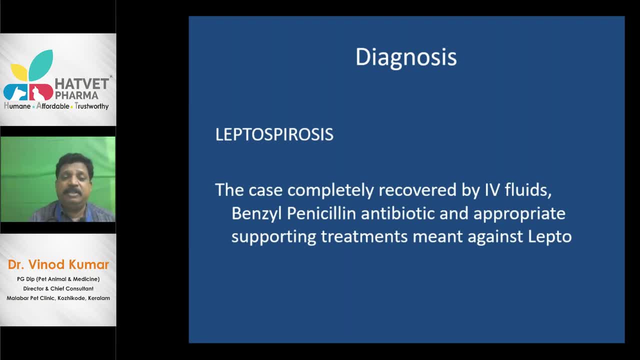 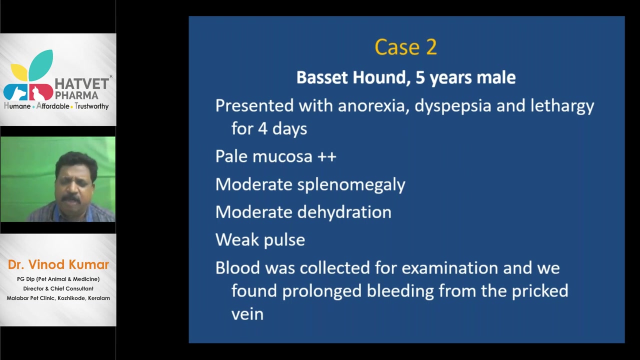 So the case completely recovered by IV fluids, benzyl, penicillin and appropriate supporting therapies meant against leptospirosis. So that was a very simple example quoted. Let us take a second example, Another basset hound. See, I still remember the patient, the owner of the dog. 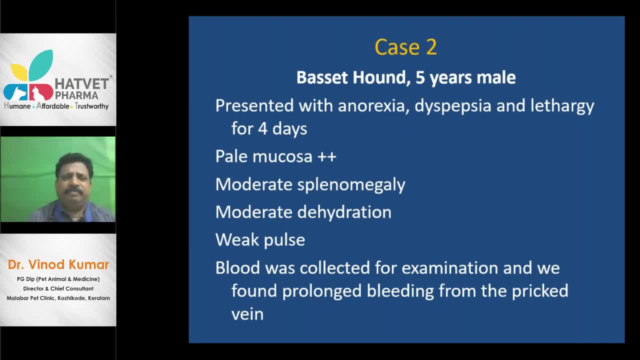 He is a very gentleman breeder. It was a male 5 years old basset hound Presented with anorexia. It had dyspepsia and lethargy for 5 days. No, she was telling that: no eating, no drinking and very weak for the last 4 days. 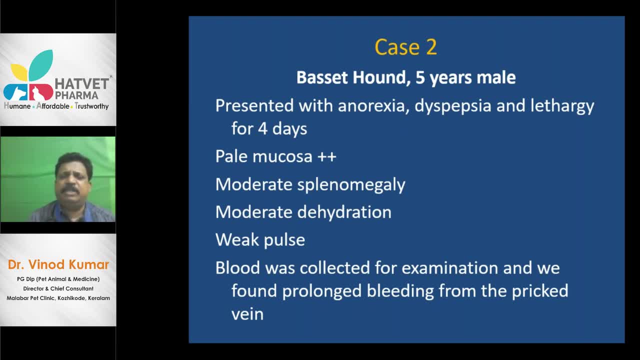 There he called a doctor. He was a quake, I think. He came there, He gave some injections- I don't know what it was- Ranitidine or something. Then he left. On clinical examination it showed a pale mucosa 2+. 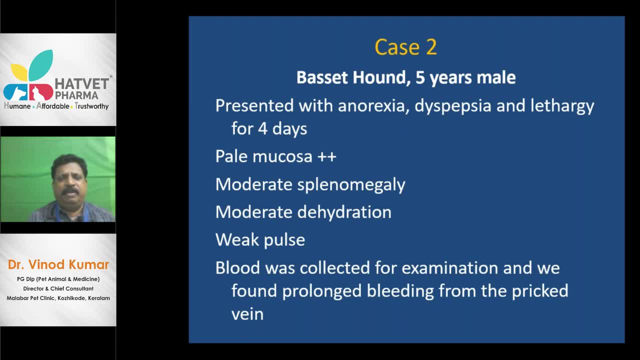 It showed moderate splenomegaly. Now the clue is coming: It showed moderate splenomegaly. It showed moderate dehydration, It showed a weak pulse. So with these clinical findings- And in this case I remember there was swollen prescapular lymph nodes- 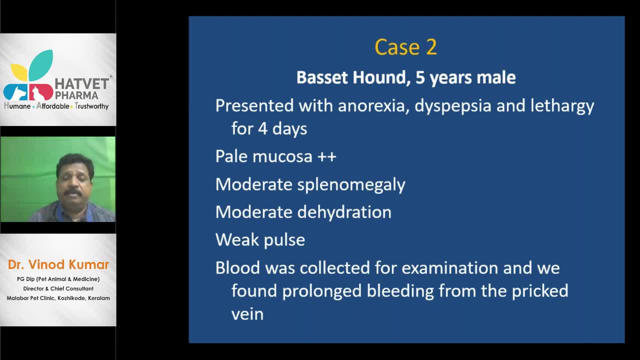 This case, blood was collected and examined. See, when I pricked the vein it took lot of time to stop the bleeding from the vein. Nowadays, in our clinic, If we get a case of whatever is the bleed, If we get a case of anorexia with dyspepsia, 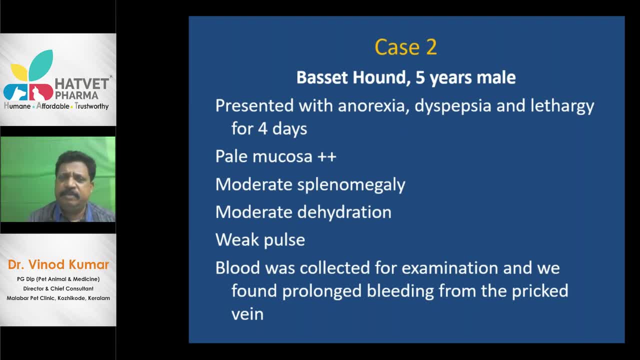 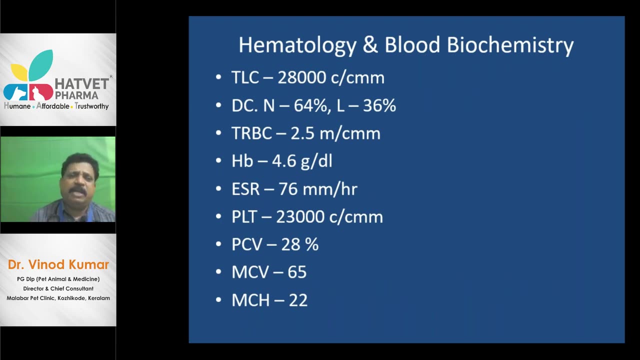 Weakness And the physical examination finding is anemia with splenomegaly- What should be the assumption, Because this disease is very, very common. And we subjected the blood for hematology and blood biochemistry, We saw that total leukocytic count was 28000 cells per cubic millimetre. 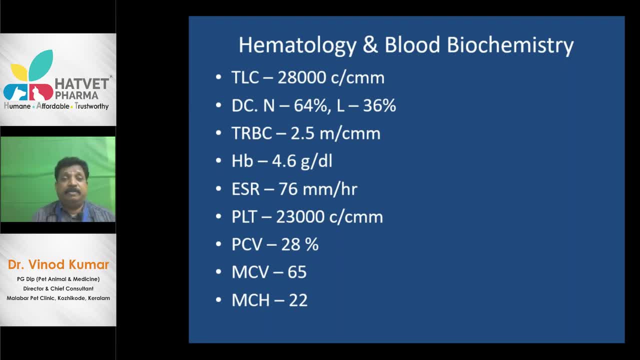 It is high, of course, But not like the leptospirosis Coming to DC. Neutrophil 64%, Lymphocyte 36% RBC is too low. It is 2.5 mL per cubic millimetre. 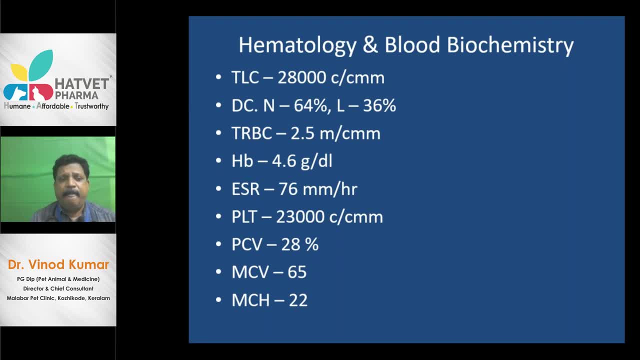 There is anemia. Haemoglobin is 4.6.. Very, very low, Actually. it has to be transfused with blood. ESR is high: It is 76. Blood lead is very, very low, 23000 only. This was a challenging case for us. 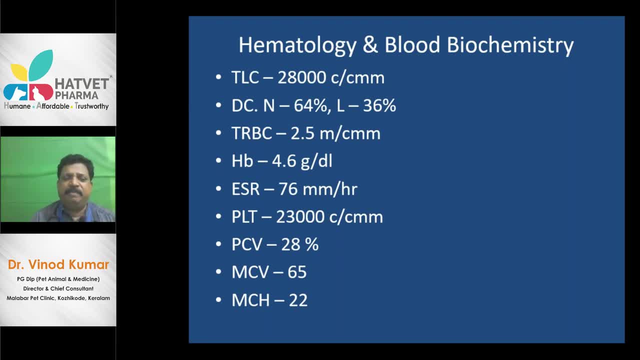 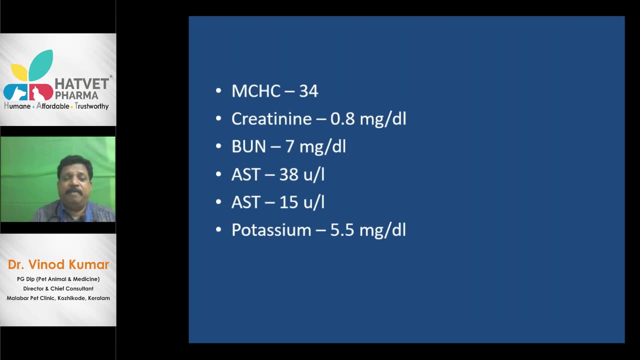 PCV is only 28%. MCV is unremarkable. MCH is low. Definitely, MCH is low Because there is anemia. MCHC is normal. Creatinine is 0.817.. There is no renal impairment. 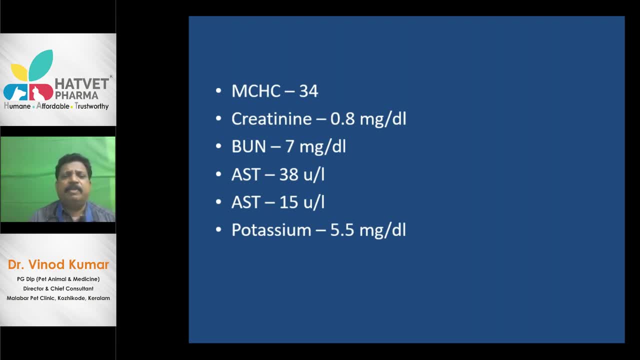 There is no renal impairment, Then AST, AST, ALT, All these things are normal. Of course, there is no hepatic involvement, There is no renal impairment. So what it could be? Now I suspected something. I took the blood On clinical examination. 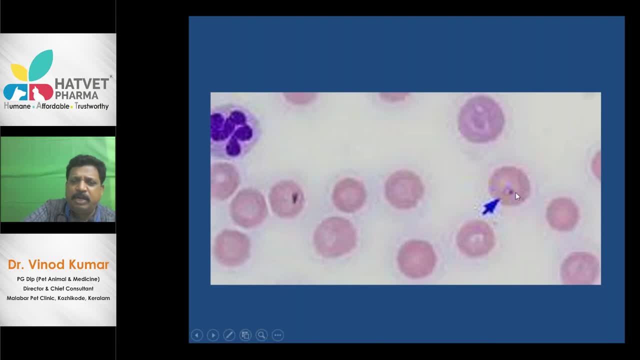 I saw this small thing. What is this? This is very commonly found. This is inside the RBC. You can see the pale RBCs. You can see the anemic picture itself. It was so simple. Very simply, we could diagnose. 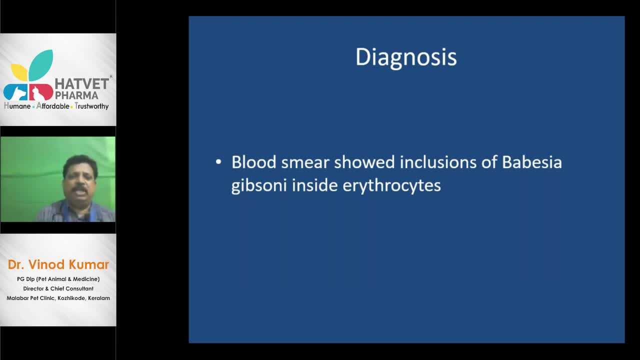 It was Babyshek-Gibsoni. So, my dear friends, Whenever you get such a case, Sometimes in Babyshek-Gibsoni, The leukocytic count will rise To 50,000,, 60,000,, 70,000 cells per cubic millimeter. 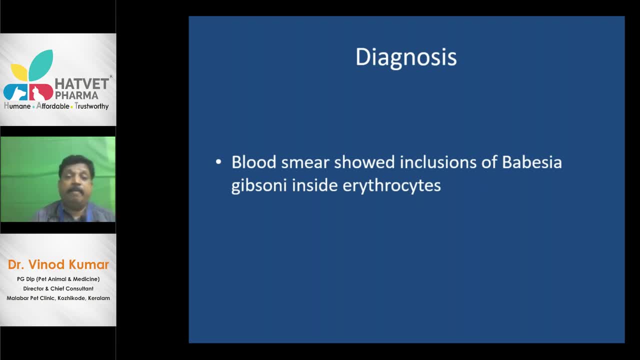 As well as cells per ml. So in Babyshek-Gibsoni, generally, The leukocytic count will be very low, Between 20 and 30.. In Babyshek-Canis, it will be something around Between 30 and 50,000 thrombocytes. 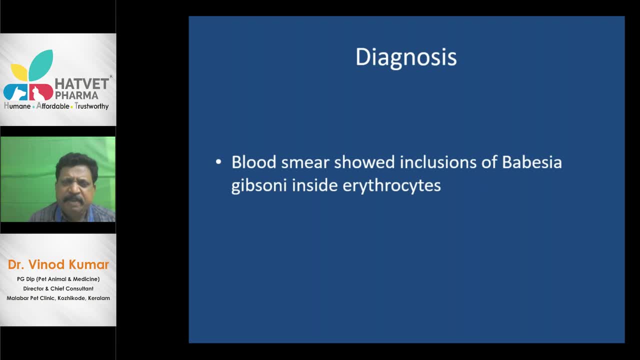 In early Asia it will be something Between 50 and 90. And in leptospirosis Generally it will be between 90,000 and 1.2 leptospirosis Or 1.5 leptospirosis. 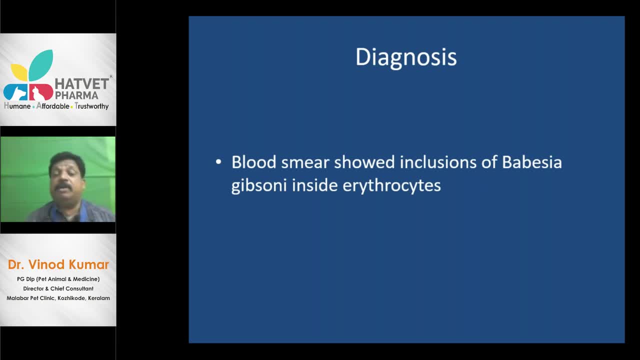 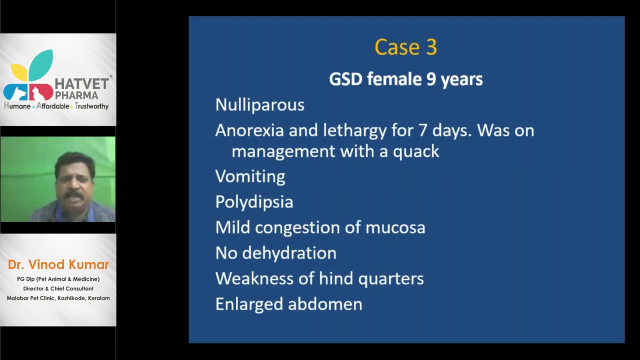 This is my simple assessment on In general Regarding our thrombocytic count. So this was very easy to diagnose. It was Babyshek-Gibsoni infection Inside the erythrocyte. Let us take a third case. 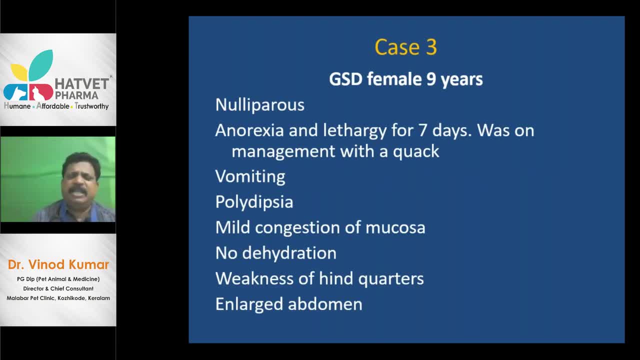 It was a German Shepherd female, 9 years. It is again my friend's dog, 9 years old German Shepherd female. It was presented With anorexia And lethargy for 7 days. He was all the day. 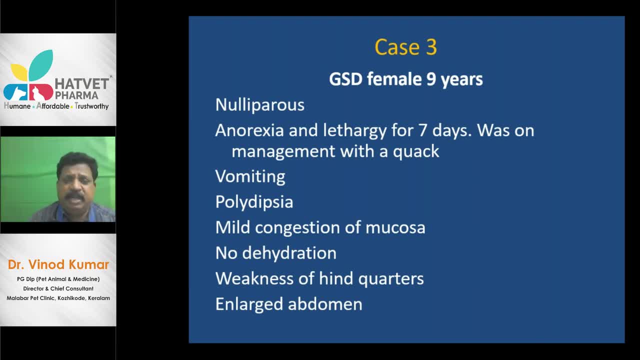 He was calling me, He is not eating anything. I said you give Le 52.. Le 52.. How many times Once I said: you present the dog. No, I have no time Going on with Le 52.. And at last, what happened? 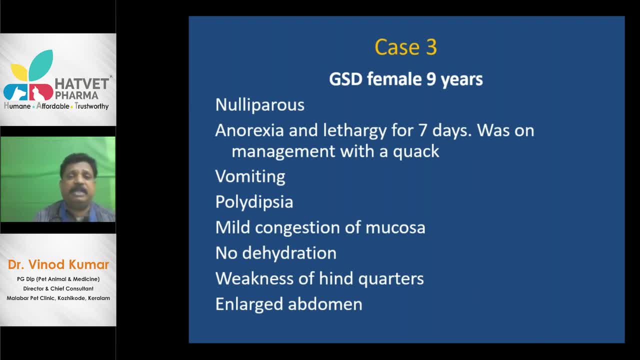 Even I was there. He came back, He gave some injections And there was no response at all. He was presented to me. This Female German Shepherd Was presented to me. I have not ever whelped. It had vomiting. 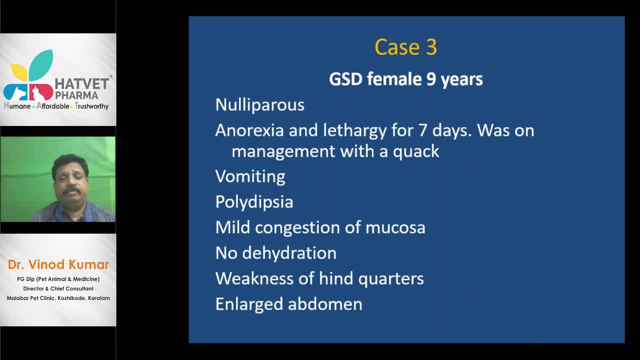 It had polydipsia. There is. There was mild congestion Of the mucous membranes, But Since it had polydipsia There was no dehydration. The hind quarters Was little bit weak. He was having a staggering. 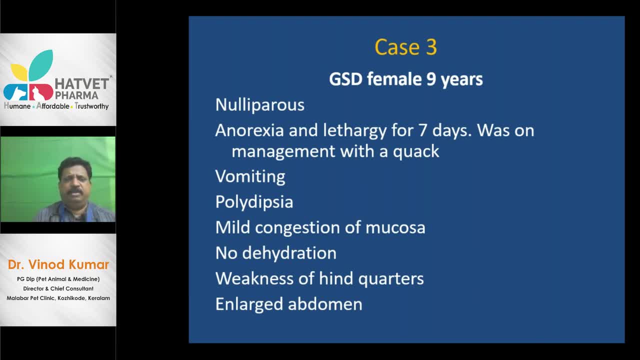 Or swaying gait, Abdomen was enlarged. Now Almost 90% of the doctors Sitting in this webinar. Definitely I know You have diagnosed it. You are very clever living beings. You can very cleverly, You can very easily diagnose it. 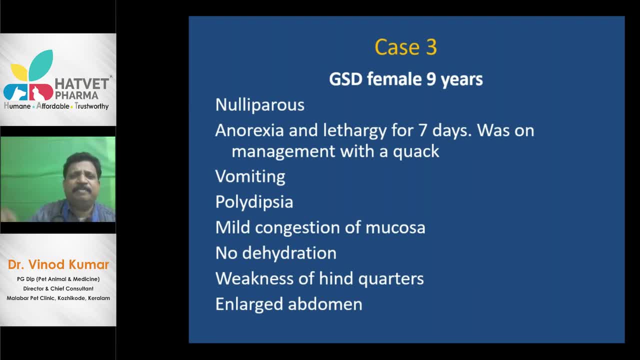 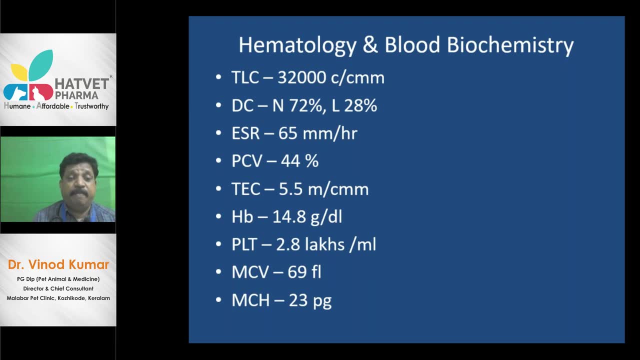 Do it. You are all very clever living beings. Let us come through The hematology and blood vacuum. Total leukocytic count was very high: 32,000.. In DC, Neutrophils: 72%. Lymphocytes: 28%. 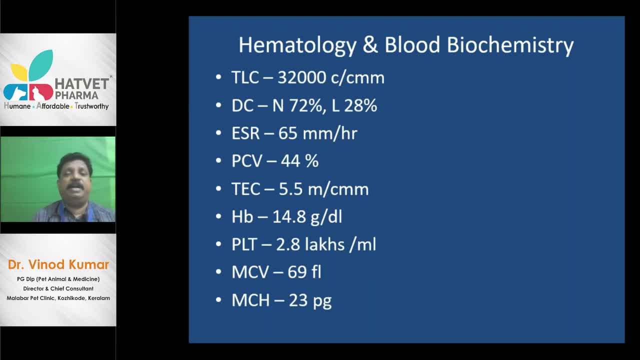 ESR is high- 65.. PCB is normal. It is well hydrated. Erythrocyte count is 5.. Erythrocyte count is normal. Platelet is normal. MCV is normal. MCH is normal. 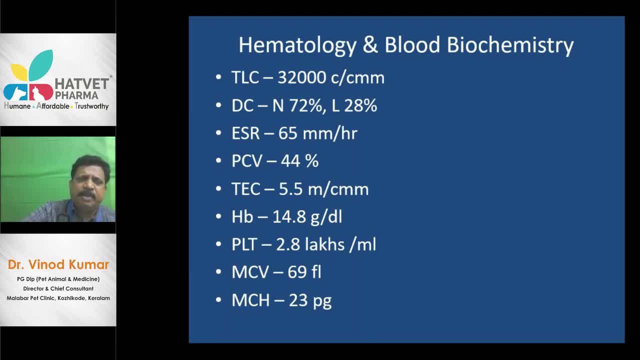 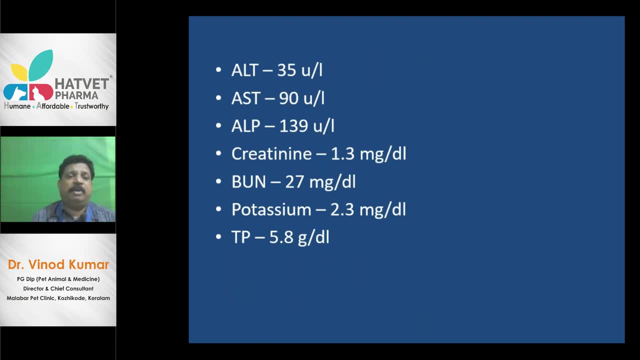 Of course MCH is slightly low, Slightly low, But it can be considered as normal. But the total leukocytic count is high, ESR is high, LT, AST: everything is normal. Liver is normal, Kidney is normal. 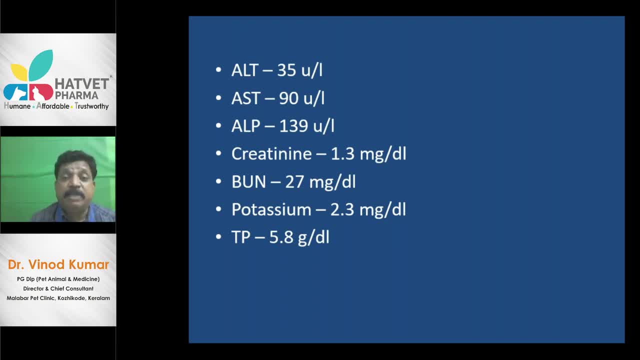 Potassium is slightly low. Why the potassium is slightly low? Because of polyurea. When there is polyurea, Potassium depletion So produces hypokalemia. That is why there is slight staggering rate or weakness of the hindquarters. 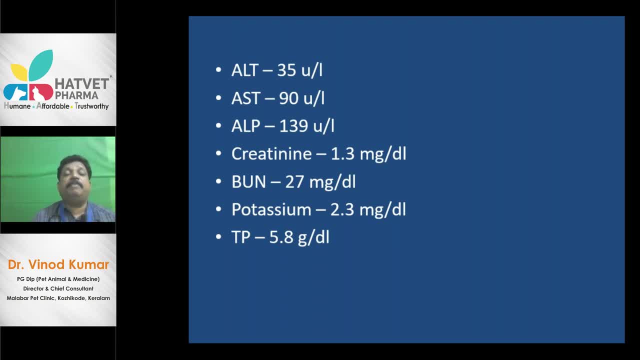 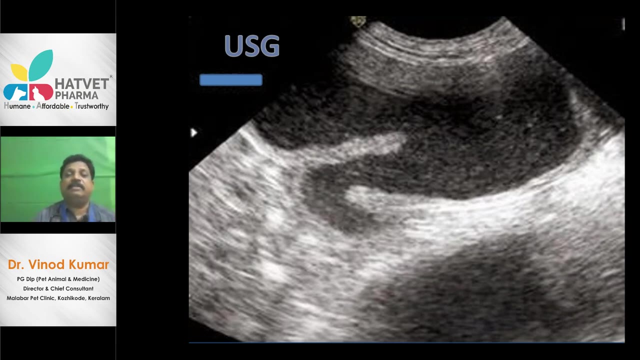 Got it Here. the total protein was 5.8 gram per deciliter is normal. Then what happened? I subjected for ultrasound examination. On ultrasound examination of the abdomen, I saw this. What is this? I know very well, almost 90% of our doctors. 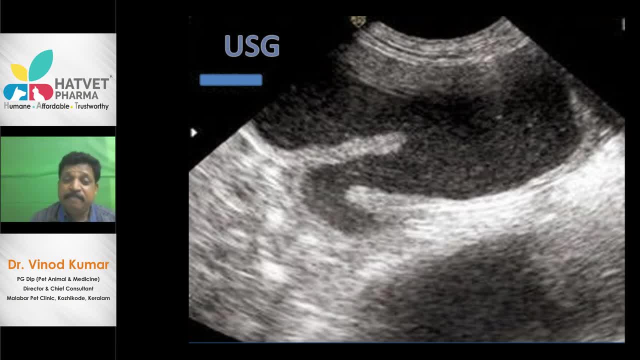 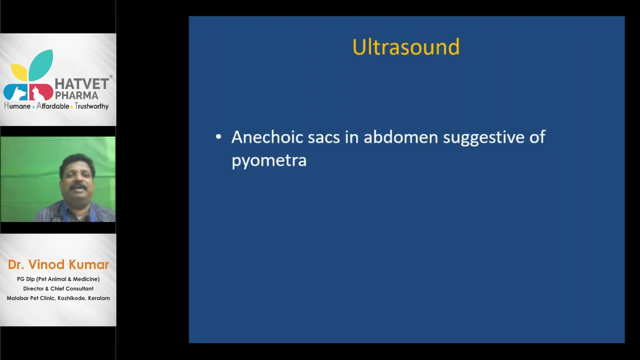 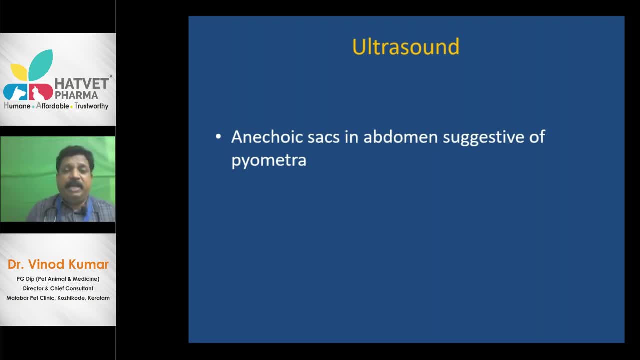 Because the body is tending to eliminate as much as toxins from the body. So in ultrasound anacoid sacs in the abdomen was seen which was suggestive of pyometra. In that condition the quake came there. He gave some injections and went. 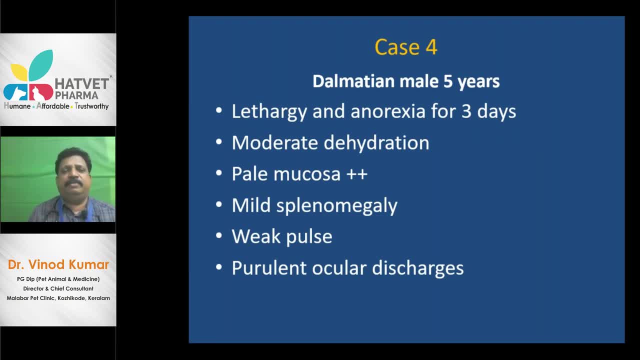 Let us move to the case number 4.. Let us move to the case number 4.. It is again a gentleman, I hope I remember he is from. He is a government servant. He is a government servant, A Dalmatian male 5 years old. 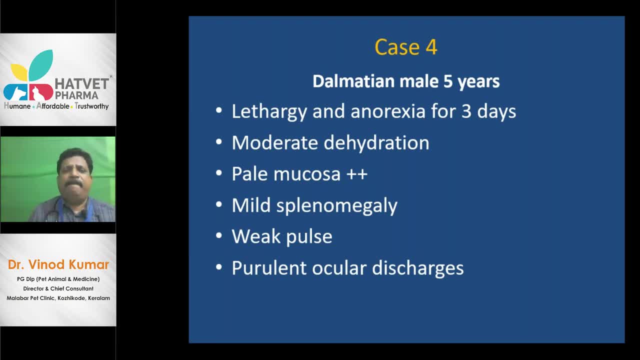 It had lethargy- A Dalmatian male, 5 years old. It had lethargy and anorexia for 3 days and anorexia for 3 days. Lethargy and anorexia for 3 days. 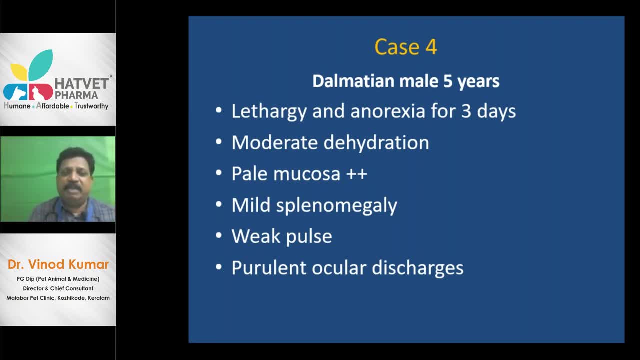 It had moderate dehydration. These are my physical findings On physical examination. Pale mucosa 2+: Ok, good, There is mild splenomegaly. Very good, There is weak pulse. Of course we have so many pulse like Weak pulse. 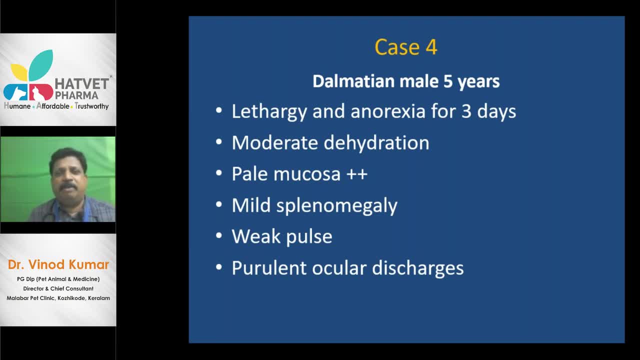 We have strong pulse, We have bounced pulse, We have Wiry pulse, We have thready pulse. So many pulse In that we have a weak pulse here. Since it is anorexic and dyspeptic for 3 days, It has moderate dehydration. 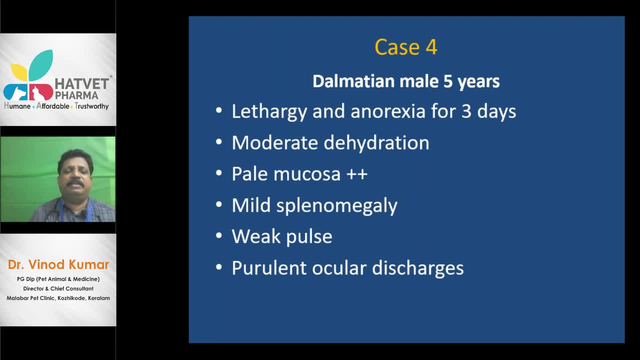 It is definitely it is likely to have a weak pulse like this: Purulent ocular discharges. Why it is having purulent ocular discharges. Why it is having purulent ocular discharges: Oh, maybe it is having canine distemper. 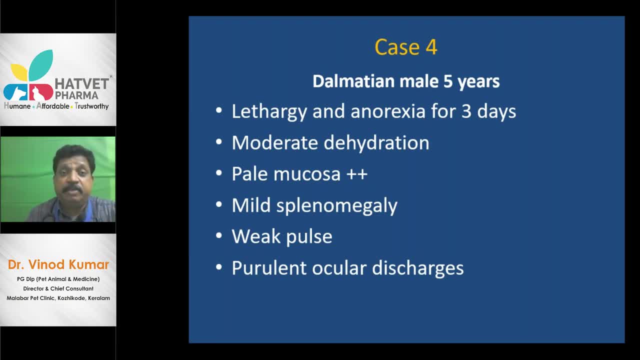 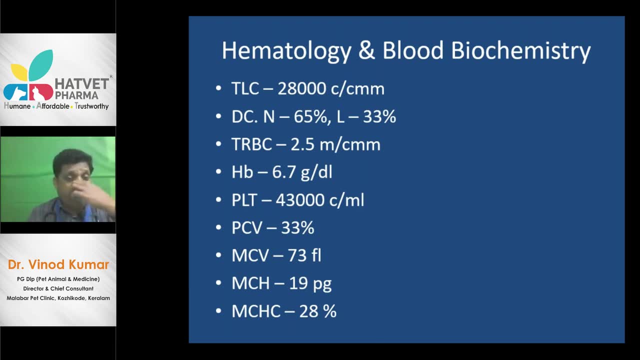 Yes, Let us see whether it is canine distemper. Ok, We took the blood, We went through it. Total leukocytic count is 28000.. Differential count: neutrophils 65%, Lymphocytes 33%, RBC. of course there is anemia: 2.5%. 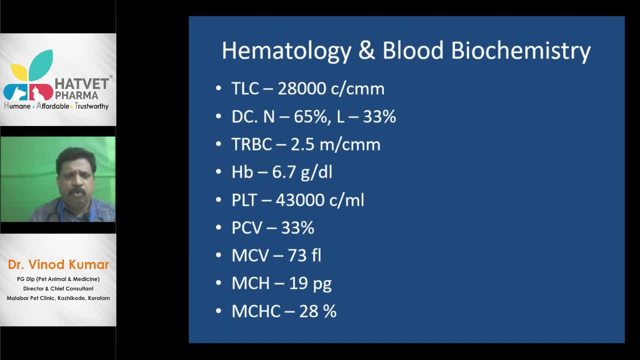 No, in canine distemper. how come anemia? No, no, no, RBC is 6.5 mL per cubic mm. RBC and hemoglobin is only 6.7 g per deciliter. Of course, the Merck veterinary manual always implies us. 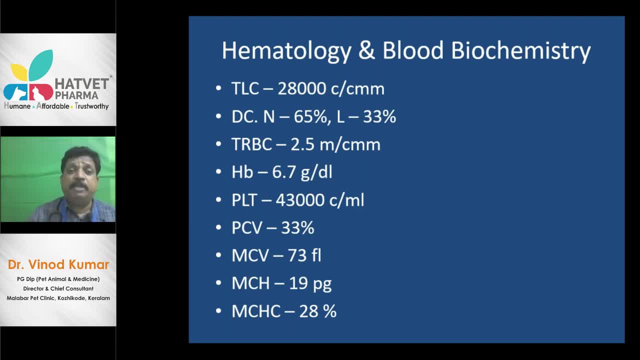 to undertake blood transfusion if the hemoglobin is below 8%. if the hemoglobin is below 8%, PCV is only 33%. PCV is only 33%. It should be 45%. MCV is normal. MCH is very low. 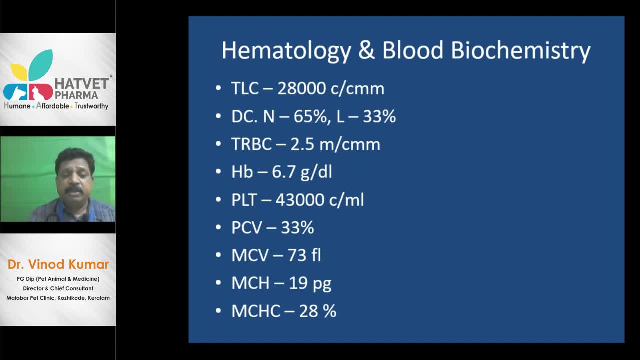 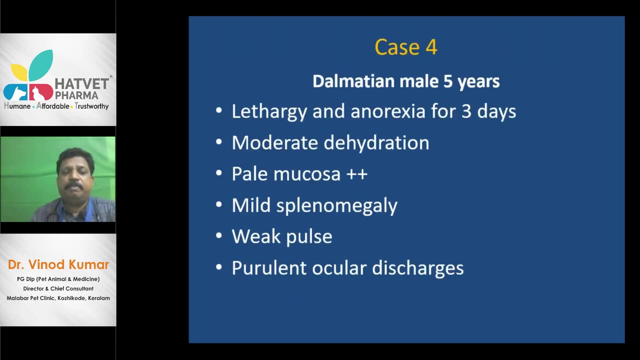 It is only 19 PG, 19 micrograms. MCHC is also slightly low, So what should be it? What is it? I don't know. I don't know what has happened. See, it is a Dalmatian male, 5 years old. I don't know what has happened. 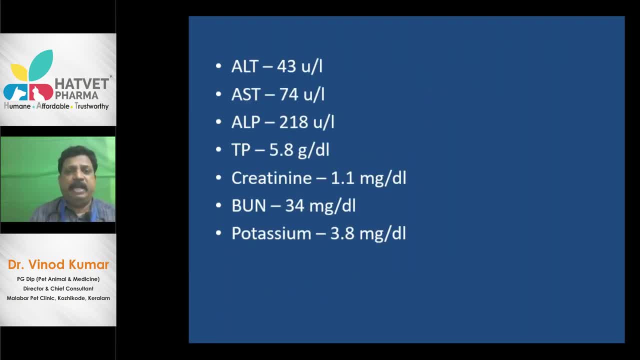 The ALT and the AST level. Okay, it is normal, Leave it. LPL. alkaline phosphatidase is normal. Total protein is normal. Creatrin is normal. Blood urine and ethylene is normal. Potassium is normal. Okay, go Everything. The liver function, kidney function, everything is normal. But what happened? 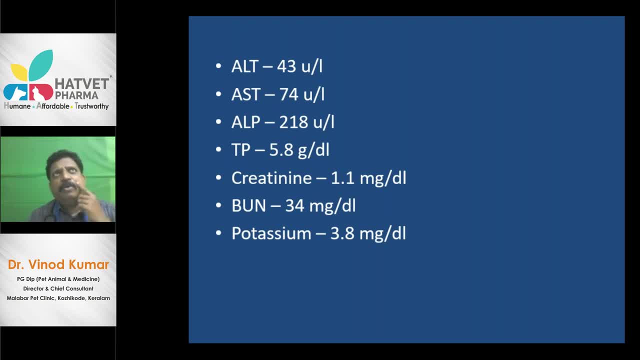 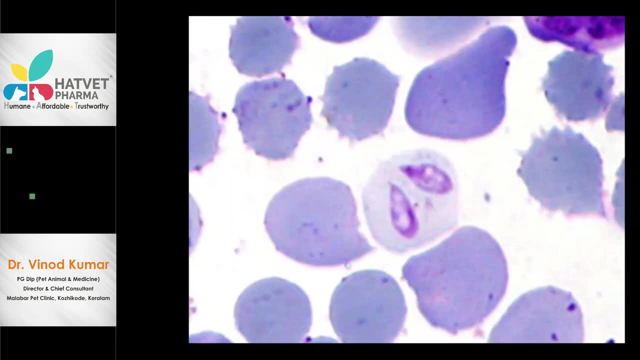 Is it canine distemper? We have only that clue. It is having full endoclonal discharges. So that was submitted for examination. What I saw? I saw this piriform object. See the piriform, This piriform object inside the RBC, Inside the erythrocyte. What is this? 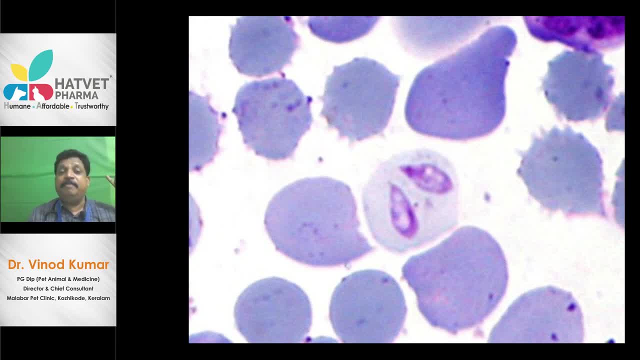 Now you know very well. See, it had a mucosa pale- mucosa 2+, But it did not show any splenomegaly. That was very bad. It had a mucosa pale- mucosa 2+, But it did not show any splenomegaly. That was very bad. 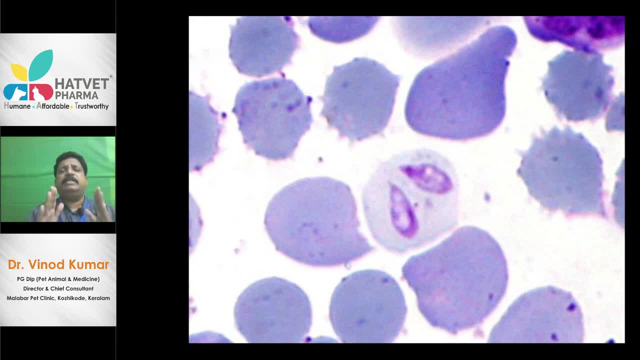 Very important. It did not show in perfectly. So all this from this you should say that splenomegaly is not always consistent. in vector-borne diseases It is not mandatory, But if splenomegaly is not the law for anemia, you can suspect Babesia canis. This is Babesia canis. 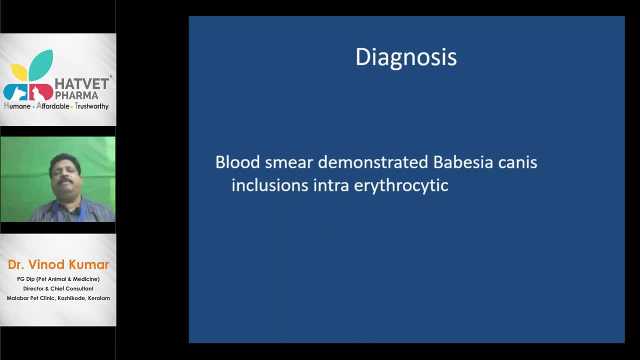 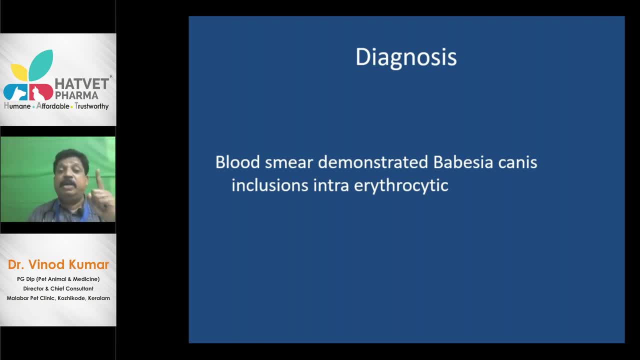 now, in the next session, i am coming with better one diseases, two days class: vector one diseases: it's a very vast class. we'll take it no today. three days, three days class. yes, it is there, it is coming, it's coming. it's a very important class, nobody should miss it. then our next case. 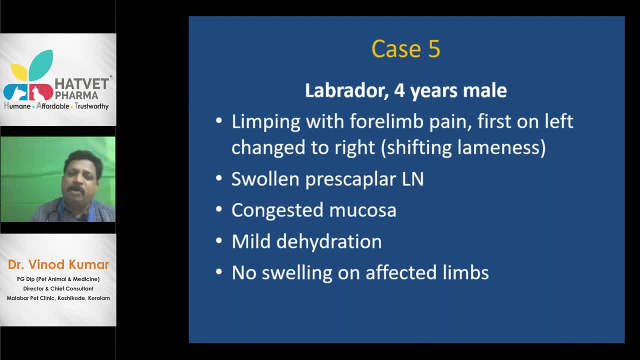 it's again my good client. it's a laboratory four years old male. he is limping the forelimb. it is limping the full limb and he said that the limping was on the left of our limb at the first and now the right forelimb is limping. 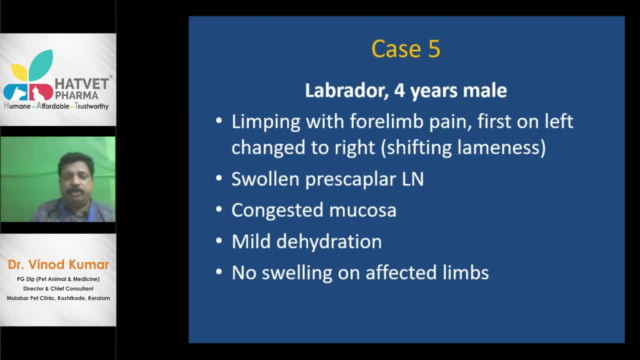 so we say a shifting lameness. of course we see a shifting lameness in the dog and i want to talk about the줄 in a minute, so the could. of course i have met the consideration etc. but today we will say something that i am. i'd like to see something different from the un. استugg tel. 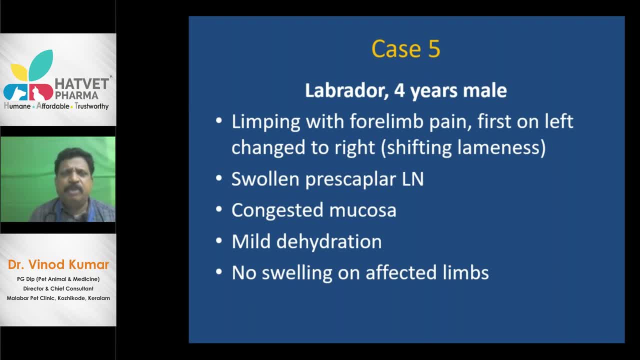 We very well know the shifting lameness in the cow. What is the shifting lameness in the cow? We have the infectious bovine viral rhino. infectious bovine viral rhabdomyolysis. It's a very big disease in the cow. Infectious bovine viral rhabdomyolysis. 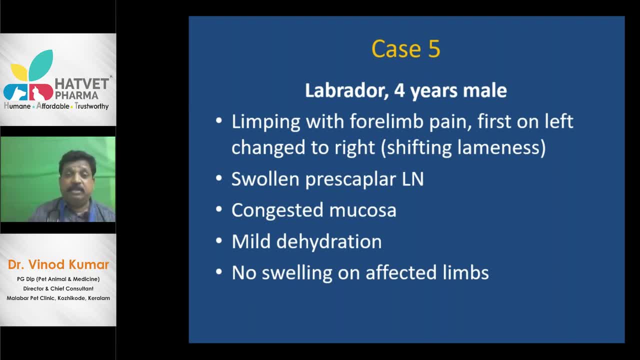 What is that disease, my dear friends? Infectious in the cow. It is infectious. It is infectious, It is not non-infectious. Infectious bovine in the rumen cow, Viral. The etiology is a virus. 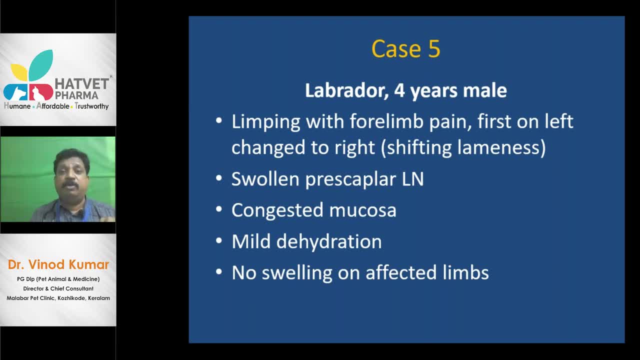 Rhabdomyolysis. What is rhabdomyo and what is leomyo? Rhabdomyo means it is a skeletal muscle. Leomyo means it is a smooth muscle. Rhabdomyolysis: Smooth muscle inflammation. 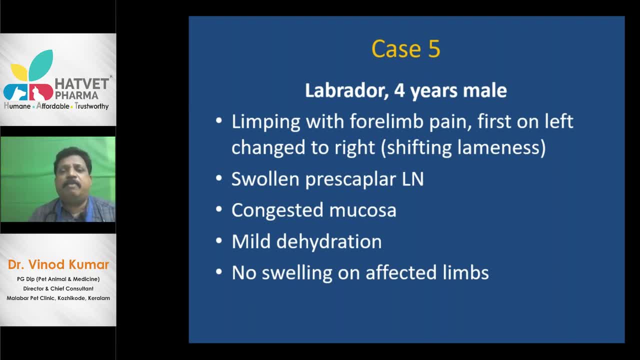 What is the disease? It is nothing but the rhabdomyolysis. Rhabdomyolysis is a three-day fever virus, Or the ephemeral fever. It is a technical term for the ephemeral fever, So the ephemeral fever will produce a typical gait. What is it? 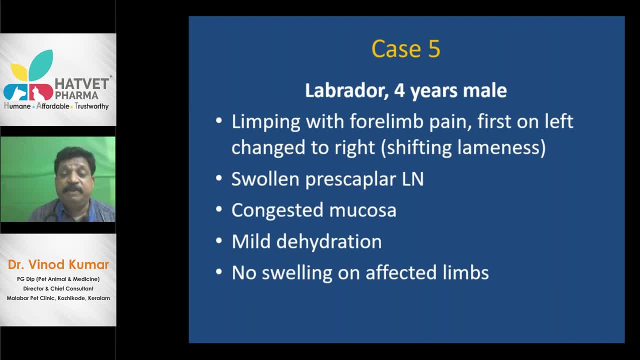 It produces shifting lameness or a three-day fever. So, likewise in a dog, you find it shifting lameness. It could be this disease. What disease? This disease? I don't know what this is. I am seeing only shifting lameness. 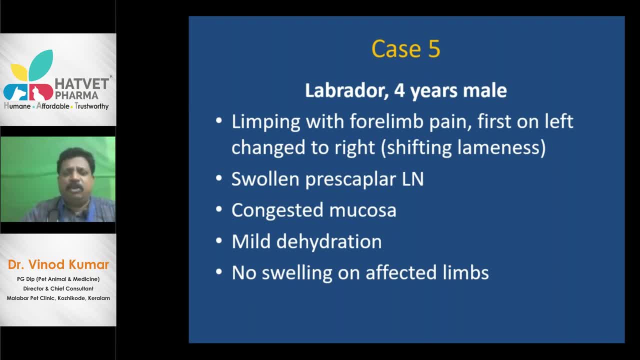 What is it? It could be arthritis, synovial Diseases, Acute synovitis. I don't know. I don't know. You decide, I don't know. There was swollen prescapular lymph nodes. It was a congested mucosa. 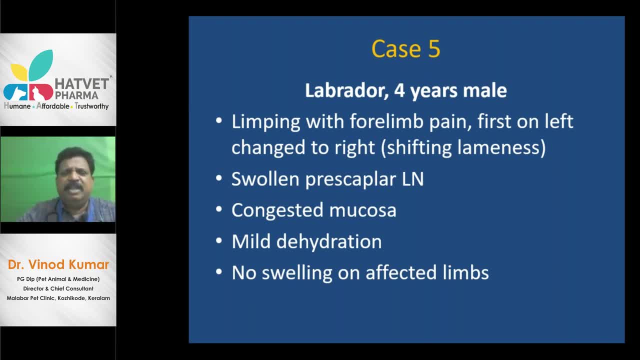 There was a mild dehydration. There was no typical swelling on the affected limb, But it is limping And the client clearly said that it was limping on the left at first. Now it is right What it could be, my dear. 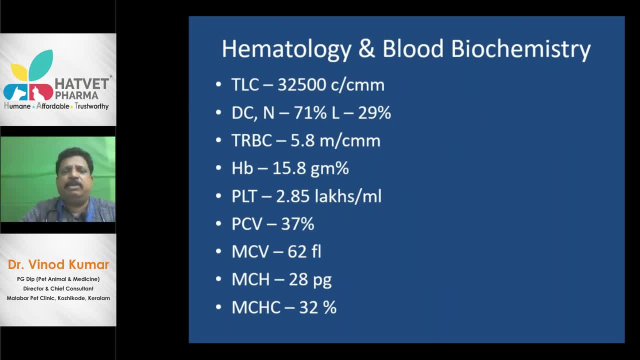 See the total leukocytic count here: 32,500, very high DC, 71% neutrophils. high RBC. normal Hemoglobin normal Platelets normal. PCV normal. MCV normal. 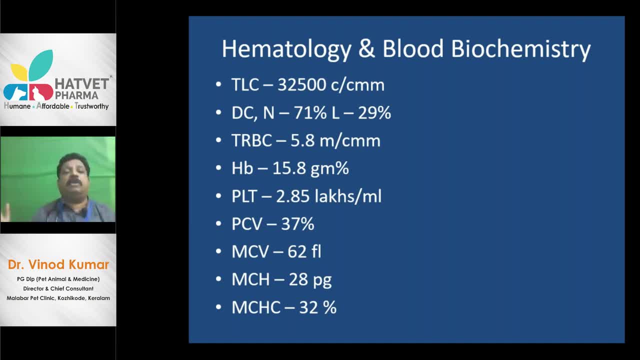 MCH normal, MCHC normal. Everything is normal Except the leukocytosis. What is this? So whenever you get such a case, it is shifting lameness, Mucosa will be congested, There is swollen lymph nodes. 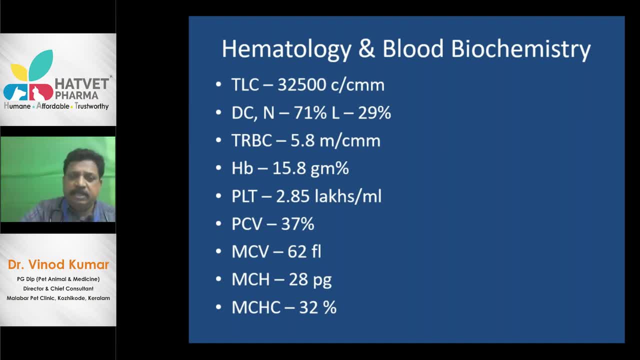 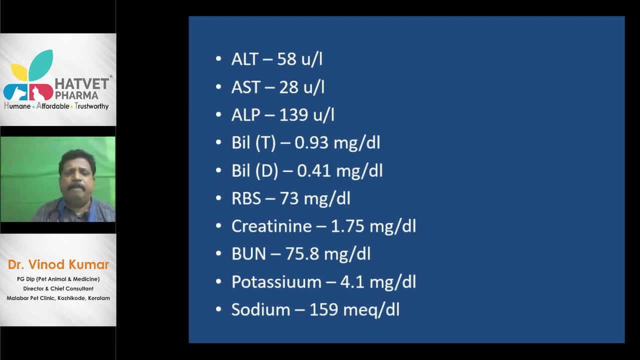 Of course, we are not able to diagnose what it is Such a case? See now we have gone through the ALT AST. Liver is normal. Bilirubin is normal. Random blood sugar is normal. Creatinine is slightly high. 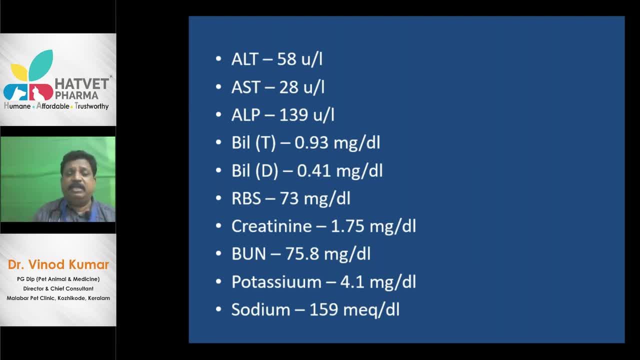 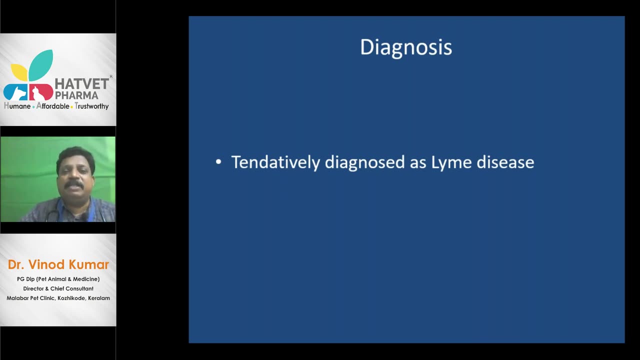 Blood urine nitrate is slightly high. Potassium is normal. Sodium is normal. What happened to this dog? I don't know What happened to him. So the diagnosis It was a tentative diagnosis. It was tentatively a diagnosis. If there is a shifting lameness, we should tentatively 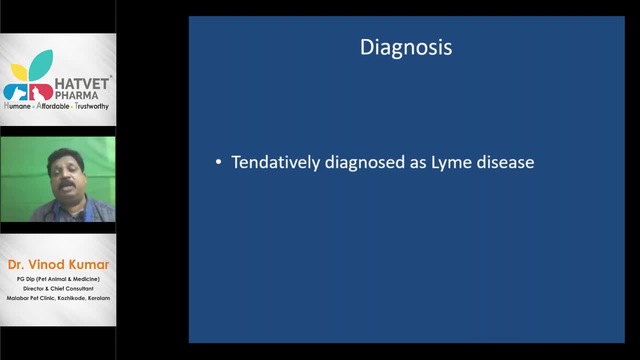 There is no method by which you get conclusive diagnosis. Diagnosis that is really a burgdorferi infection. It is a spirochete. Of course we know the spirochetes. We have different types of spirochetes in the body. 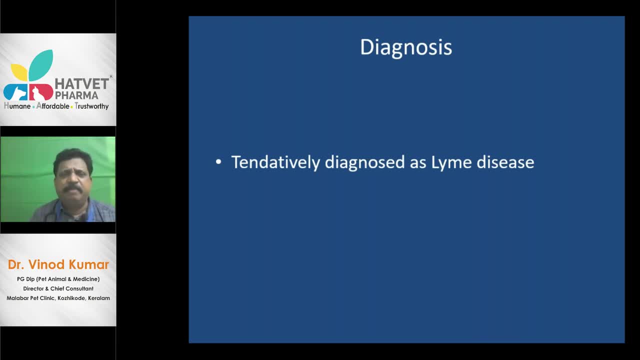 We have human syphilis- Tryponema pallidum. We have rabbit syphilis- Tryponema cuniculi. We have human and animal leptospirosis. Leptospira interrogans: Leptospira biflexa. 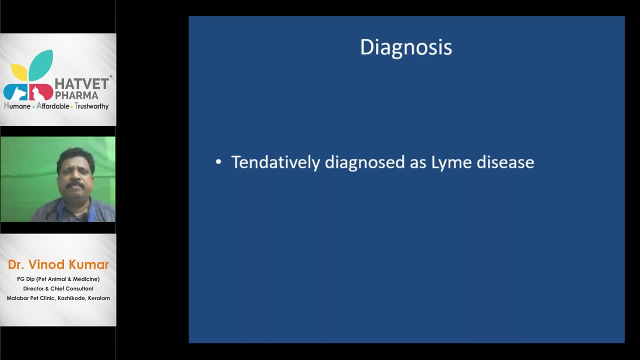 Leptospira pormona, Icterohemorrhagiae Canicola, Osteolysis Autumnalis. All these things are leptospires, All these are spirochetes. This is again the Lyme disease. 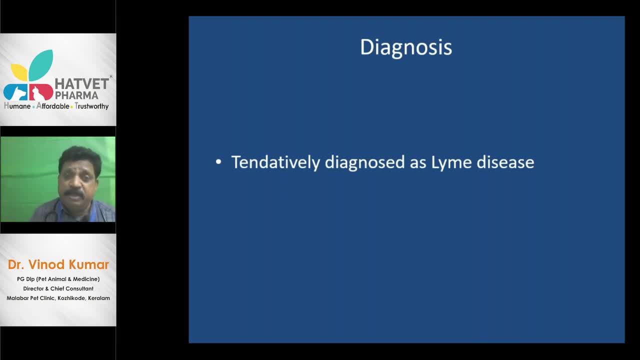 The etiology for Lyme disease is a spirochete. What is it? Borrelia burgdorferi. So it was a tentative diagnosis. I clearly say it was a tentatively diagnosed And I gave benzoyl penicillin for this also. 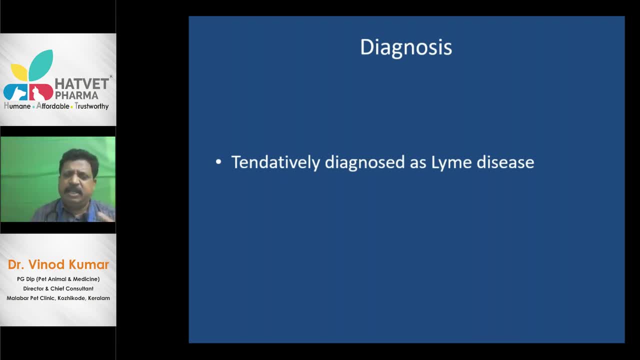 It was completely recovered after 3 days course, Just 3 days course of benzoyl penicillin injection. You know the dose of benzoyl penicillin: It is 20,000 to 50,000 IU per kg. 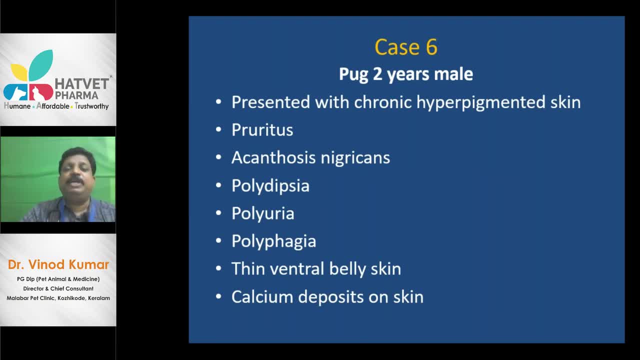 Let us go to the 6th case. It is a 2 years old male. I don't know, I don't remember this client. I don't exactly remember this client For 2 years, male Presented with chronic hyperpigmented skin. 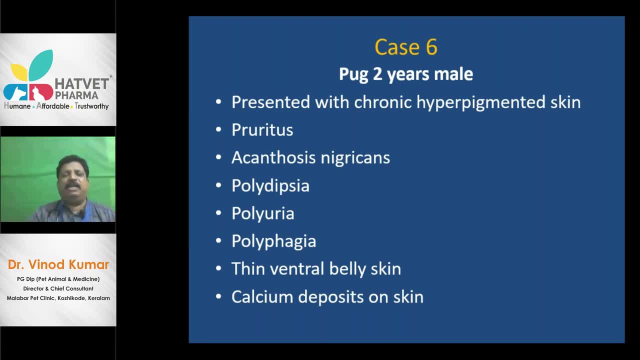 It contains all the clues. All these are my PE findings, My physical examination findings. It has chronic hyperpigmented skin, It has pruritus, It has itching, It has acanthosis nigricans, It has polydipsia. 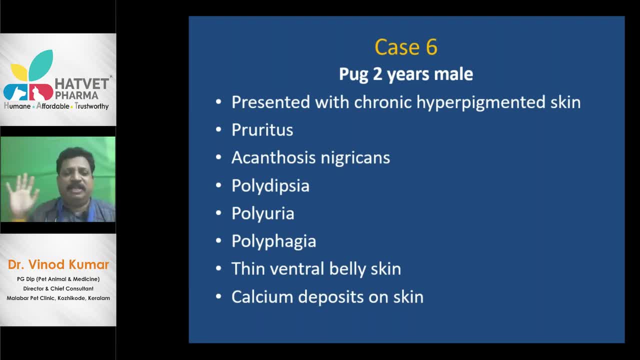 It has polyuria, It has polyphagia, It has very thin ventral belly skin. It has calcium deposits on the skin, Of course. now, my dear doctors, 100% of my doctors- have come to know what the disease is exactly. 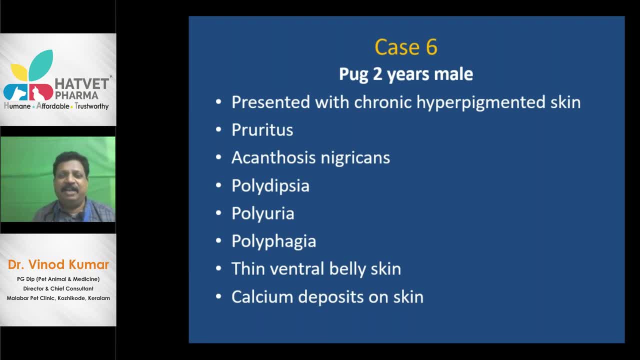 Even my junior doctor, who is sitting on my side, A lady junior doctor sitting here which you cannot see over the camera. She is sitting here, She is smiling and laughing Because she knows what has happened, Because she is listening to all the classes which I am uttering daily. 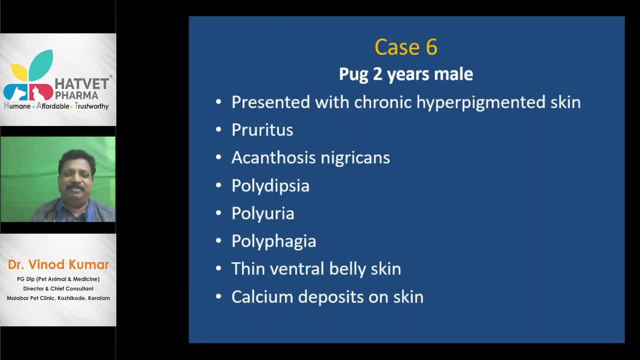 And my clinical cases are also described to her, And now she is shaking the head. Okay, that is good. She also understood. She just completed her degree course And so, And so what it could be, It is a pug, 2 years old male. 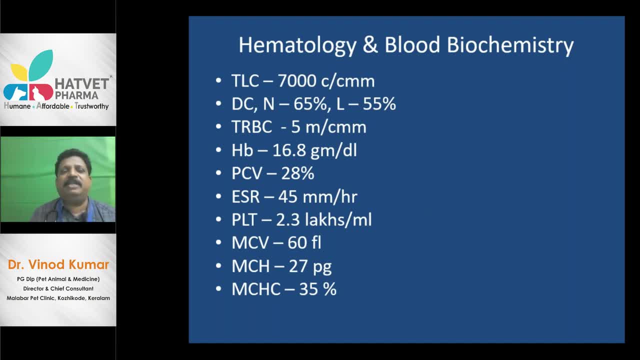 Coming to the hematology and blood biochemistry We have taken, the total leukocytic count is normal. DC normal Everything neutrophil normal Lymphocyte, normal RBC normal Hemoglobin, normal PCV, normal ESR slightly high. 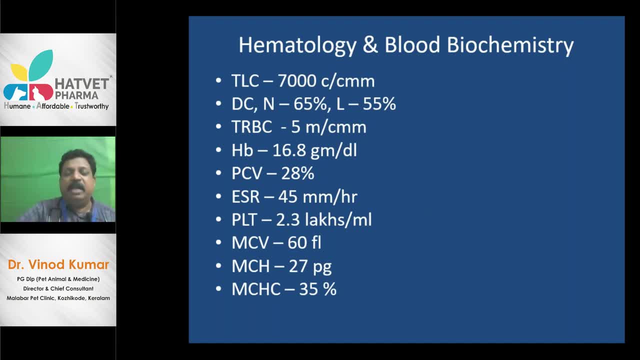 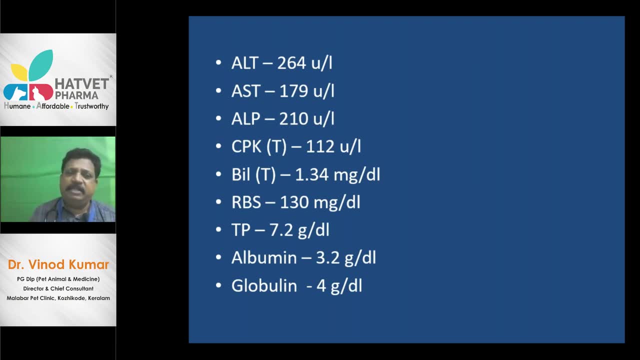 Platelets: normal: MCV, MCH, MCHC, Everything normal. Everything is normal. And T is raised. Yes, Why? ALT only is raised? AST is also raised, ALP is raised, So there is a hepatic impairment. 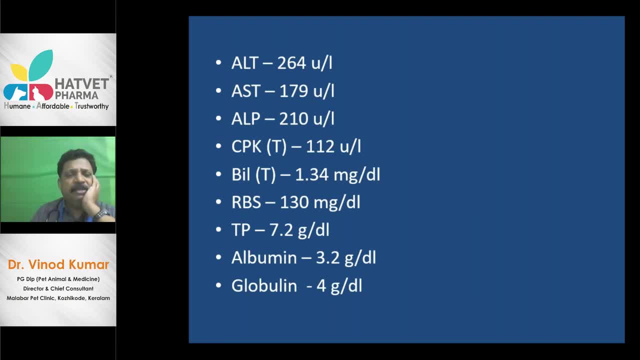 What happened? There is a hepatic impairment, CPK. CPK is normal, Bilirubin total is normal. Random blood sugar is high. It is 130 mg per deciliter is high. So the hepatic dysfunction, Random blood sugar high. 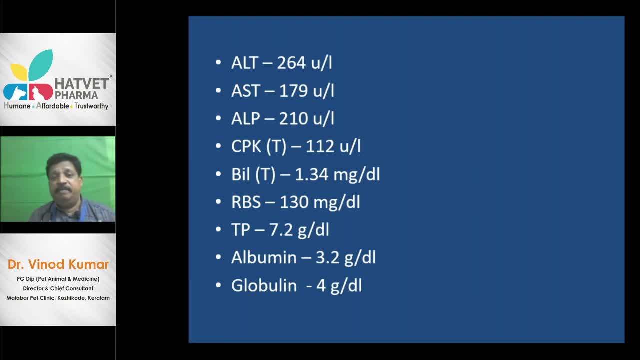 Having calcineosis cavities, Thin skin, Hyperpigmented skin, Polyuria- polydipsia- polydipsia. Polyuria polydipsia- polyphagia. Ok See, now you have come to know what the disease is. 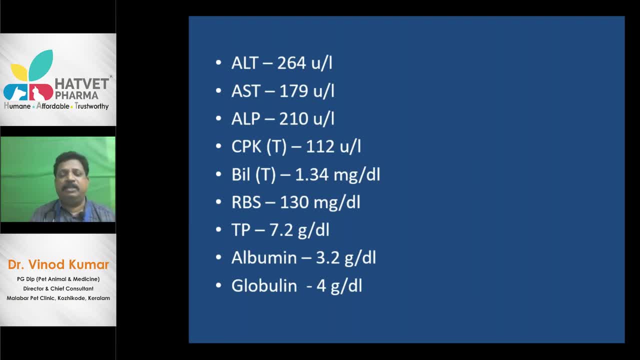 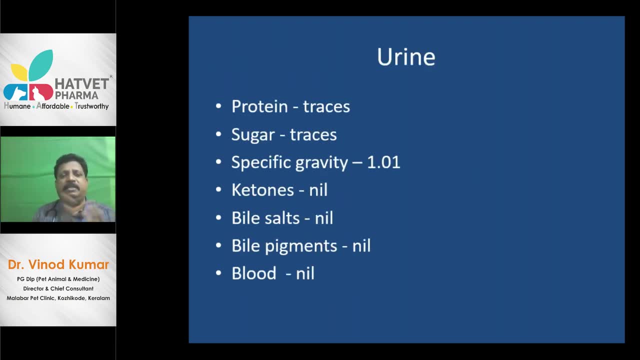 Alkabin is low, Globulin is normal. Of course, what has happened? We went to the urine examination. We collected the urine, Protein traces, Sugar traces. Specific gravity is 1.01.. Of course, See, I told that 1.015 to 1.032.. 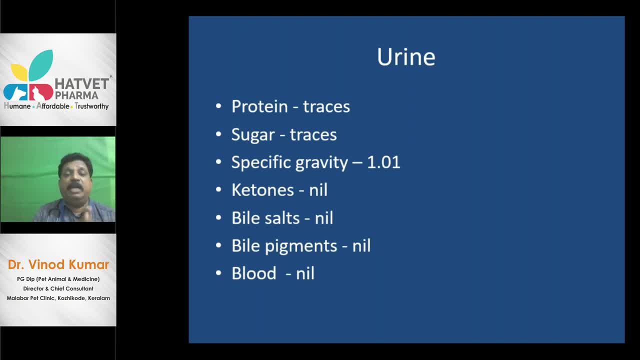 Is the normal specific gravity of urine. Anything below 1.015 is said to be hyposthenuric urine Or hyposthenuria. Ok, So there is hyposthenuria Due to increased quantum of urine. There is hyposthenuria. 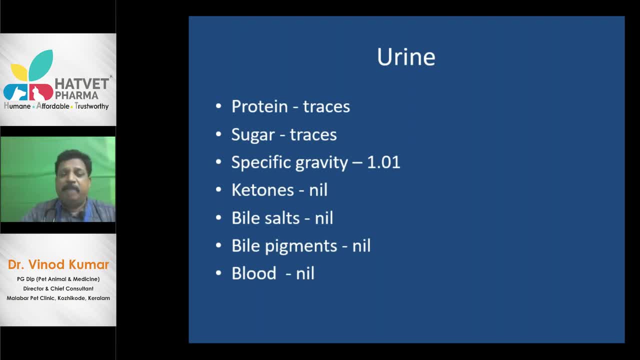 And ketones, nil Bile salts, nil Bile pigments, nil Blood nil. So The only point in urine is hyposthenuria. Now we have diagnosed. I know that You are all very intelligent people. You diagnose it very well. 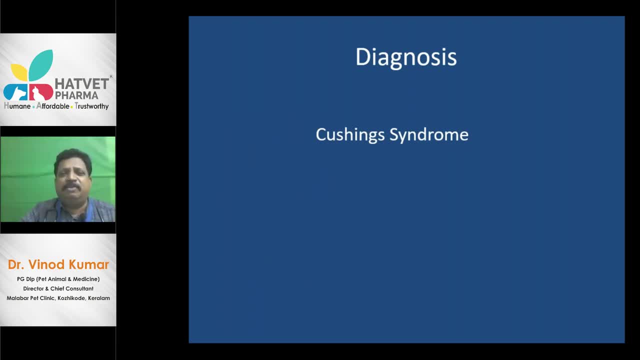 So it is so easy, Very easy to diagnose. it was Cushing's syndrome. It was Cushing's syndrome. Then let us come to the last case. This case also is very important for me Because One of my girl friends- She presented this animal. 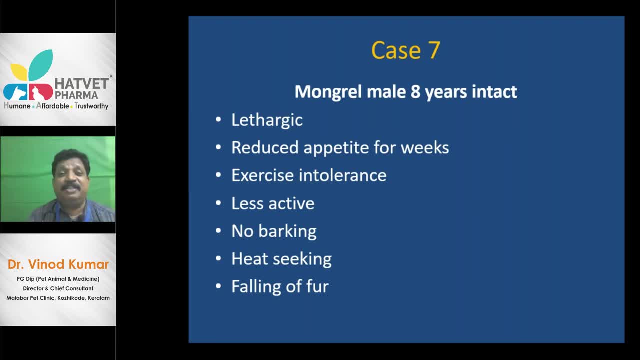 She is a lady client. My wife should not hear this. She will make a hell of problem after this, So I should be very much cautious While telling that this is my girl friend. So this is case number 7.. Our last case. 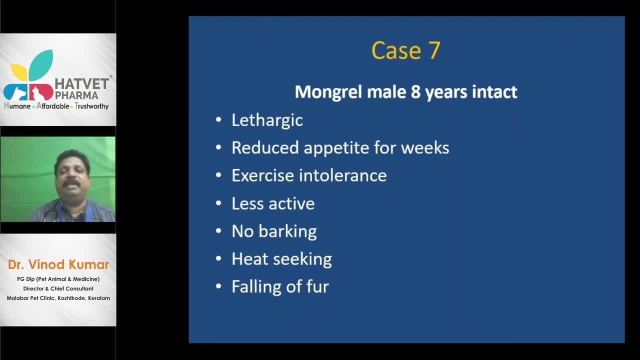 It is a mongrel Male, 8 years male. It is intact. It was lethargic. See now again You can go through the clinical science itself. My findings: It was lethargic, Reduced appetite for weeks together. 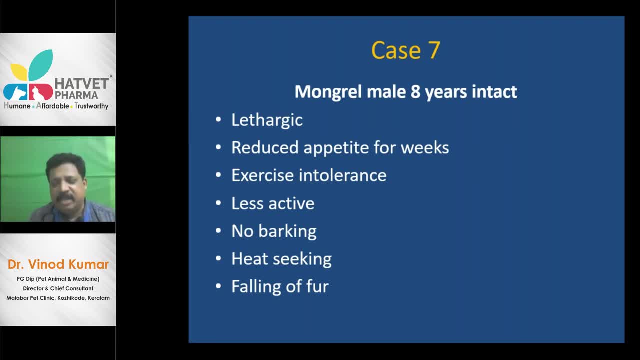 With exercise intolerance, Always lethargic. And having exercise intolerance It is less active. No barking at all. It is hesitant to bark. Sometimes it may bark. That will be the bark. like this: It is hesitant to bark, It is heat seeking. 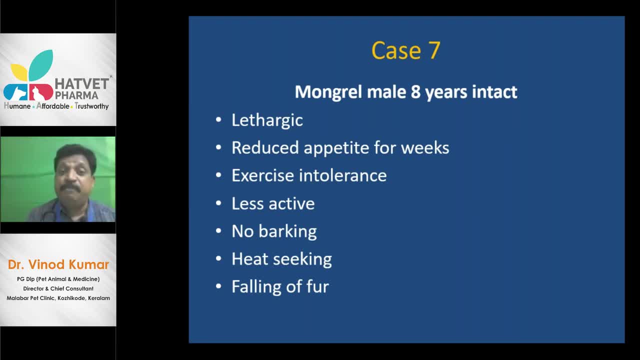 He told that Whenever it is let free, It will go to the sunshine And sleep there. Well, A heat seeking dog. There is falling of fur. There is no falling of hair in the dog, It is only falling of fur. 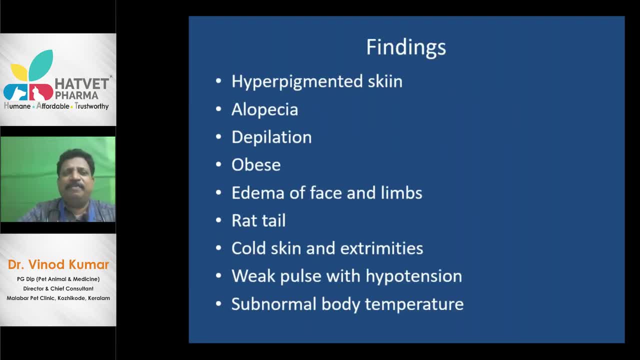 Okay, So These were my findings: Hyper pigmented skin, Hypophasia, Depilation, Obesity, Edema of the face and limbs, Rat tail, Cold skin at extremities With hypertension, Subnormal body temperature. So, my dear doctors, 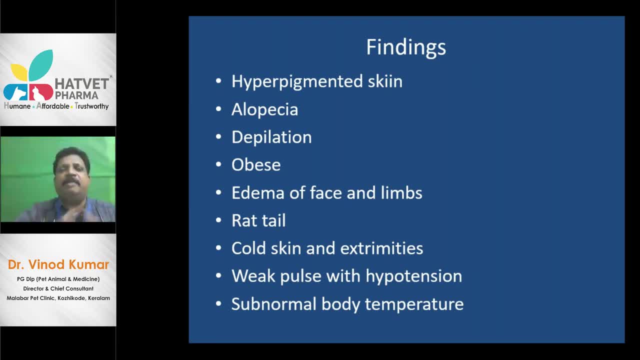 I know that you all are excellent in diagnosis. You are all brilliant people. You have diagnosed this So simple. it is Now Unremarkably. We are taking the Hepatological blood vacuosity factors. Total leukocytic count. 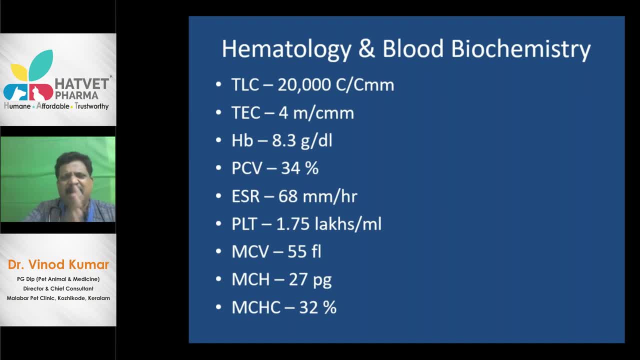 Of course We can say About 17000 is abnormal, But now Only 20000 is normal. We can say Erythrocytic count is just 4.. It is coming to the lower side. It is having slight anemia. 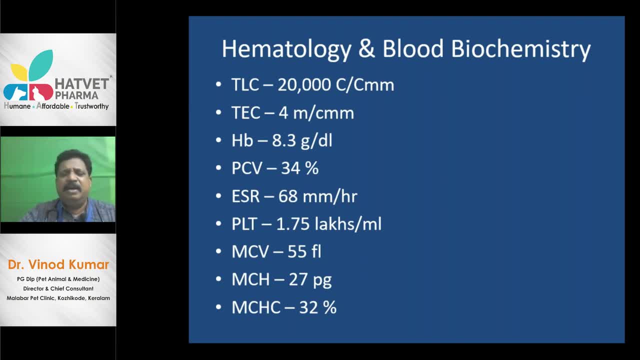 Hemoglobin is low, PCV is low, ESR is high, Platelet is normal, MCV normal, MCH normal, MCHC- normal MCHC normal. There is no hemorrhage, There is no ion deficiency, But there is. 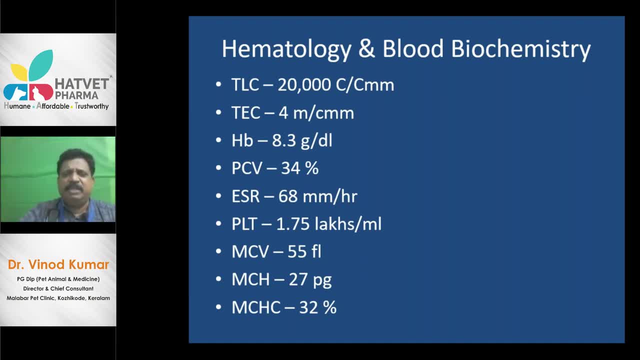 Slight anemia. LT is high. LHT is normal Or high LLP is normal. Bilirubin is normal. Bilirubin direct is normal. RBS is low. Random blood sugar is low. Cholesterol is high. 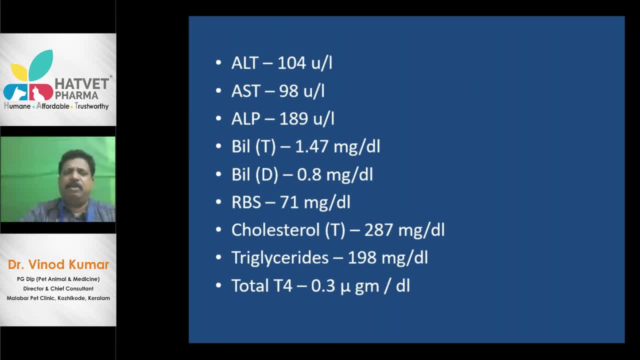 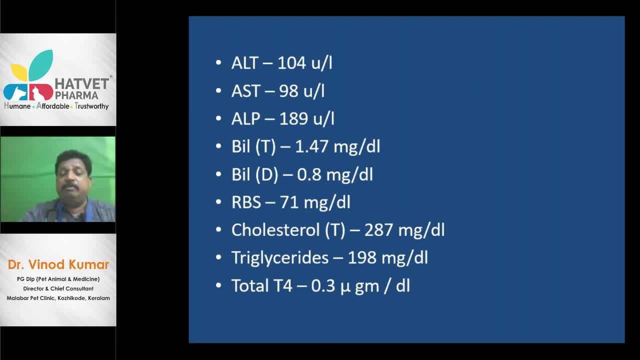 Desireably it should be 240 mg per dl. Here it is Almost coming to 290 mg per dl. Triglyceride is high. Then I took the total T4.. Now you have got it. See Total T4.. 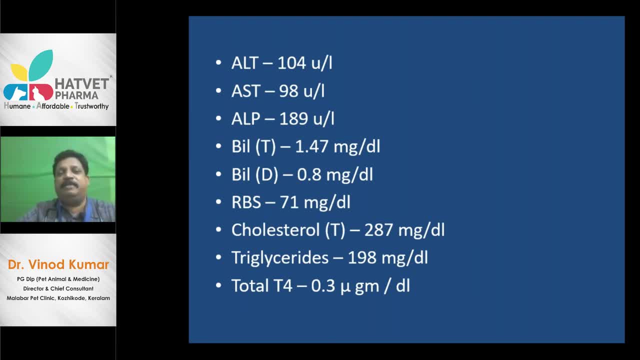 Why I take total T4? I should not have told this Total T4. I should have hidden this, Then only shown to you Total T4 was only 0.3 microgram per deciliter. I said that in my dermatology class itself. If the total T4 is normal, it should be between 1.5 micrograms to 3.5 micrograms. 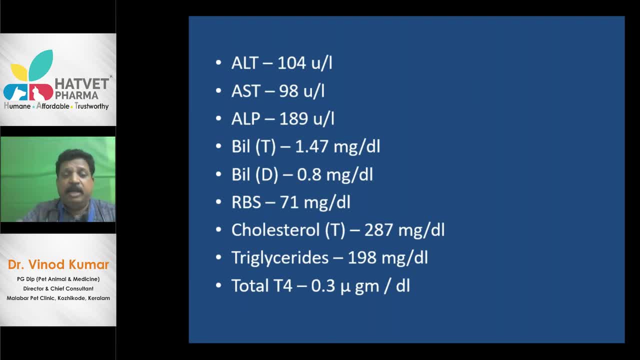 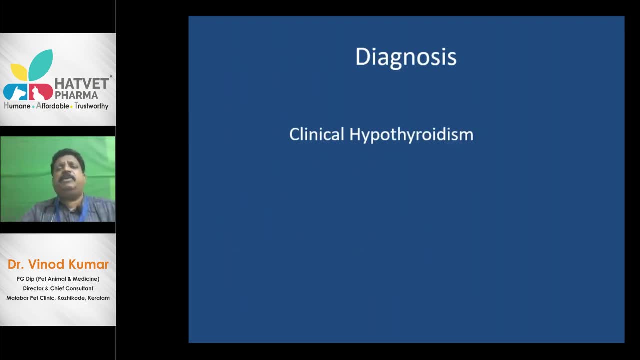 So anything below 1.5 is abnormal. It is only 0.3 micrograms per deciliter. See how slow it is. Invariably, It is very easy to diagnose that it was clinical hypothyroidism. It is very easy. And this case is that is still alive, That dog is still alive.